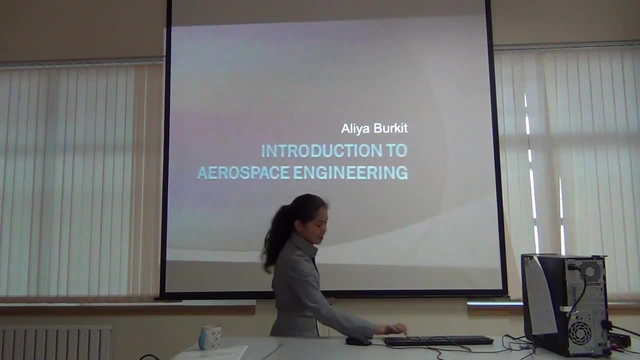 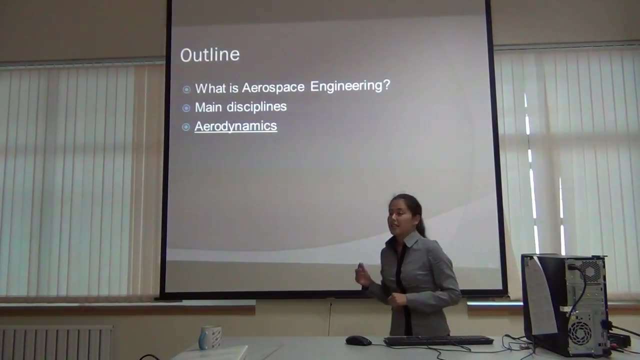 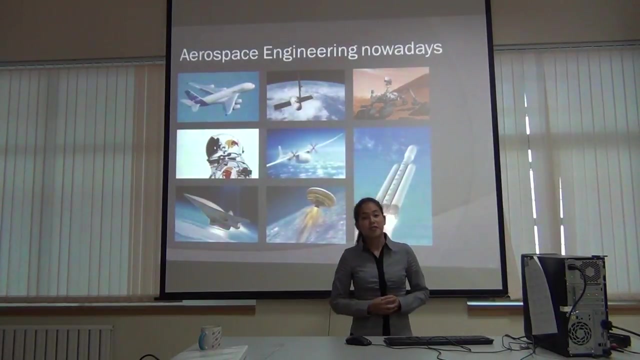 Okay, let's see our agenda for today. Today I will talk about what Aerospace Engineering is, what it consists of, and for the rest of the class, we will focus on Aerodynamics, which is one of the main disciplines of Aerospace Engineering. So what is Aerospace Engineering? It is a branch of engineering that deals with design, development, building and testing of aircraft and spacecraft. 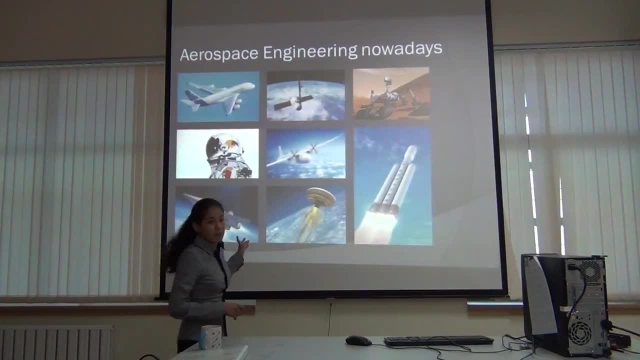 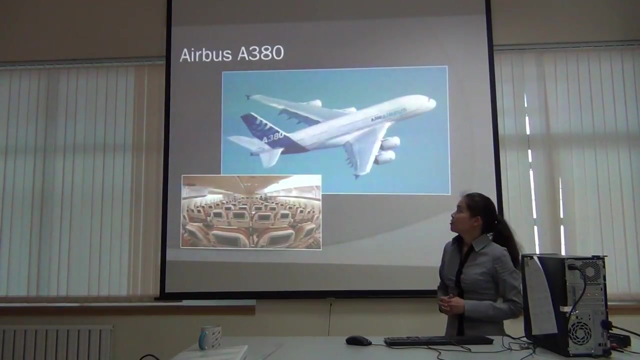 Here I highlighted just a few of the projects that are going on today in Aerospace Engineering, and I will talk about them a little bit more so that you could have an idea of what Aerospace Engineering is. Let's start with Airbus A380.. This is the largest passenger aircraft ever built. It can carry about more than 500 people at a time. 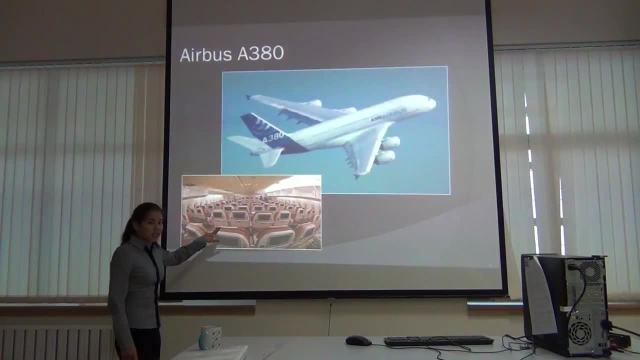 This is the largest passenger aircraft ever built. It can carry about more than 500 people at a time And you can see the seating configuration here, so it fits 10 people in a row. and also it is a double deck, so you can imagine how many people can fly in one flight. 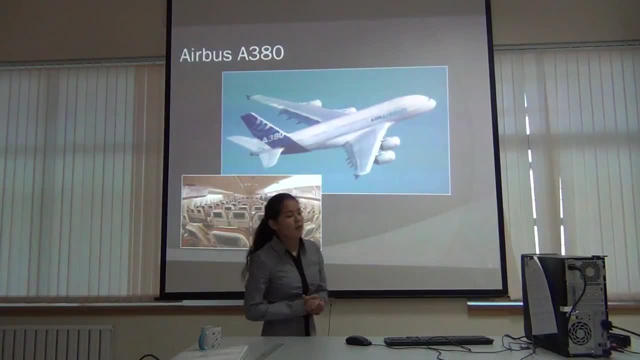 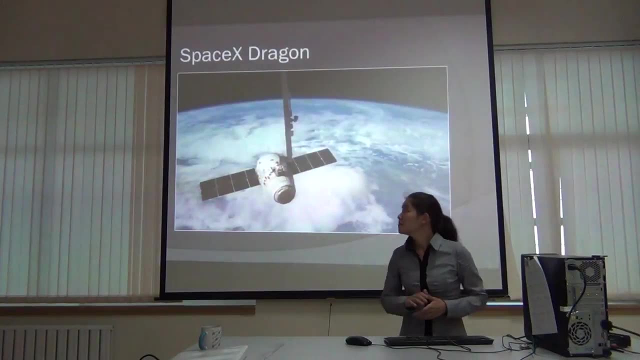 It weighs around 600 tons, so you would wonder how this heavy machine can go up in the air. The answer is Aerospace Engineering. Next is SpaceX Dragon capsule. This is remarkable because it is the first private spacecraft to dock the International Space Station. 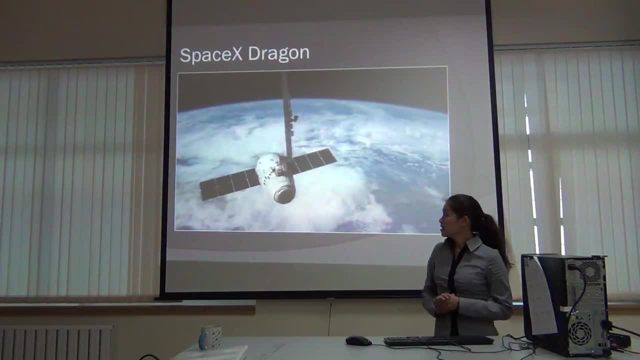 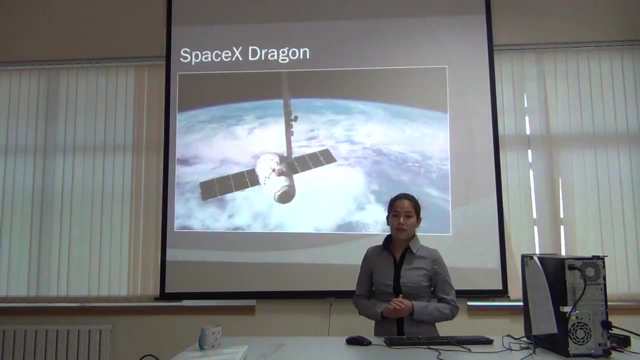 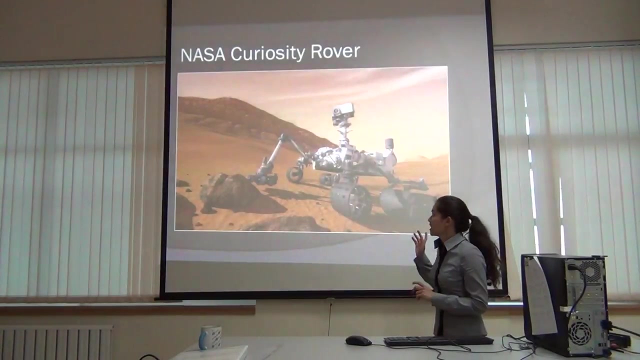 It delivered the necessary supplies to astronauts, but SpaceX is working on the next model of Dragon that will be able to deliver people to the International Space Station. And you've probably heard about this one in the news. It is Curiosity Mars rover from NASA. 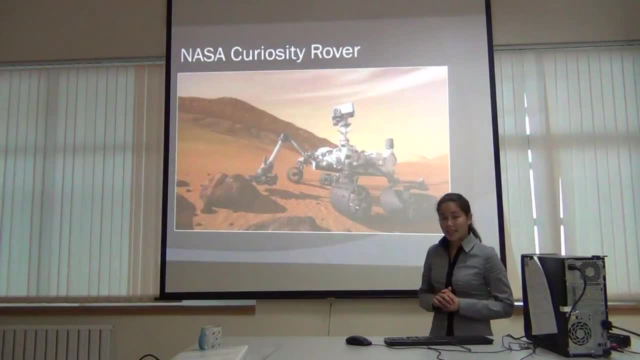 And it is a Mars science laboratory that will investigate the surface of Mars and find out if it is possible to support microbial life there. So you would question how this car-sized object was delivered millions of miles away and there was a 7-minute communication delay, but it was still possible and it is there on Mars. 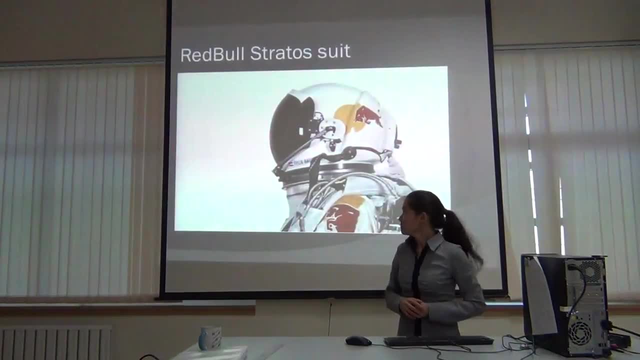 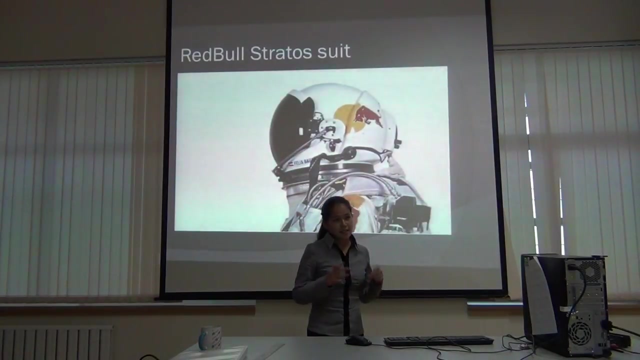 And the answer is Aerospace Engineering. Also, you've probably heard about this guy, Felix Baumgartner, who jumped from 24 miles above the Earth's surface. He was the first person to achieve supersonic speed, that is, the speed higher than the speed of sound. 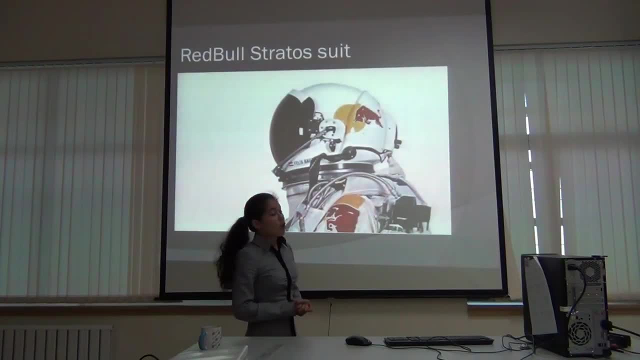 And he was not in a vehicle at that moment. So he broke a world record and achieved a speed of 840 miles per hour. What made it possible for him is his pressure rates Pressurized suit from David Clark Company, which keen years in designing protective equipment for pilots and astronauts. 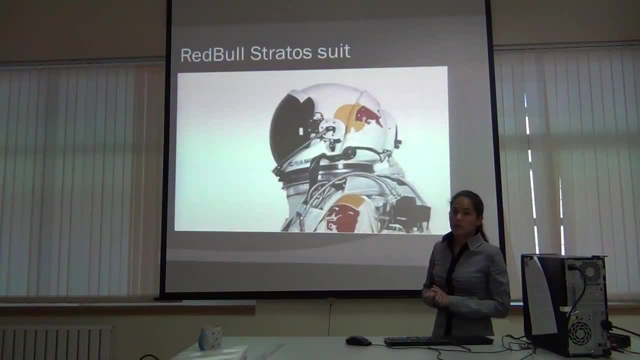 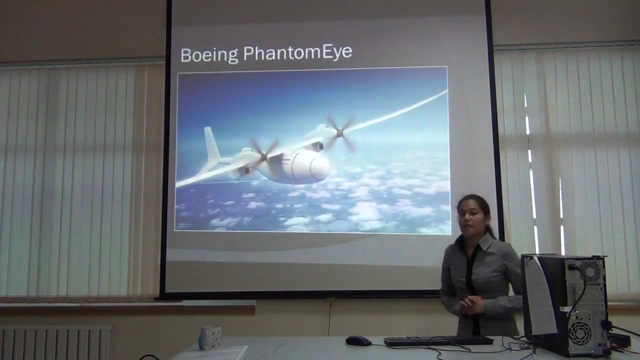 So one of the world records was broken because of Aerospace Engineering. Next is Boeing Phantom Eye. It is a reconnaissance drone, And drone means that it does not have a pilot inside. It can fly autonomously or it is controlled from ground station. And Phantom Eye is remarkable because it runs on liquid hydrogen instead of conventional fuel. 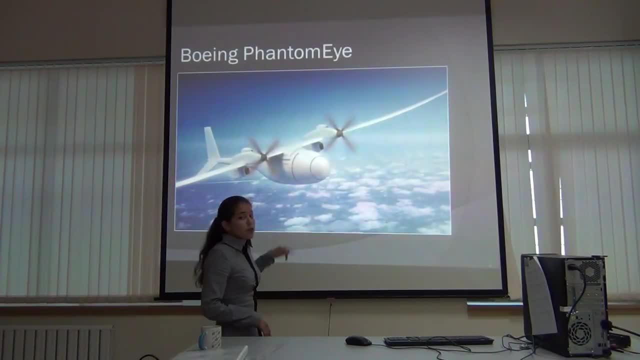 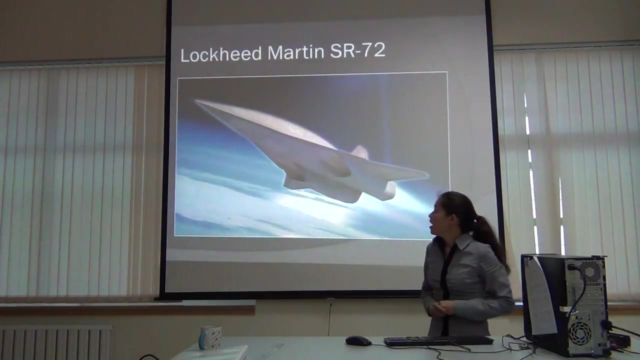 Liquid hydrogen is more efficient than ordinary fuel, So this aircraft can stay up in the air for four days without refueling, which makes it a pretty good deal for the defense industry That can make surveillance for more time now. Next one is Lockheed Martin SR-72 aircraft. 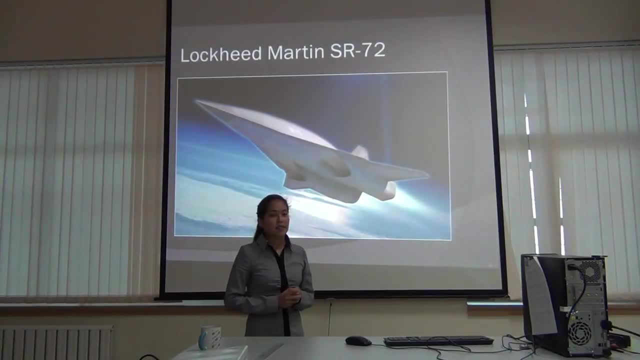 It is in development currently, But Lockheed Martin claims that when it is ready, this aircraft will be able to achieve speed that is six times higher than the speed of sound. And in order to do that, the engines should be modified, Should be redesigned completely. 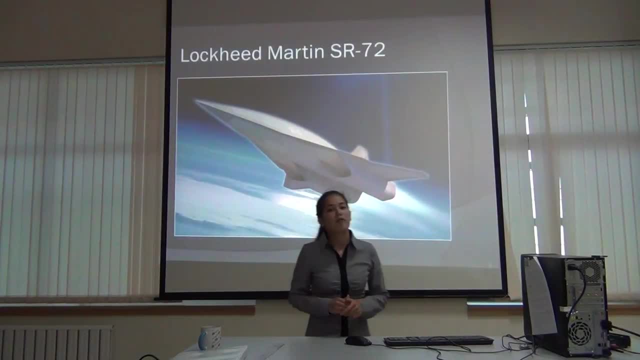 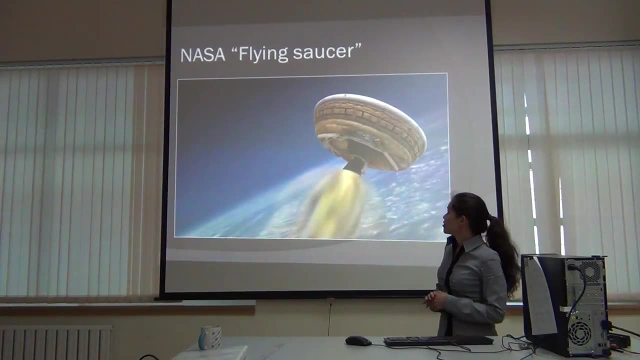 Because conventional turbo jets are not capable of achieving those speeds. And here you can see NASA's flying saucer spacecraft. It really looks like a flying saucer And it is actually ready for its first flight, But weather conditions were not optimal, So the first flight test was delayed. 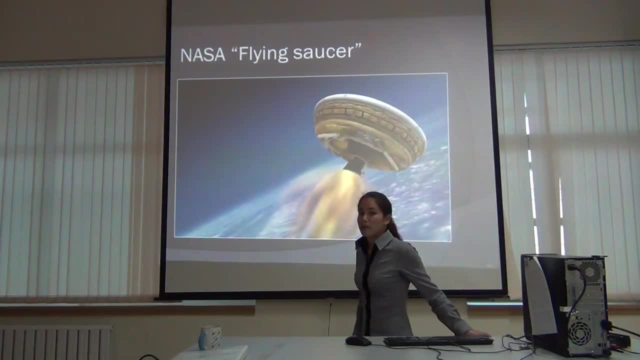 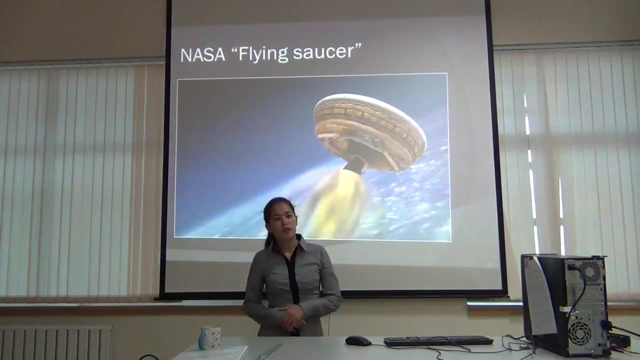 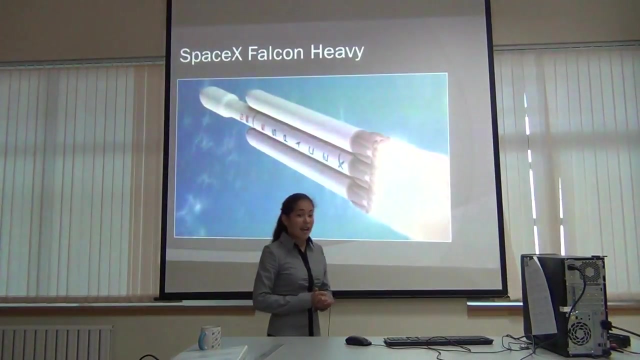 But this spacecraft is designed for flying. It is designed to test heavy payload landing on Mars. And why do we need heavy payload? Because NASA hopes to put humans on Mars, And human habitation model weighs a lot. And the final project that I want to highlight today is SpaceX Falcon Heavy rocket. It is also in development currently, But when it is ready, it will be the most powerful rocket That was ever built after Saturn V. That was used to deliver people on Moon, But SpaceX's goal is even more challenging: To put people on Mars. 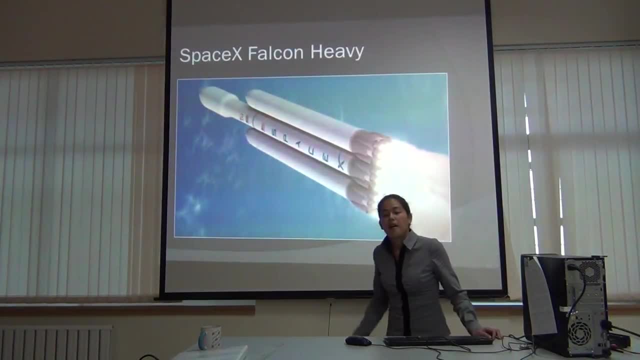 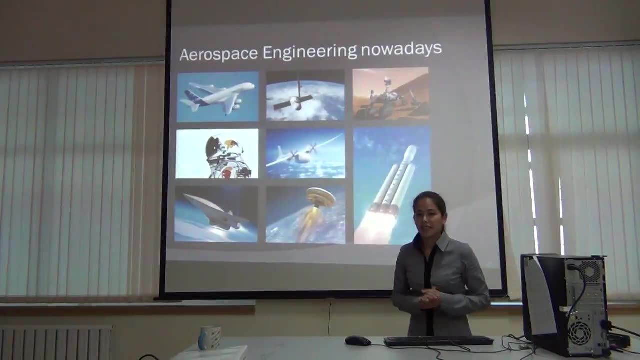 So Falcon Heavy will be one step on achieving that goal. So I've covered just a small part of aerospace engineering, But you can see that it pushes the boundaries of impossible further and further every day. And if you decide to pursue aerospace engineering, hopefully one day you'll take part of a project like this. 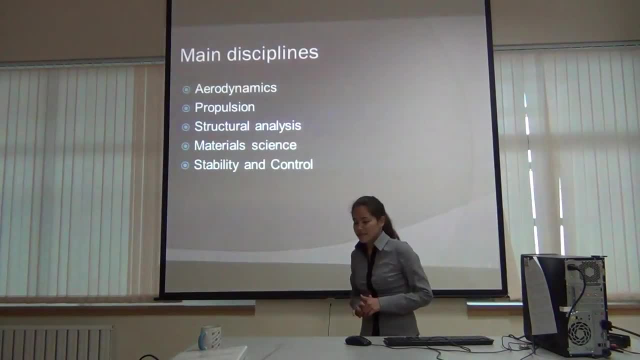 Aerospace engineering is divided into several disciplines. You cannot call yourself just an aerospace engineer. You need to have expertise in one of the fields below, But also you need to know other fields so that you can communicate with other people in your team. So some of the main disciplines of aerospace engineering are aerodynamics, which studies the motion of objects in the air. 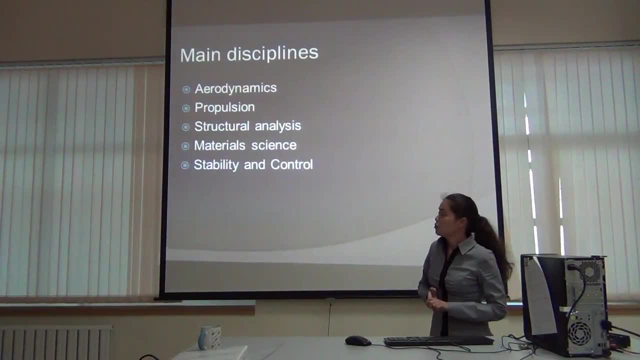 Propulsion, which is how you choose the engine and the fuel that you want to use to push your vehicles forward. Structural analysis is how you build something that is capable of achieving the goals of the mission And that can meet the requirements on the loads that will be put on aircraft or spacecraft. 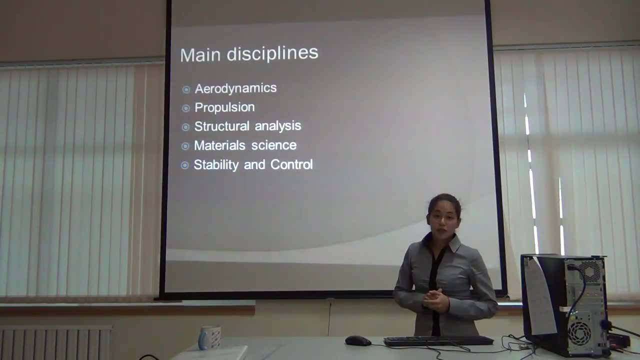 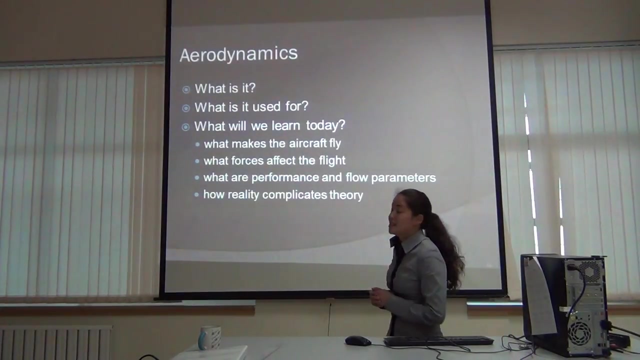 Material science is which materials you choose so that your mission can be accomplished. And stability and control. This is how you control your aircraft or spacecraft and make it go where it needs to go, And today we will focus on aerodynamics. We will talk about what is it and where it is used. 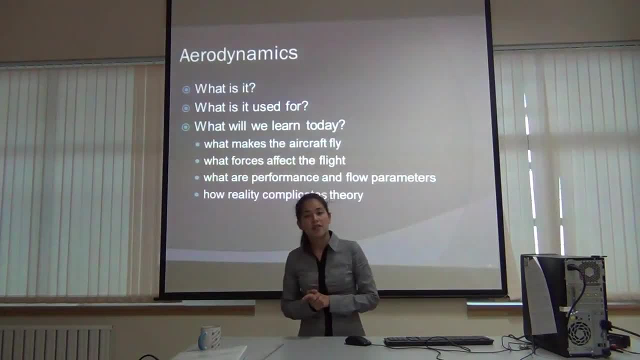 And also we will learn basic principles of aerodynamics, Such as what makes the airplanes fly and what forces affect the flight, What are some of the basic performance and flow parameters, And also how. in real life, things are more difficult than described in theory. 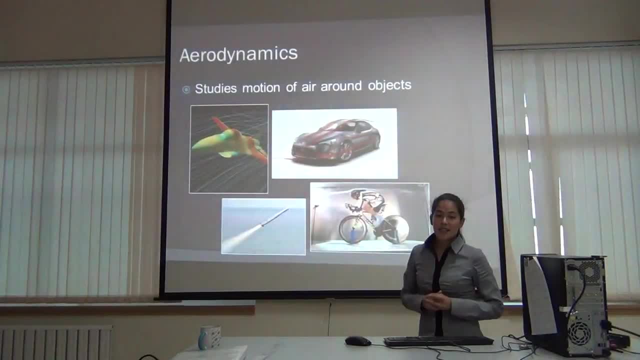 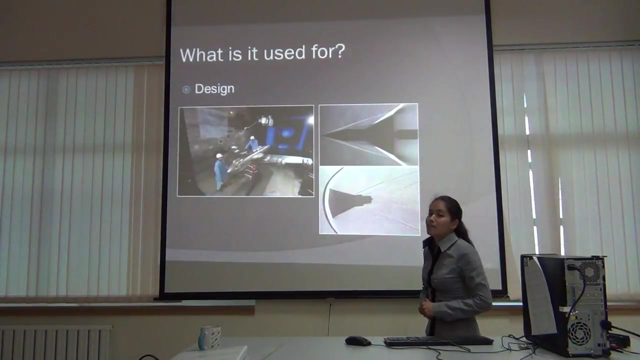 So let's start Aerodynamics studies: motion of air around moving objects. Aerodynamics is applied not only in aerospace industry, but also in automobile industry and even sports. Aerodynamics is mainly used for design of better performing aircraft and spacecraft, And in other industries as well. 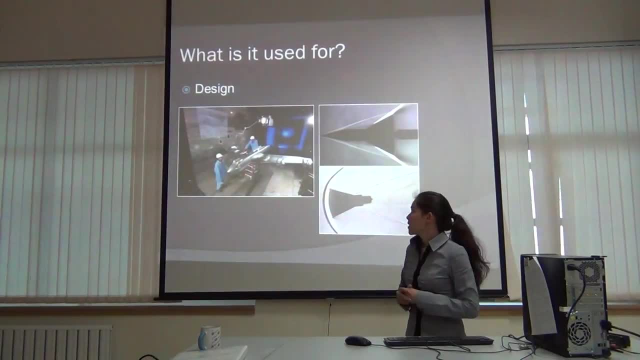 But today we will focus on aircraft. So, for example, Using aerodynamics, These engineers can test a model of aircraft in the wind tunnel, And later they can modify this model so that it will become the optimal. one Another example is how you make better design decisions for spacecraft. 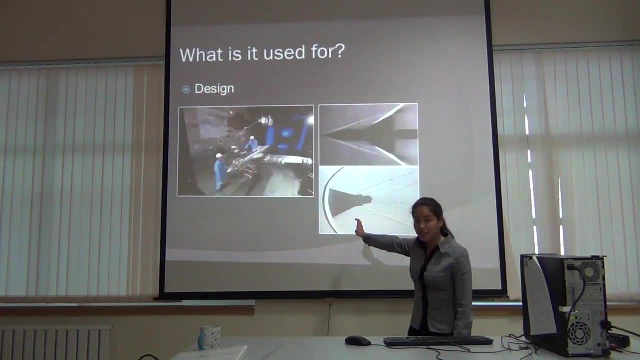 So why the reentry vehicle is blood shaped and not sharp pointed? You would logically conclude that sharp pointed objects have less drag, But aerodynamics can explain this. So if you pursue aerospace engineering, you will learn a lot more about this later, But for now, just believe me. 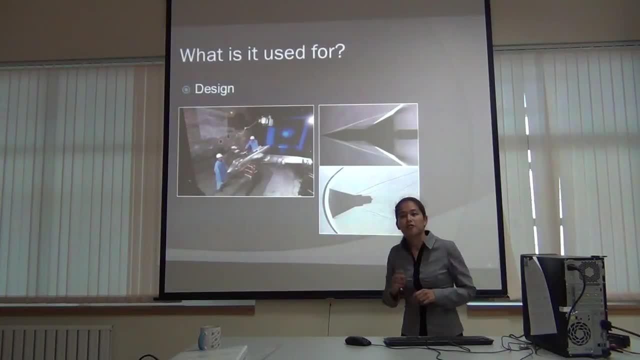 So when objects travel with speeds of greater than speed of sound, Their shock waves occur. So in the first example You see that the object is sharp pointed And the shock wave is attached to it. That makes this shock wave weaker than the other shock wave that occurred here. 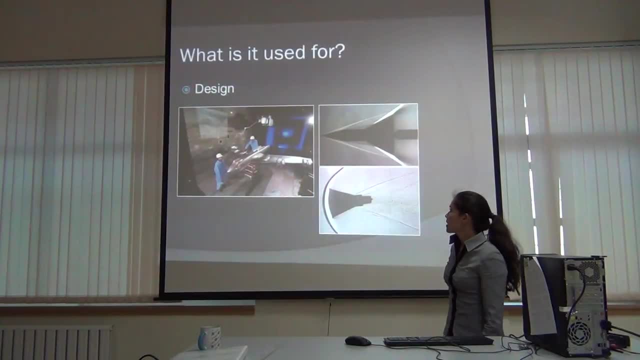 With the blunt shaped body. So in the first case The temperature behind the shock wave That is here Will be lower than the temperature behind this shock wave. That means the object in the first case Will heat up more than the object in the second case. 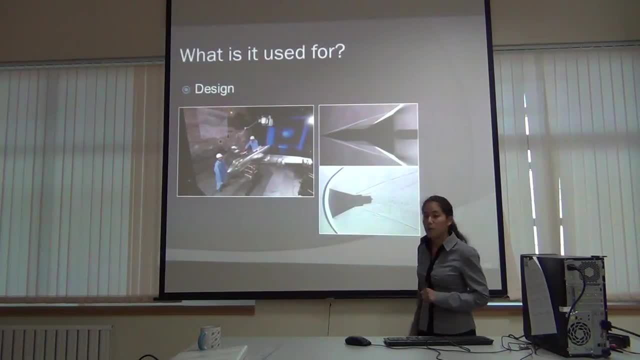 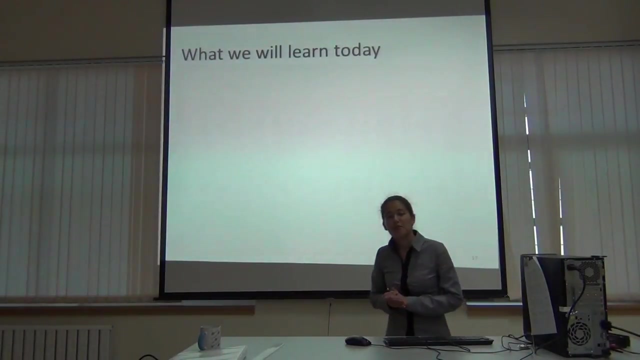 And this makes it better, Because we can come up with materials That will withstand the temperatures On the descent On this capsule with astronauts, for example. Alright, So now let's learn the basic principles of aerodynamics And we will proceed with the whiteboard. 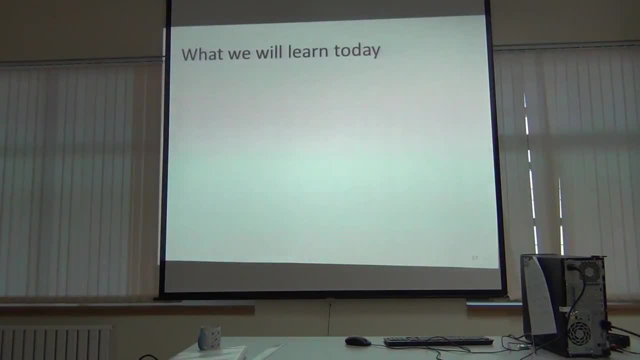 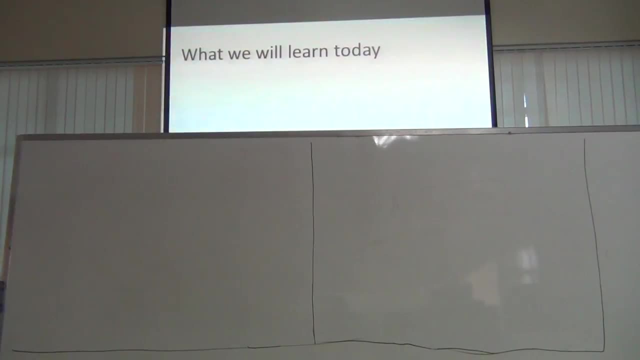 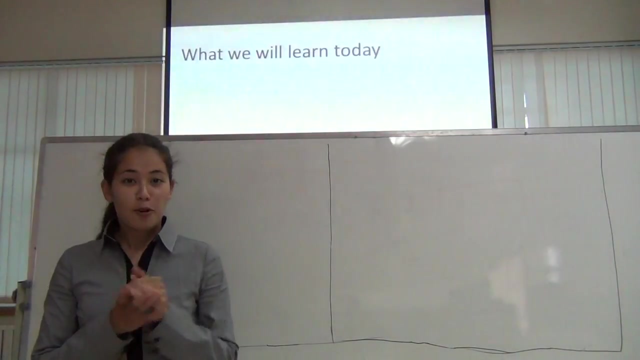 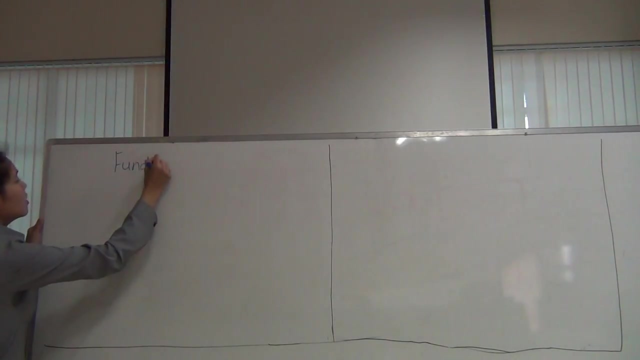 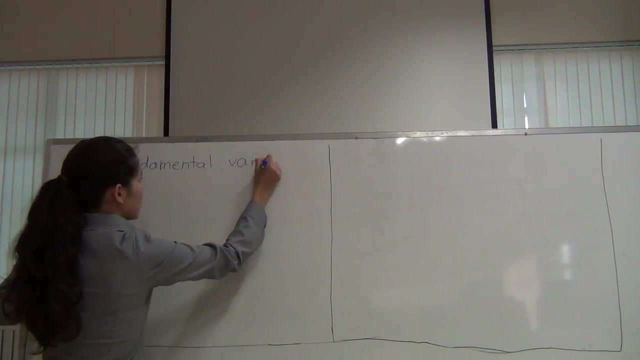 Let me get it here, Okay. So Before we start, Let us review some variables That we know from physics already, But these variables are used a lot in aerodynamics. I got my marker Okay, So let me write it down. 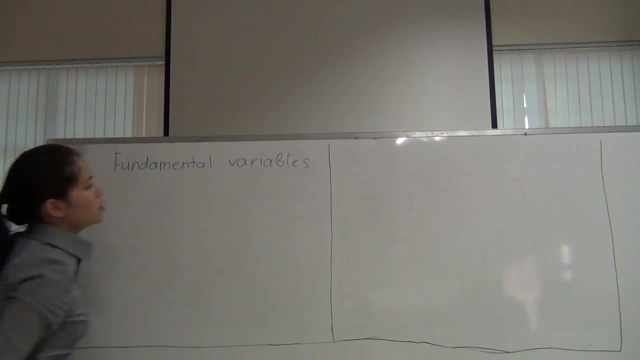 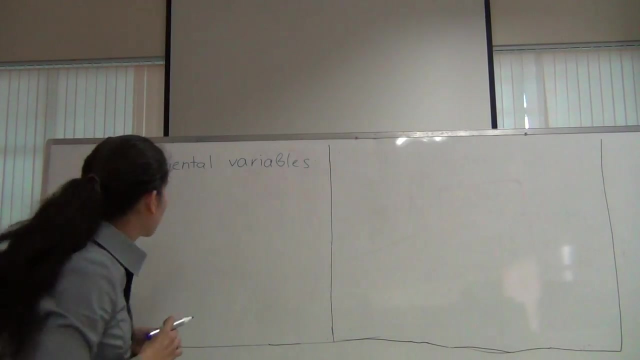 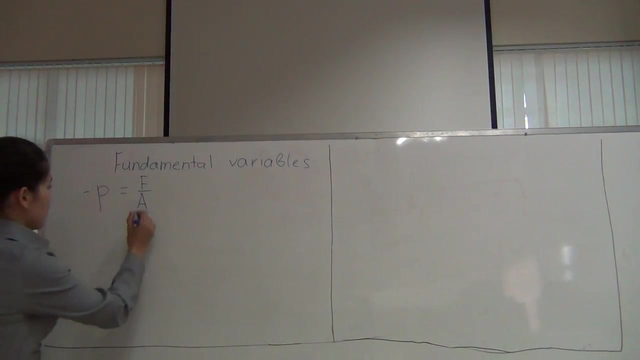 Fundamental variables. The first one is pressure, And pressure is Normal force acting on the surface of a unit area. So let me define it here as Force divided by area. And so if we have a surface like this Which is of unit area, 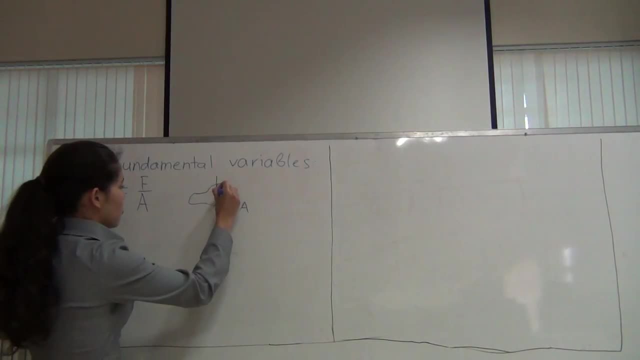 The pressure will be The force that acts on this area, And it, The force, should act perpendicularly In order to measure pressure correctly. So pressure is measured in Newton per meter squared, Or in English units. It will be. 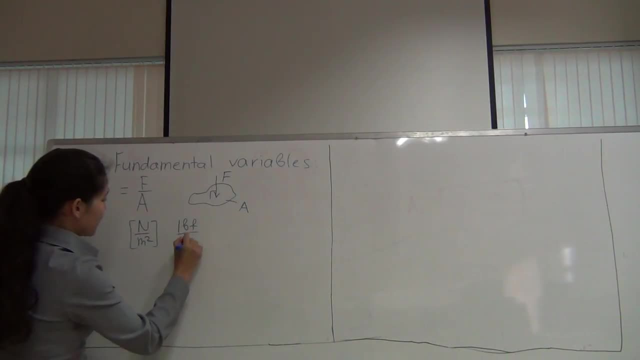 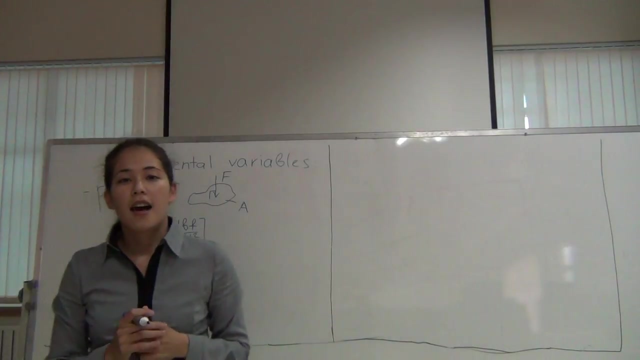 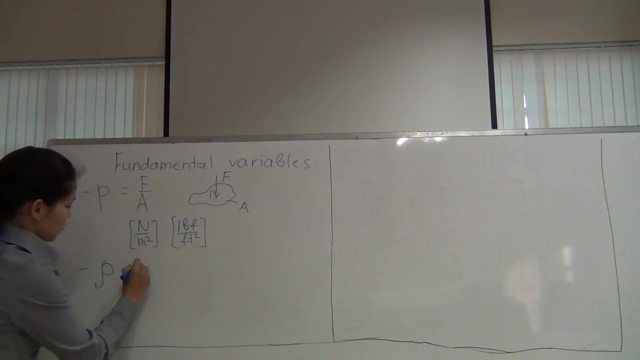 Pound force Per feet squared. So I hope you remember this from your physics. This is just a quick review. The next variable is Density, And density is How much substance you have in a unit volume. So density equals to mass divided by volume. 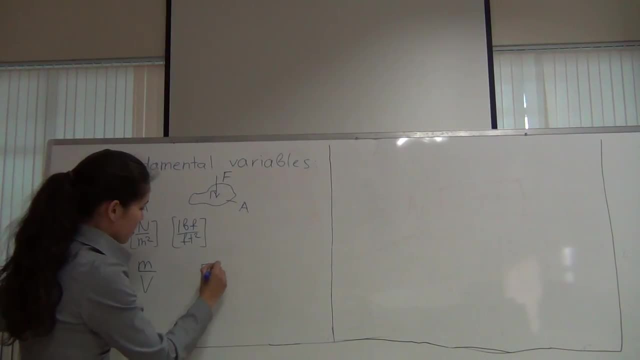 If you have a volume, A unit volume, Like this cube, for example, Then the density of the substance inside this cube Will be equal to mass Of the substance divided by the volume. Alright, And density is measured in Kilograms. 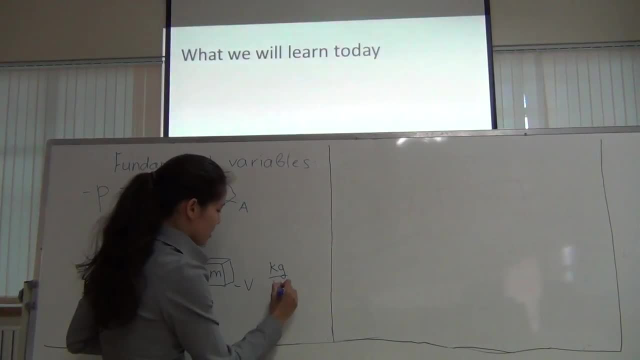 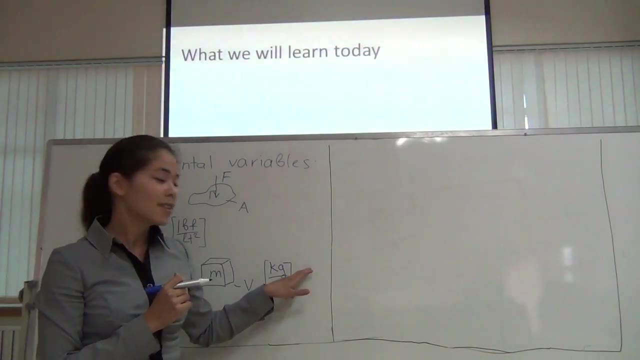 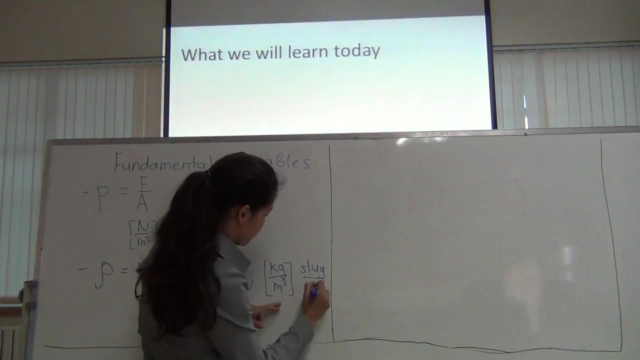 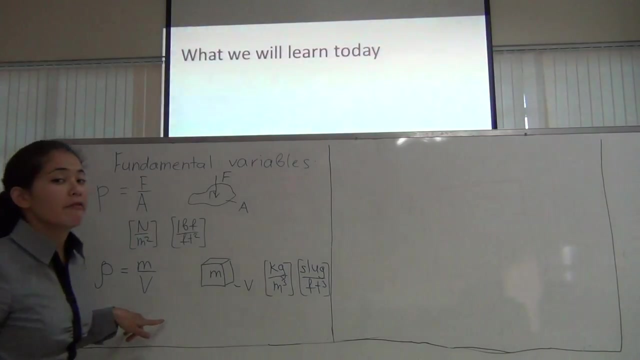 Per meter squared, Meter cubed, Sorry, Or in English units, It will be Slugs Per Feet cubed. Alright, And the final variable that we will use a lot today Is velocity, And I will write it down like a small v here: 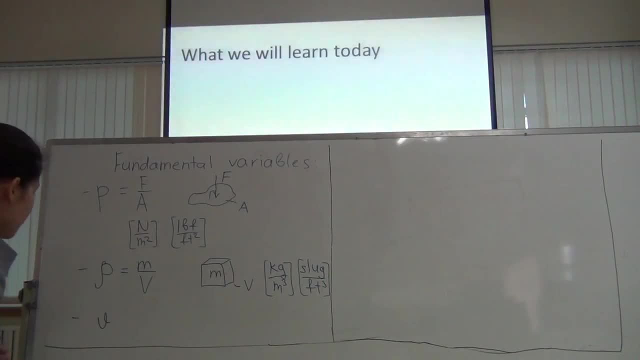 So that we will not confuse it with volume. So velocity is the rate of change of position In time. So if we have position denoted by x, Like here, Velocity will be Derivative of x With respect to time And velocity. 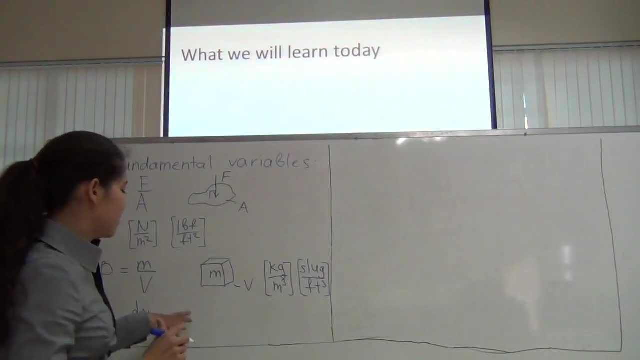 Has a magnitude, Which means that You can have high speed or low speed. Alright, Let me denote it here as Small vector, Small arrow And big arrow. But also velocity has a direction, Which means You can go in this direction. 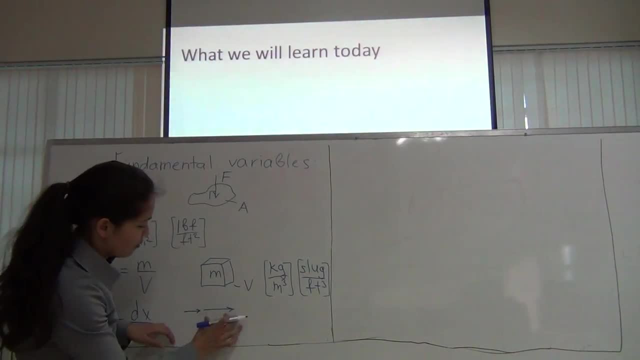 Or in the other direction. And that makes Velocity A vector quantity. So velocity Is a vector quantity. So velocity Is a vector quantity, Which means You can go in this direction Or in the other direction, And that makes 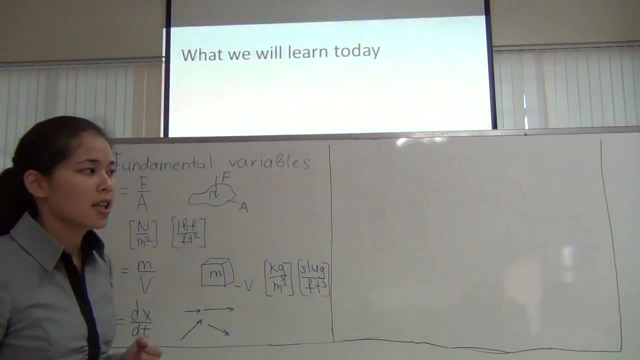 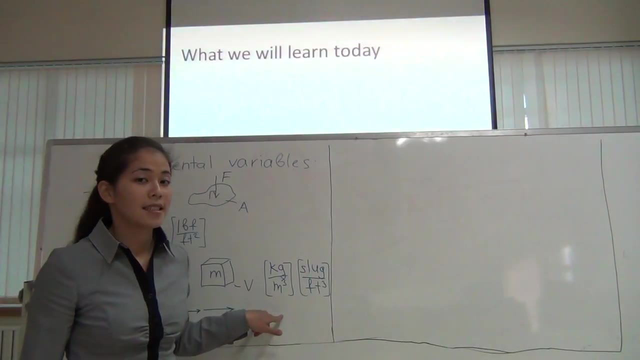 Velocity A vector quantity. So that means If either of them changes, Velocity changes. And if your speed is, Speed stays the same, But Direction changes, That will Change the velocity. Okay, So We've Reviewed. 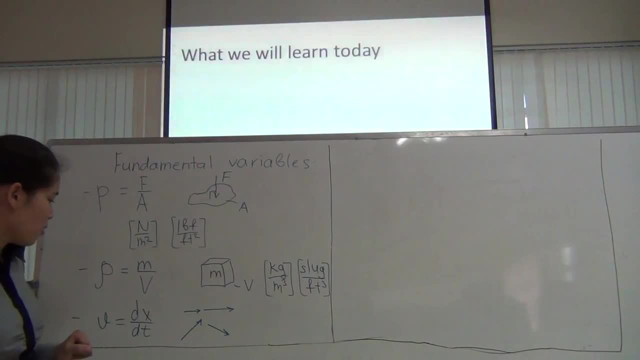 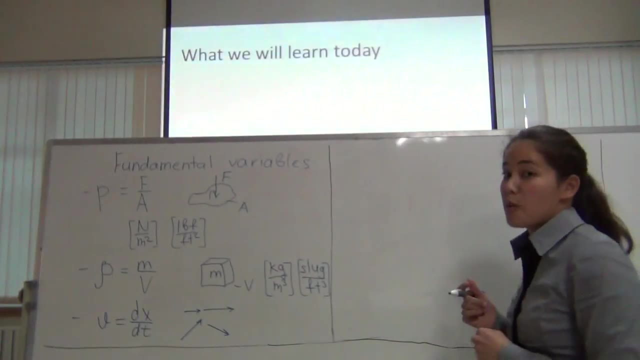 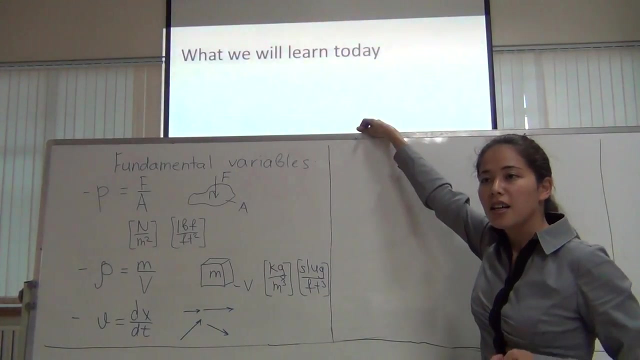 That. But now, Since we will Study Aircraft, We need To learn Some of the terminology Of the aircraft And That will be Just. It will be just Wing terminology, Because The Aircraft We will. 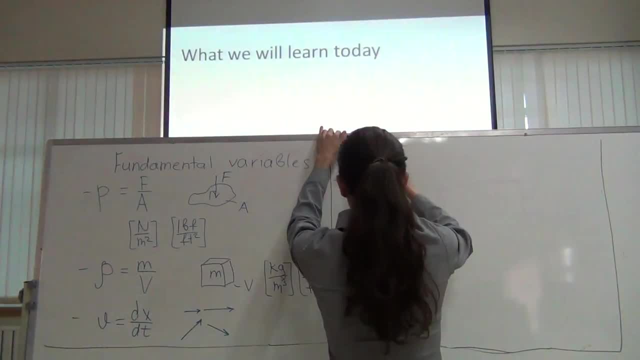 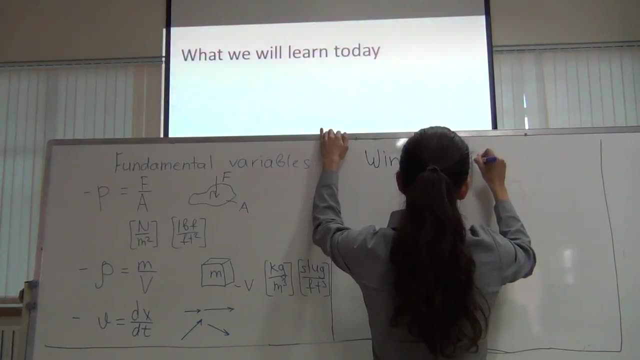 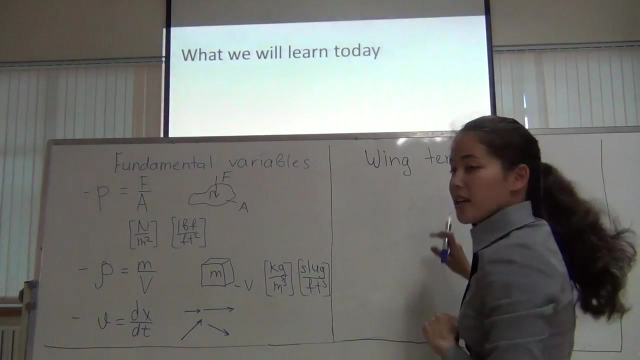 Cover just Basics Today. So Let's Look At The Wing. From The Top, We will See A Shape Like This, So Let's Look At The Wing. 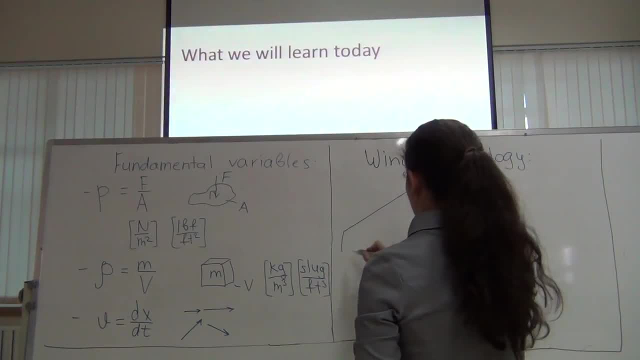 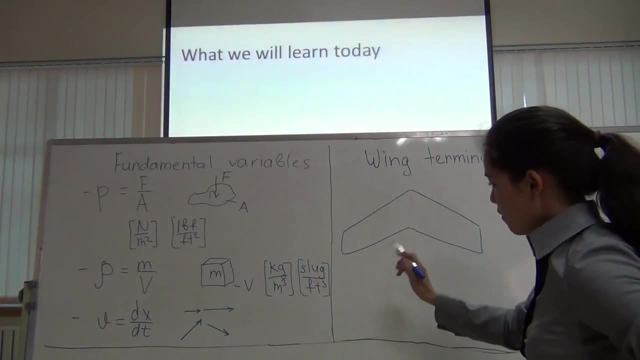 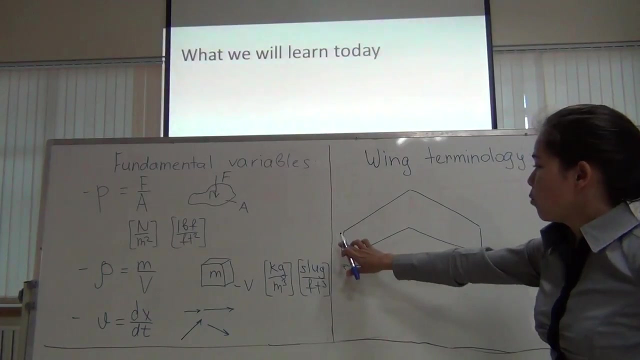 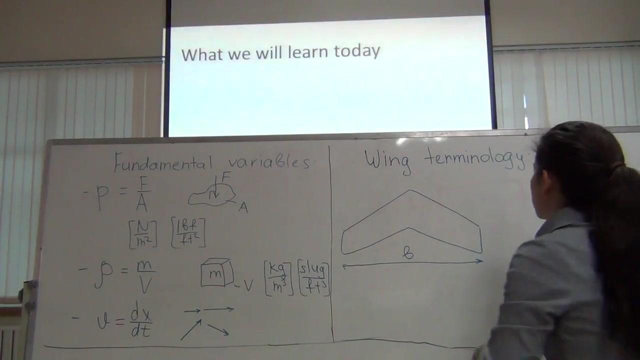 From The Top. We will Look At The Wing. So First Of All, We Define This Distance From One, One End Of The Wing To The 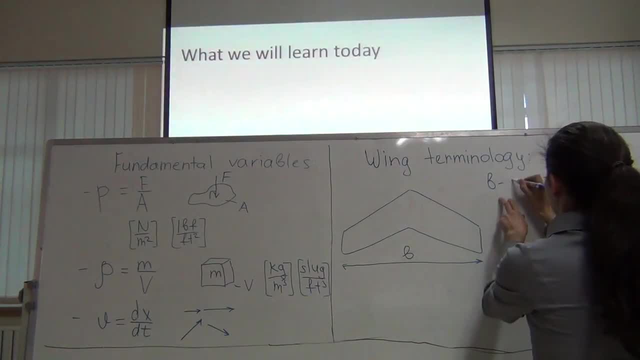 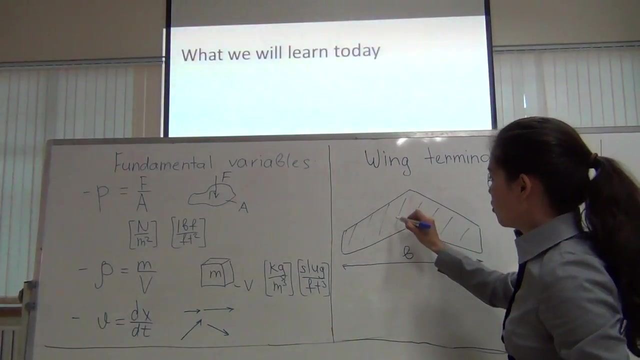 Other End It Is Denoted As B And S. All Right. Next One Is The Area Of The Wing, So Wings Can Be Different Shapes. 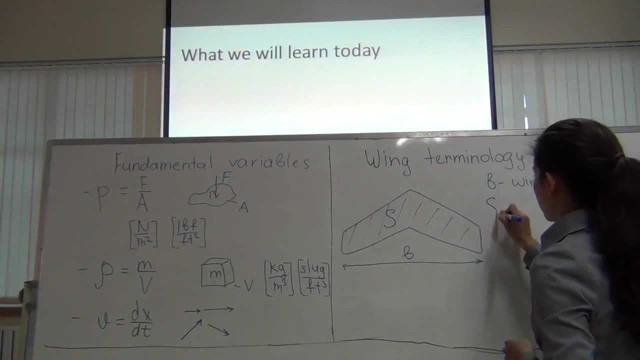 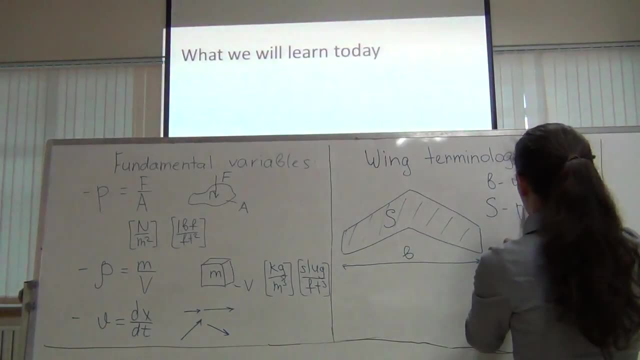 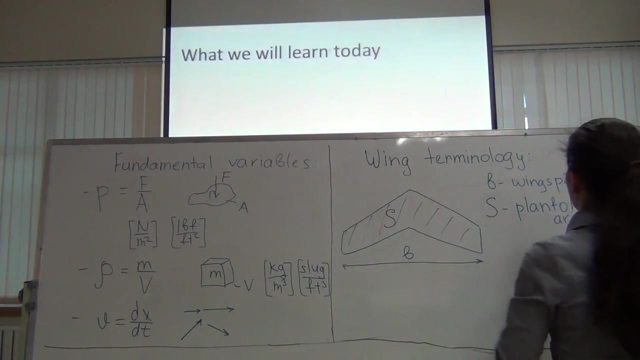 But Area Is Measured Without Taking Into Account The Shape, So Let's Denote Next. We Have Some Air Coming At The Wing And Travel. 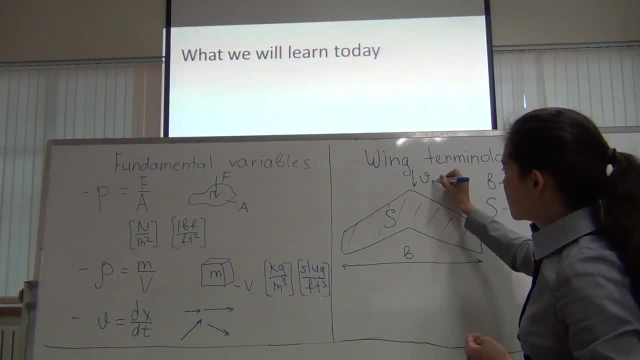 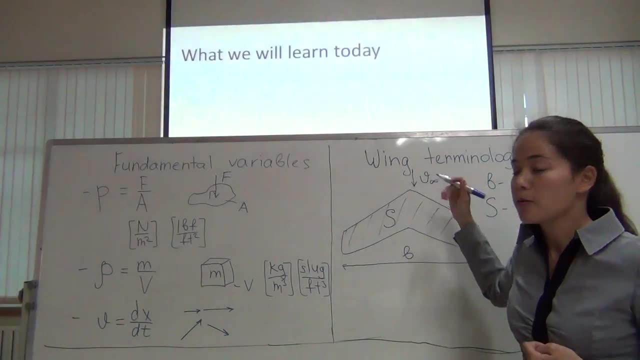 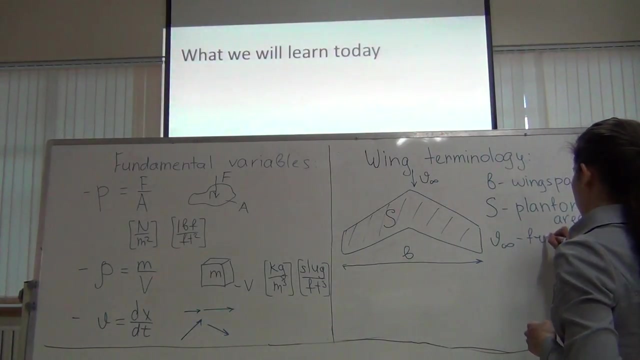 That Some Speed That We Denote As The Infinity, Which Means Free Stream Velocity. That Is The Velocity, Far Free Stream Velocity. Next Is This: 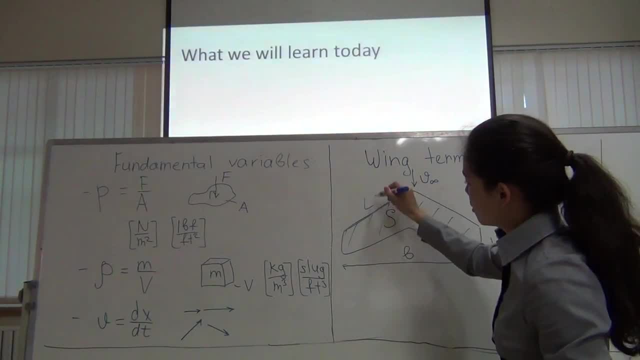 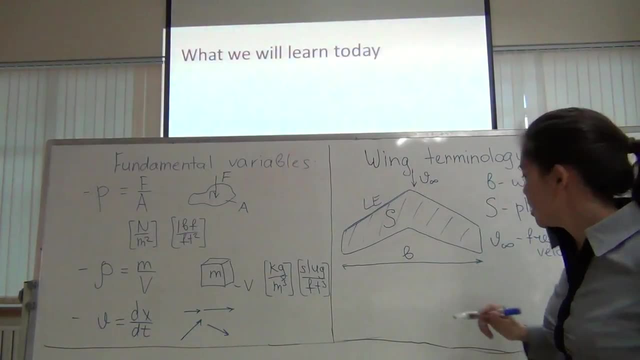 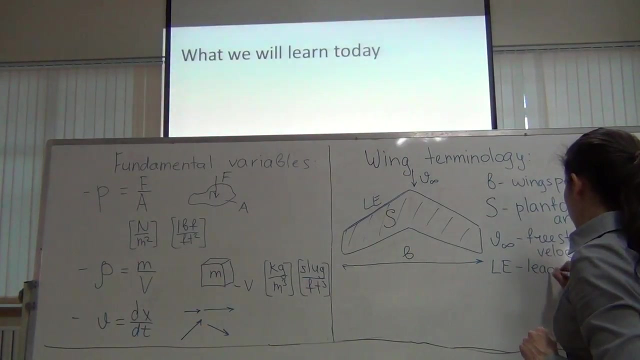 Edge Of The Wing. It Is Called The Leading Edge Because It The First One To Meet The Leading Edge And Obviously There Is Also The 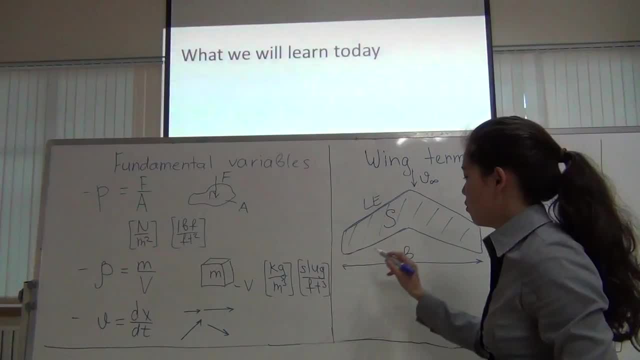 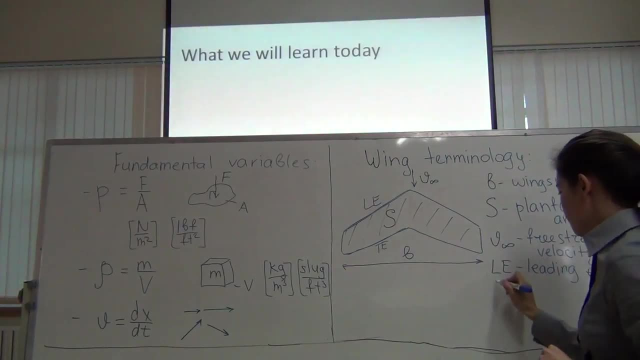 Other Edge Of The Wing, Which Is Called The Trailing Edge, And It's The Last One To Go Into The Flow. Okay, And The Last. 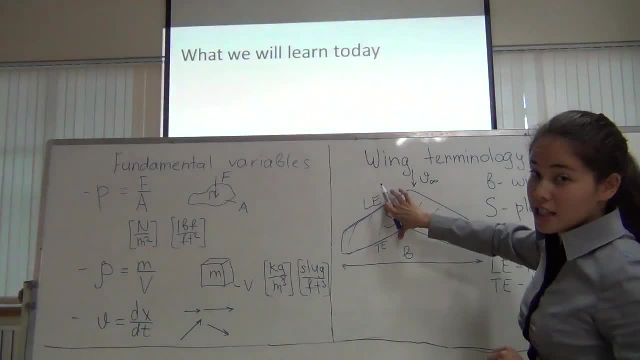 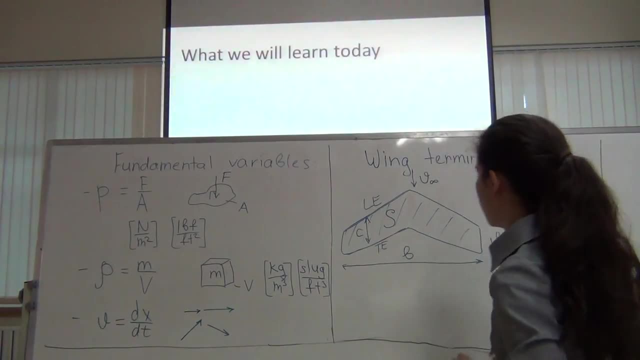 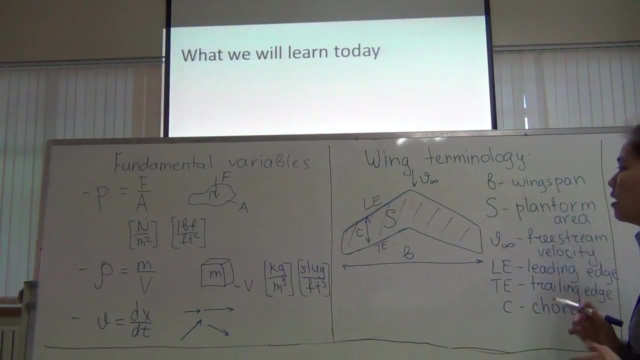 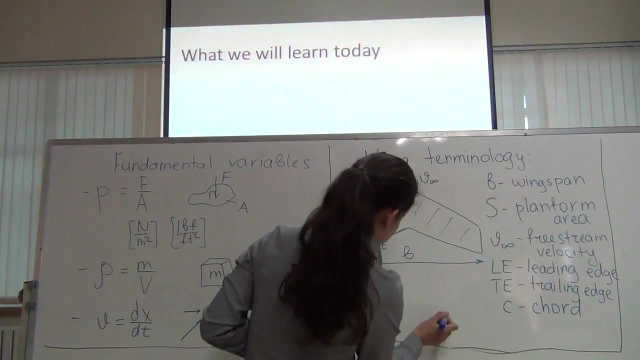 Variable That We Will Use Today Is The Distance Between The Leading Edge And The Trailing Edge. It Is Called Cord And Is Denoted By. 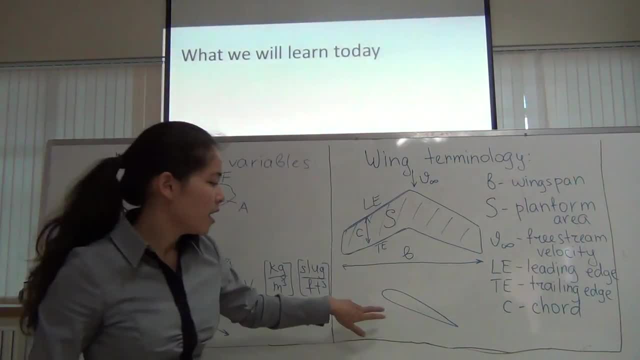 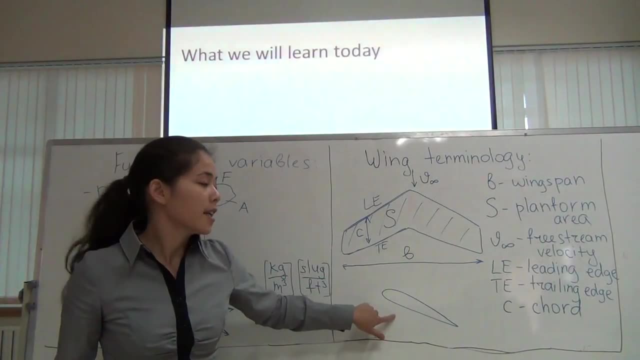 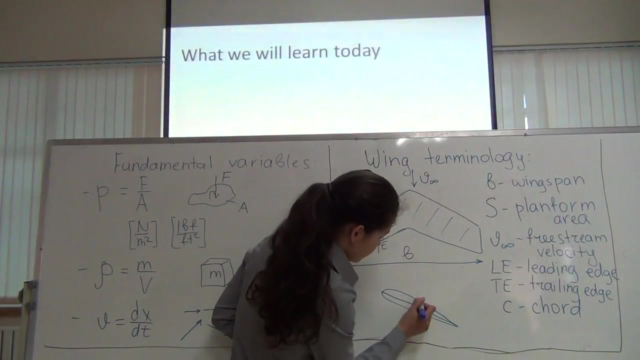 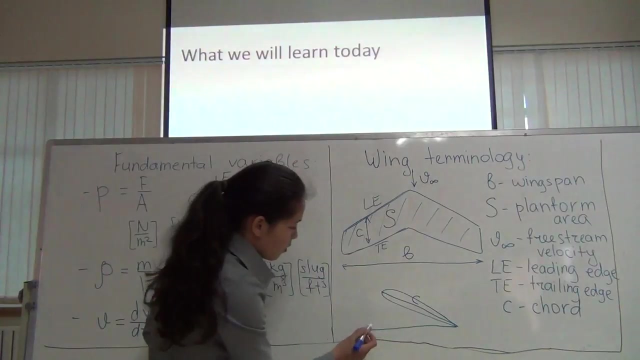 The Wing. So If We Cut Out A Section Of The Wing, We Will Have A Shape Like This And You Will Learn Today Why Wings. 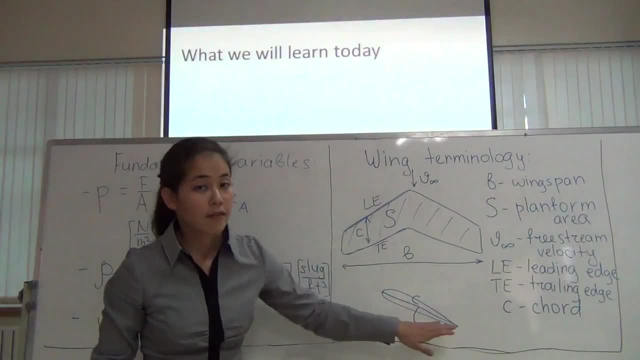 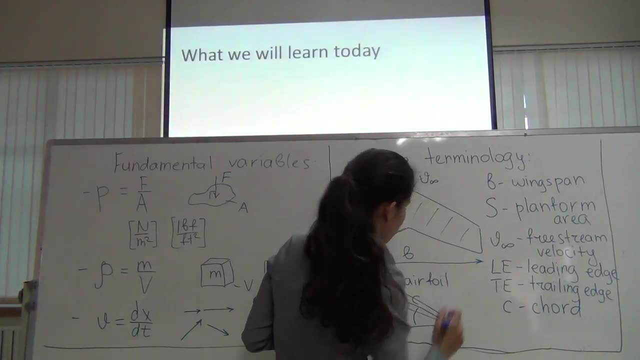 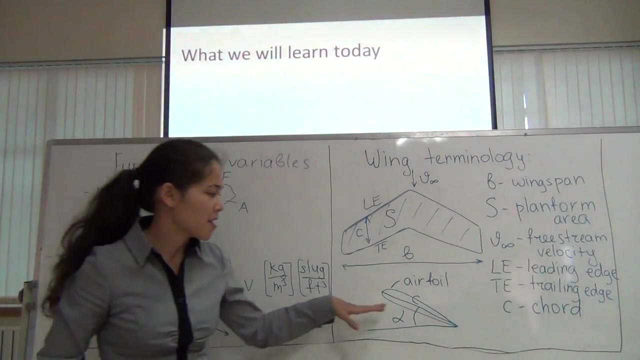 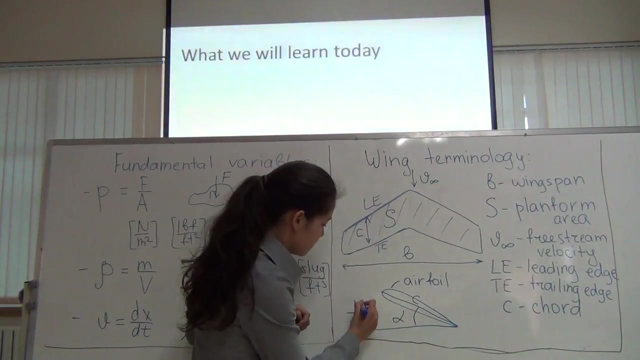 Are Shaped. So This Shape Is Called The Airfoil Or Profile Of The Wing. So Angle Of Attack Is Denoted By Alpha And It 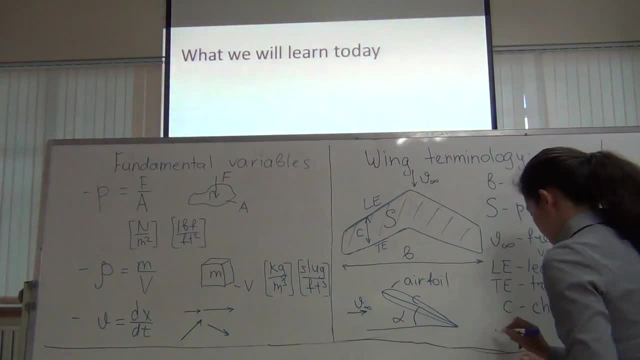 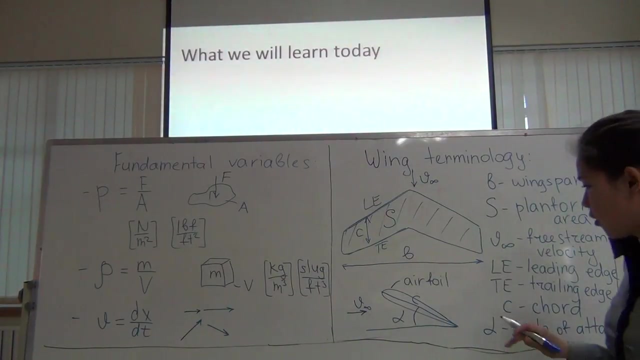 Is How Much The Airfoil Is Shaped, Like A Section Of The Wing Of The Airfoil Is Shaped, So This Will Be Good Enough. 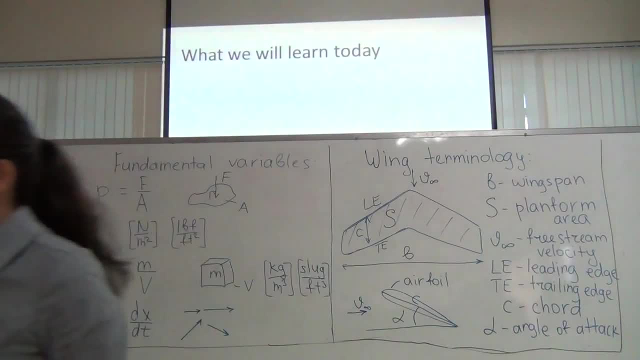 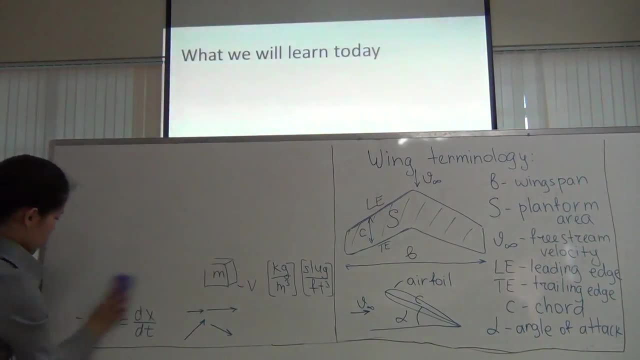 For Today's Lecture, For Wing Terminology. Now Let's Actually Learn Why Wings Fly. So, In Order To Understand Why Wings Fly, Let's Start With. 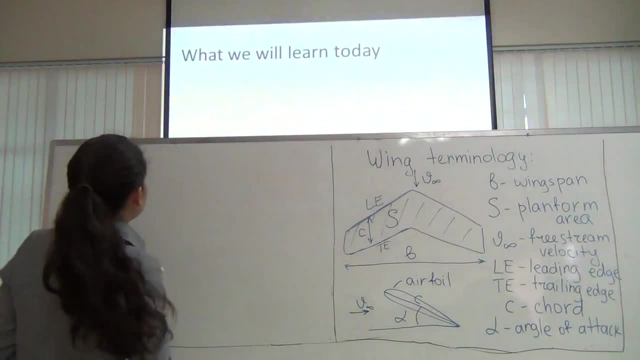 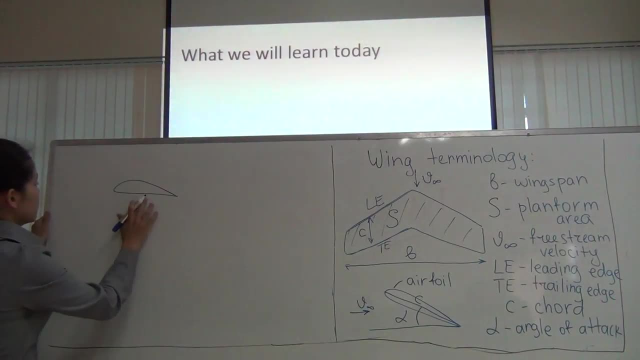 Airfoil In The Wing Tunnel. Let's Draw It Here. So This Is Our Airfoil And The Wing Tunnel. So If We Follow One Particle, 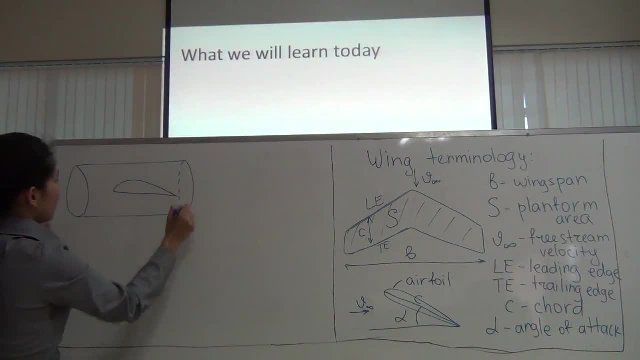 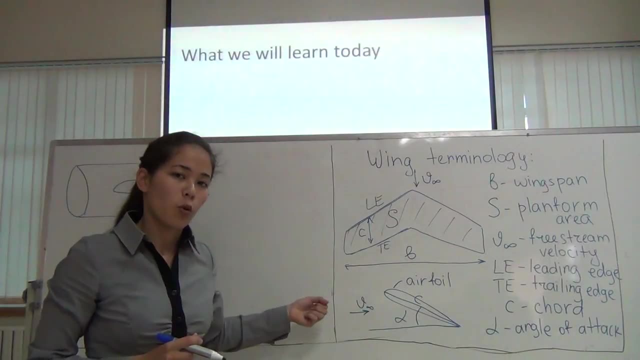 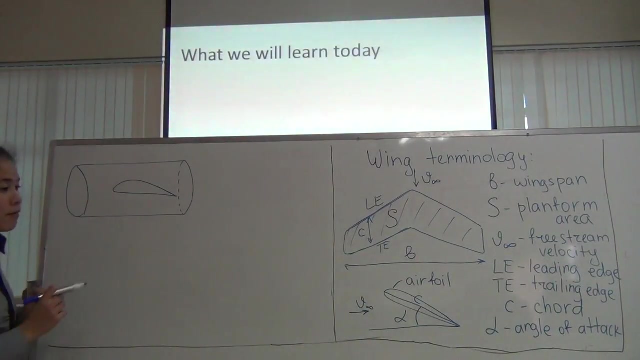 Into The Wing Tunnel. So We Tunnel Basically Just Imitates The Flow Of Air, As If The Airfoil Was Actually Flying In The Wing. 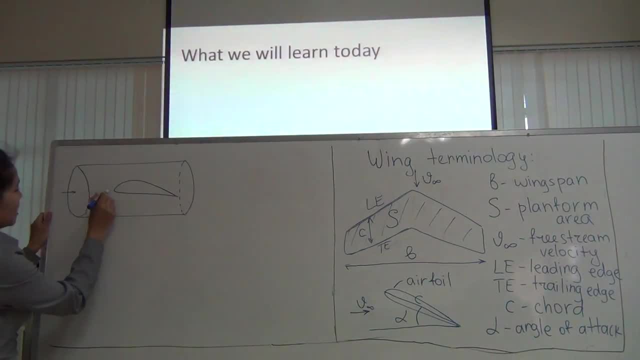 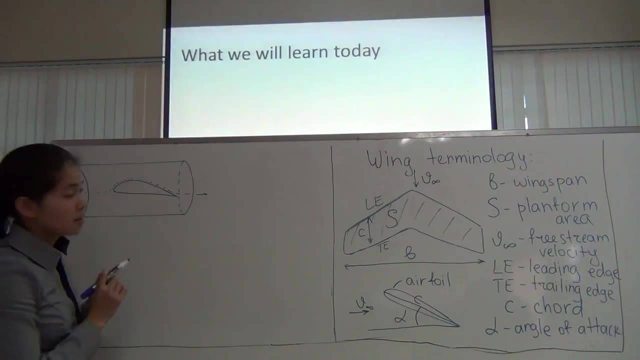 Tunnel. We Have One Air Particle Comes Here And Going Around The Airfoil And Exits At The Other Side And If We Follow Another Particle, 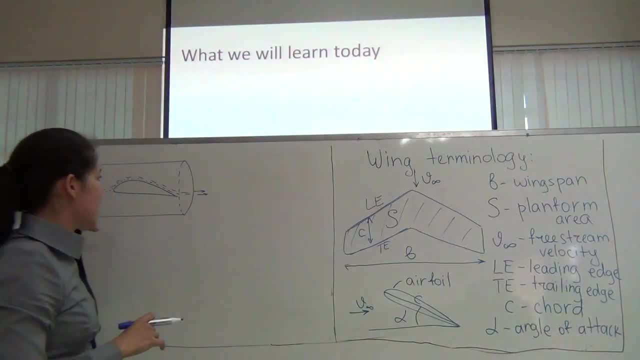 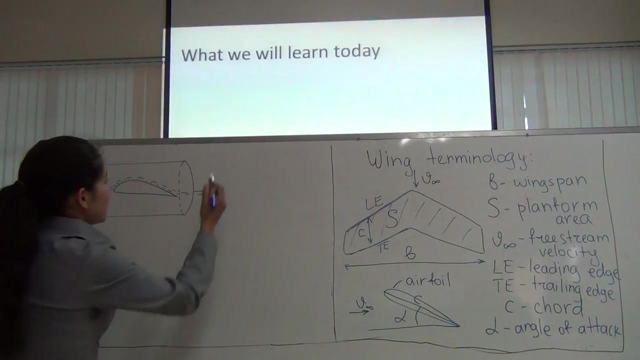 It Will Do. Whatever Mass Enters, The Wind Tunnel Also Exits At The Other Side, Because The Walls Of The Wind Tunnel Can Not Make. 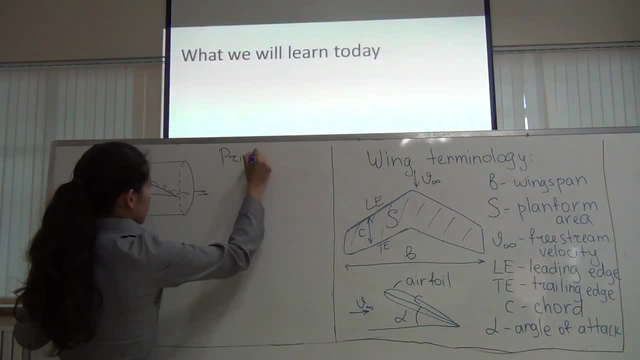 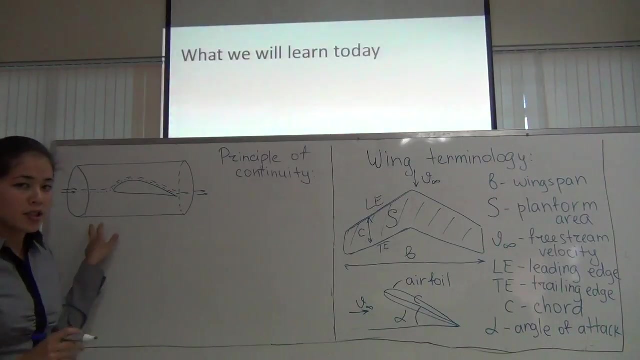 Any Particles Leave, The Wind Tunnel Exits At The Out In The End Of The Wind. Okay, Let's Introduce Some Numbers Here So That 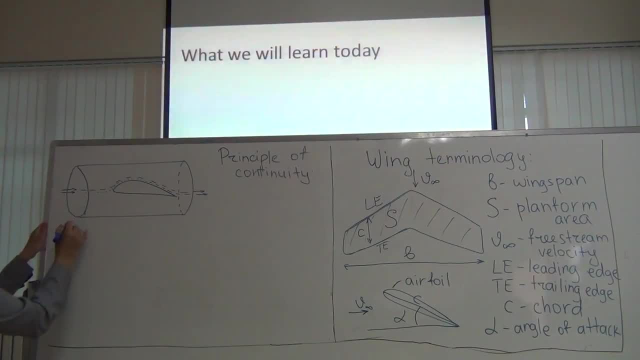 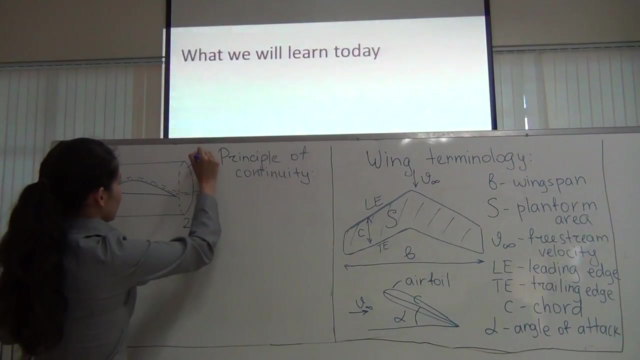 We Can Mathematically Put It, Write It Down. So Let's Name The Outlet, And The Area Of The Outlet Will Be A Two. So 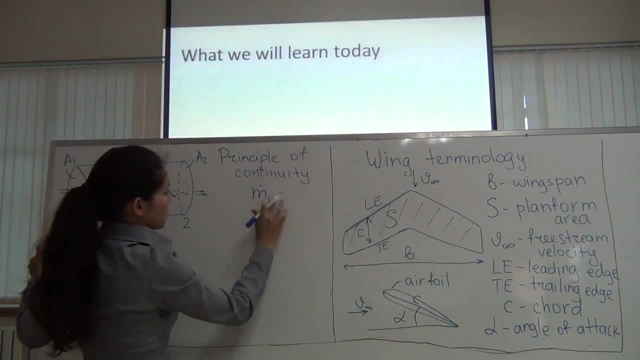 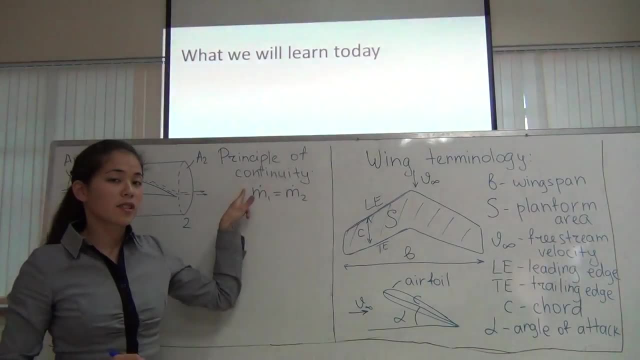 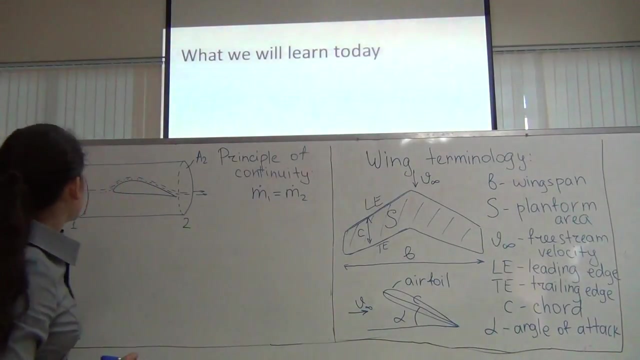 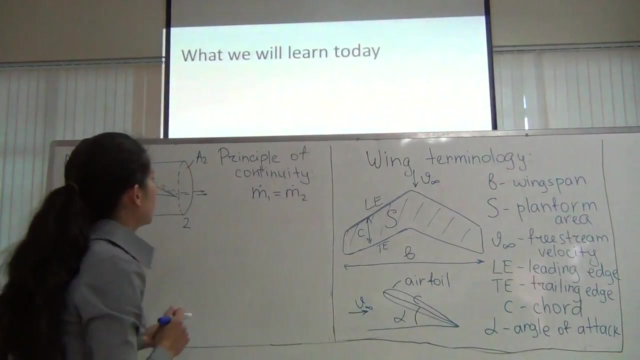 Principle Of Continuity Will Tell Us That M Dot One And One Dot Is Equal To M Two. Entering The Wind Tunnel Per Second Is: 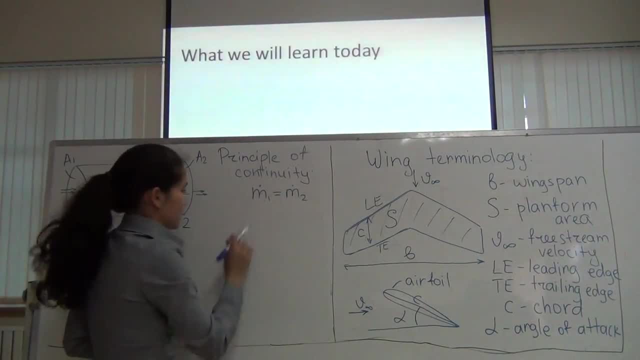 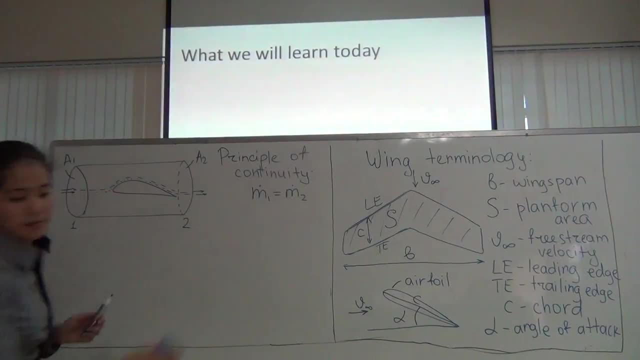 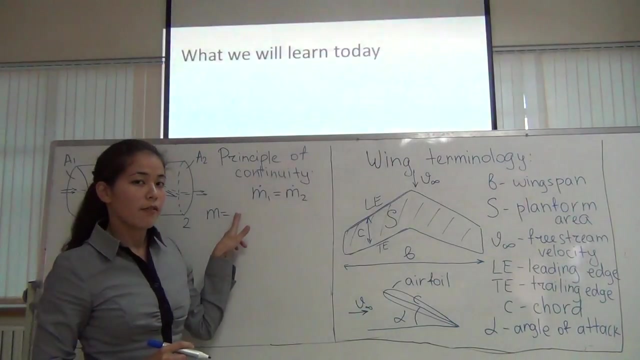 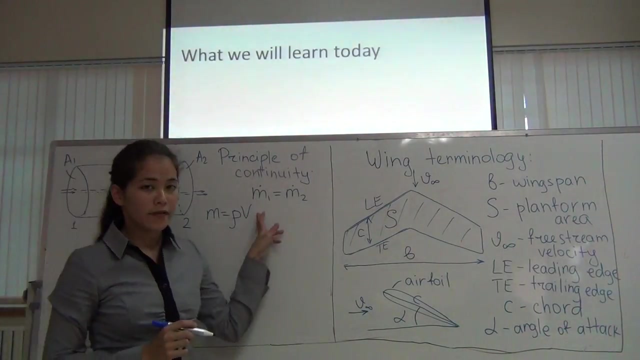 Equal To The Same Mass Exiting The Wind Tunnel. Okay, Now Let's Remember What Mass Is. Mass Is Equal Mass Equals Density, And What Is. 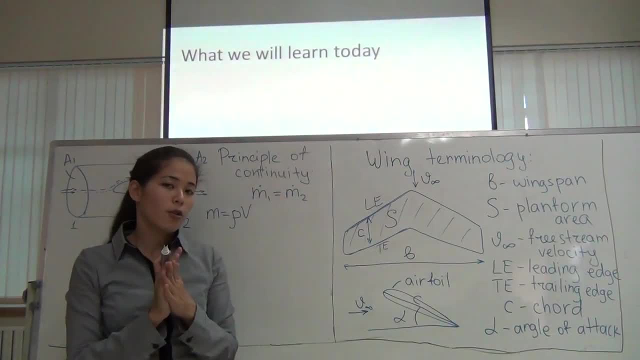 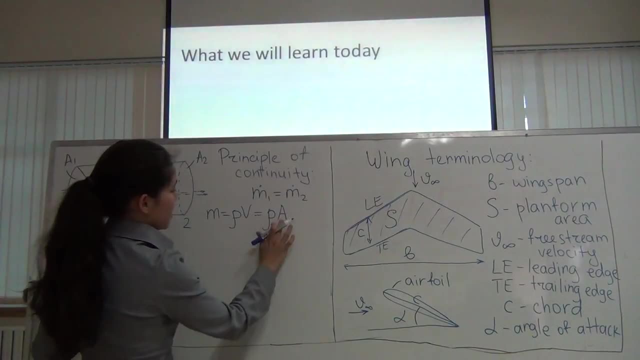 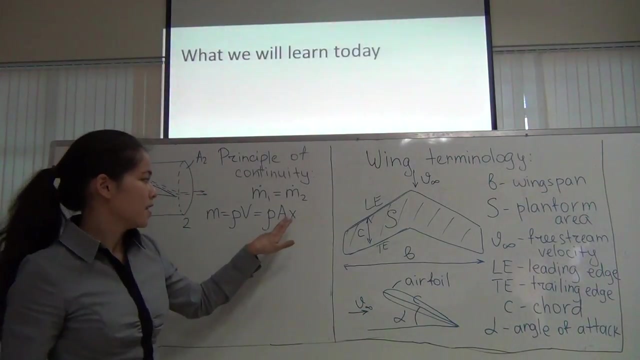 Volume. Volume Is Area Multiplied By Distance For Which That Area Is Transferred. So Area Is A, Rho Is Distance, And Let's Say X. 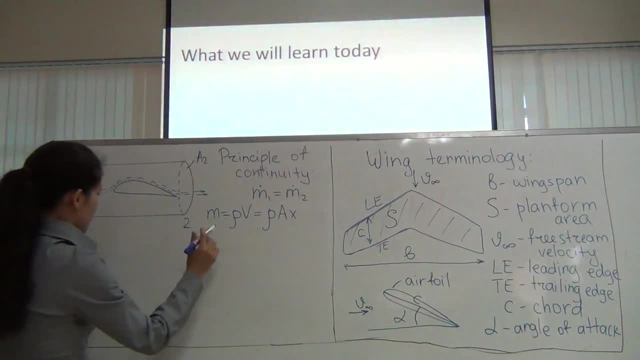 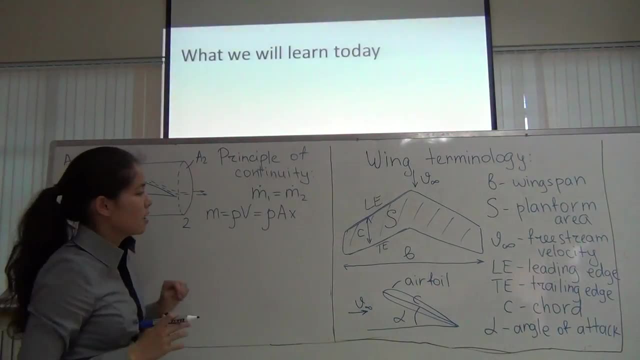 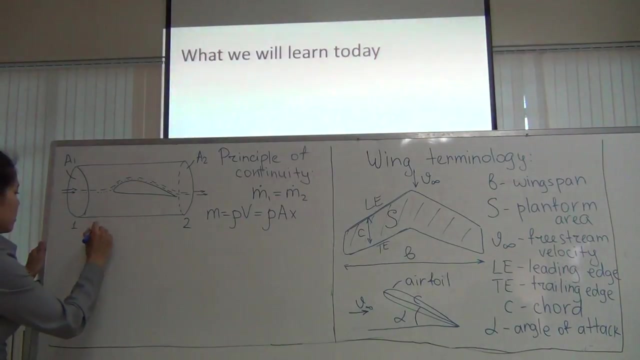 Is Into This Equation That Will Give Us. So We Said That Dot Means The Derivative. With Respected Time, Let's Write It Down As: 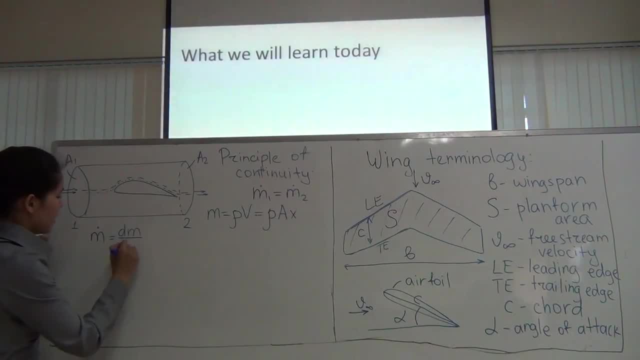 M Dot Equals Derivative Of Mass Flow. So If We Substitute Now This Expression Here We Can Say Derivative Of Rho A X, Per. 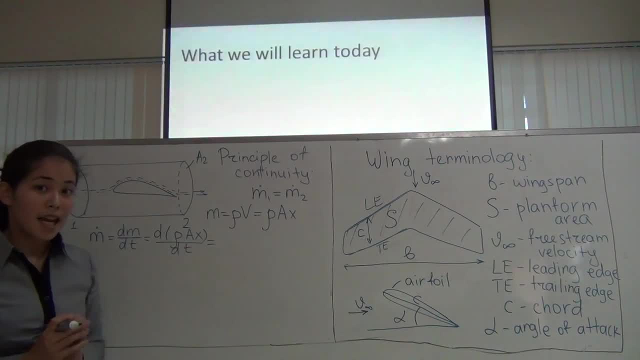 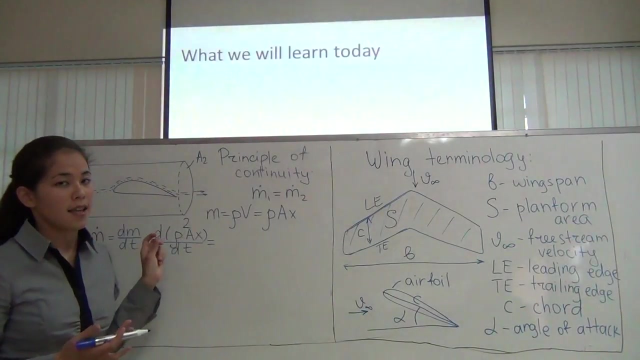 Time. So D T, And Now It's Time To Make Some Assumptions. So That Exits, That Means The Density Of This Area Will Stay. 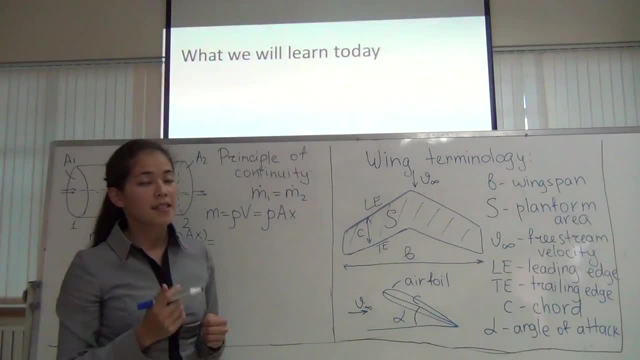 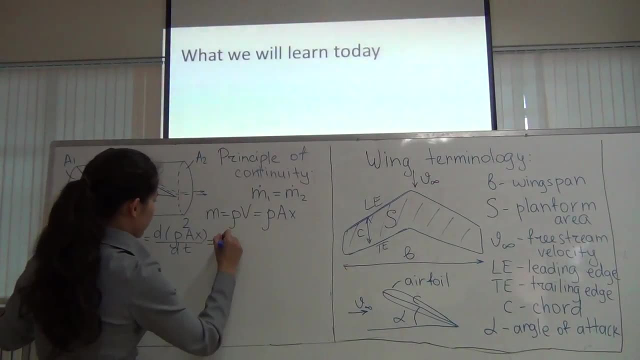 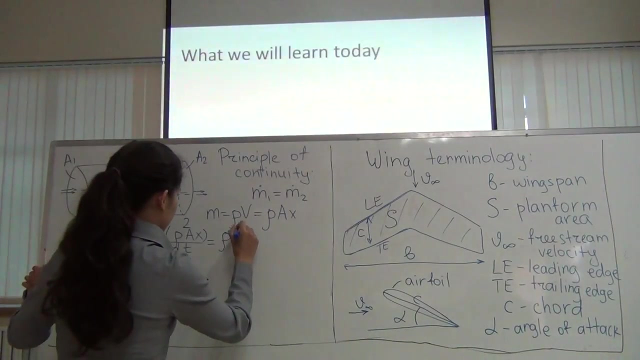 The Same, If We Assume Not The Supersonic Flow, So That Means The Density Is Constant And In, So That Will Give Us Derivative Of 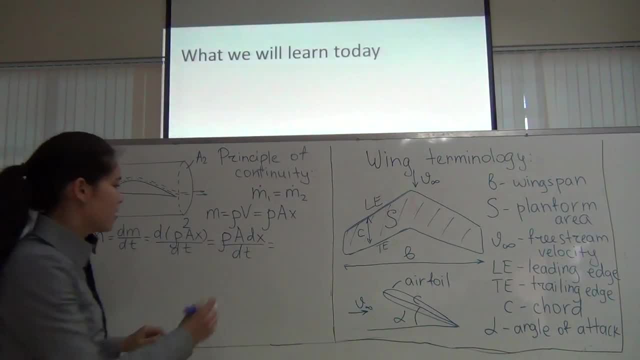 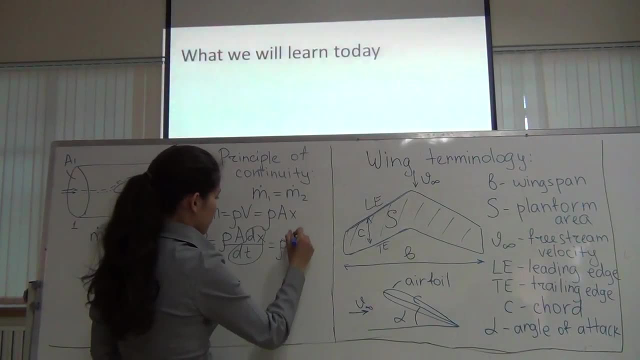 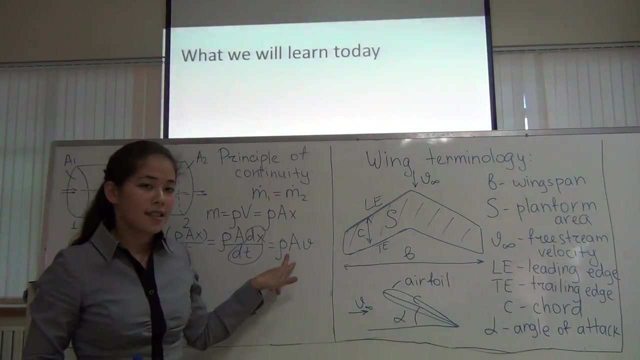 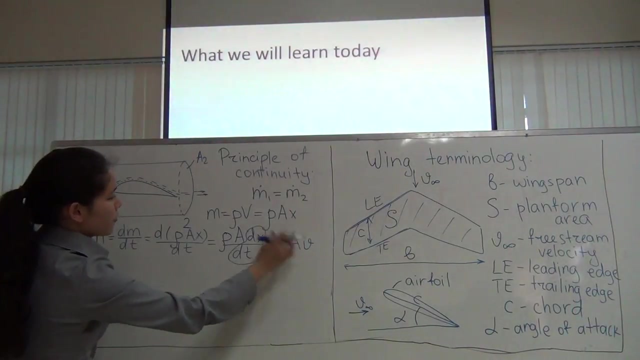 Distance With Respect To Time, And We Remember That This Expression Is Equal To Velocity, So That Means We Can Write It, So Now We Can. 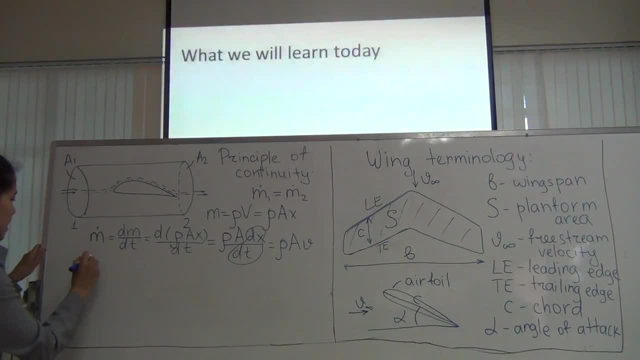 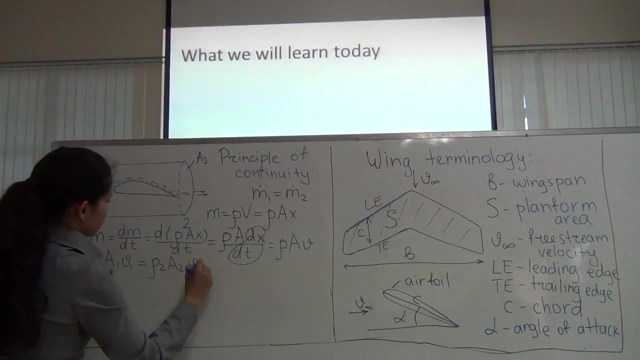 Substitute This Expression For M Dot In This Equation. Let's Do It And We Will Get Row One A One E One Equal To Row. 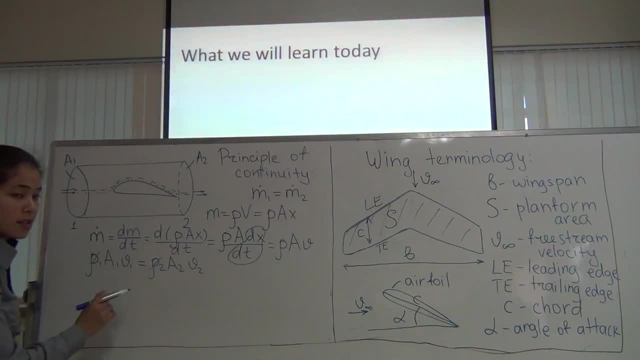 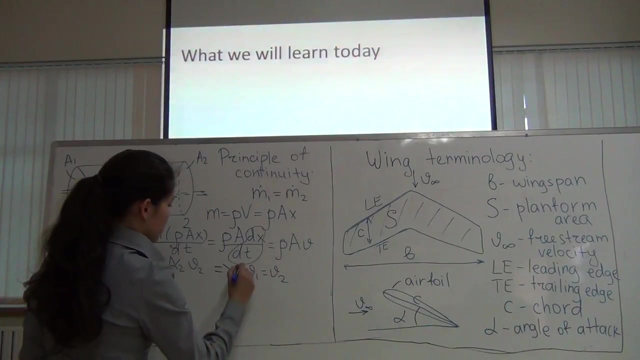 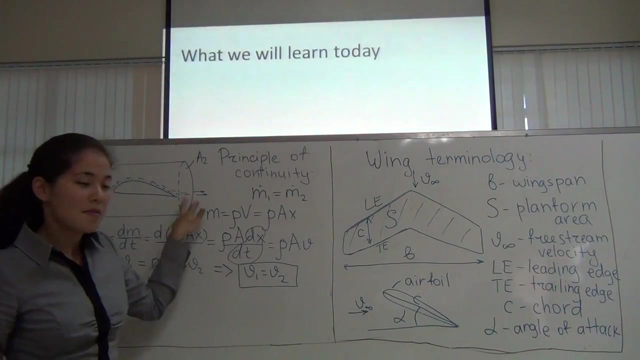 Two, We Can Cross It Out From Both Sides Of The Equation. The Areas Are The Same By Geometry, So We Can Cross Them Out. 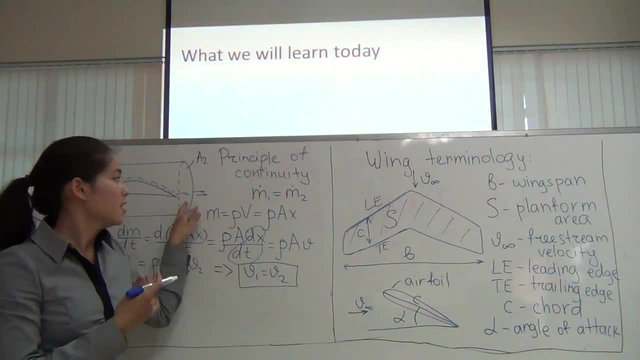 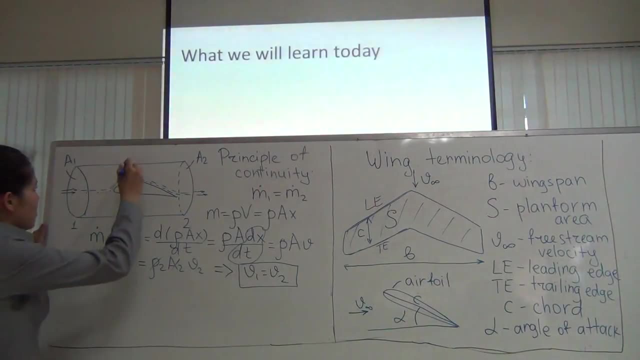 And That Will Give Us That. So It's Pretty Logical. But Now Let's See What Happens If We Change Our Wind Tunnel A Little. 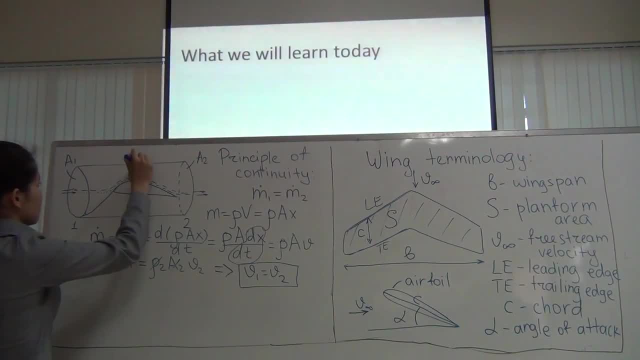 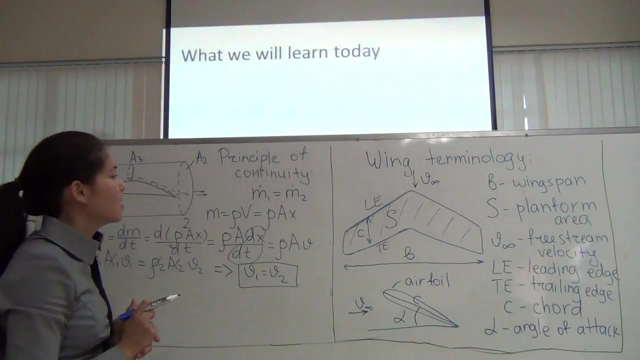 Bit And Put The Exit Right Here Above The Airflow And Through This Part Which Is A3. But Principle Of Continuity Still Applies, So 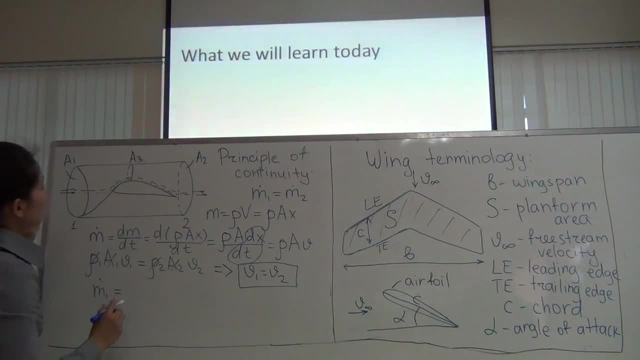 We Can Say That M1. Whatever Enters In The Wind Tunnel Should Be Equal. Whatever Is Right. This Will Give Us R1.. A1., V1.. 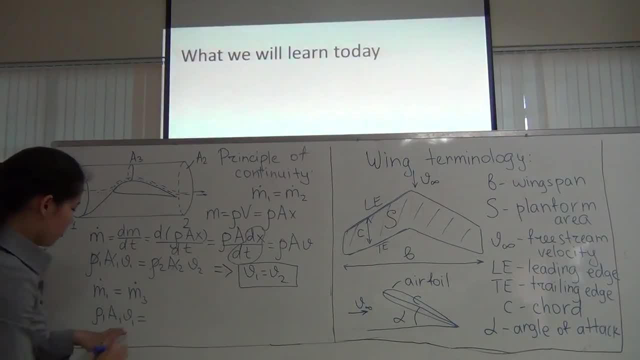 Equal To R3., A3., V3. And We Can Make The Same Assumption For The Density. We Assume That Incompressible Flow At Low To. 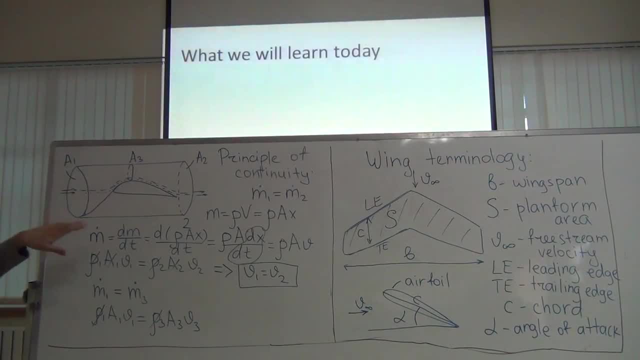 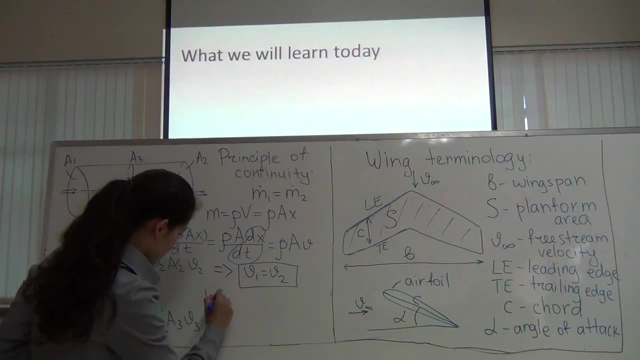 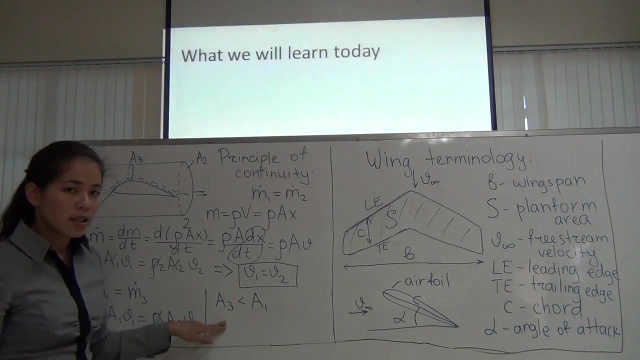 A3. V3. But We Know That A3. Is A lot Smaller Than A1. Let's Write It Down Here. So A3. Is Smaller. 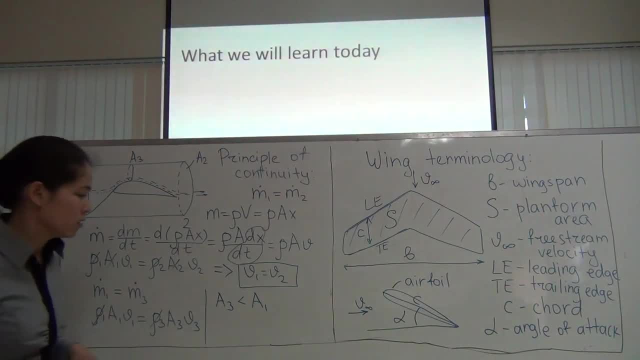 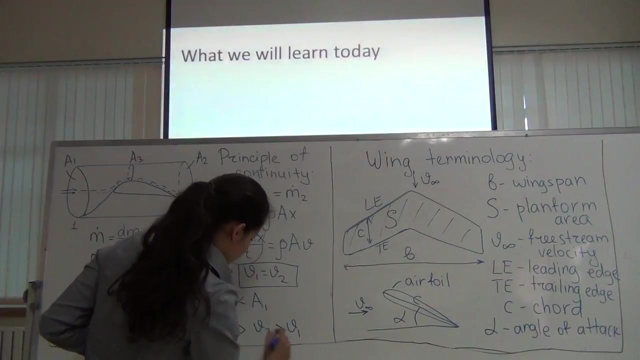 Than A1. And This Will From This Assumption That The Velocity Of The Air In The Section With Smaller Area Is Larger Than The 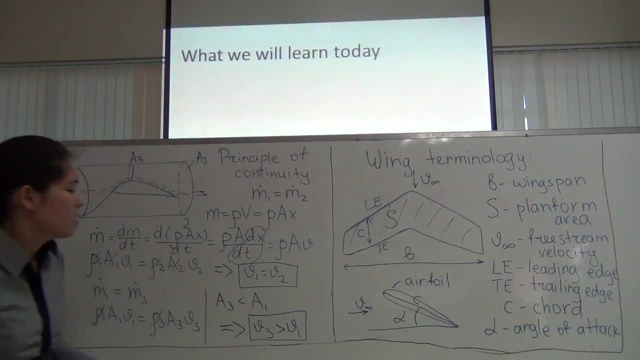 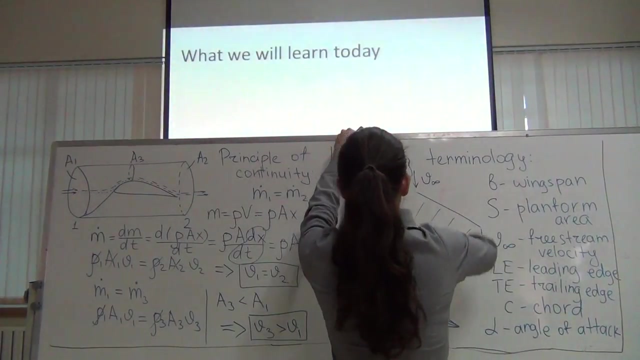 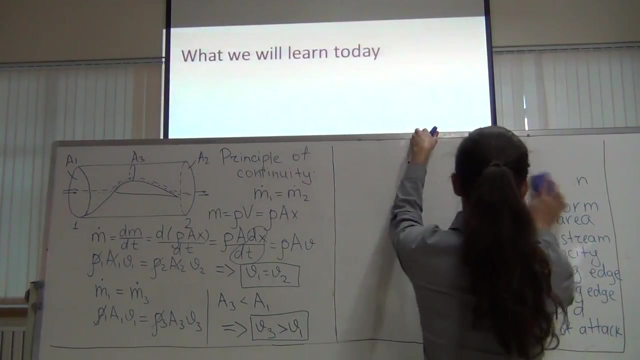 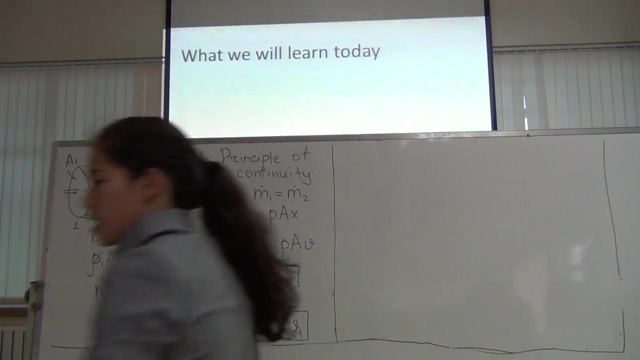 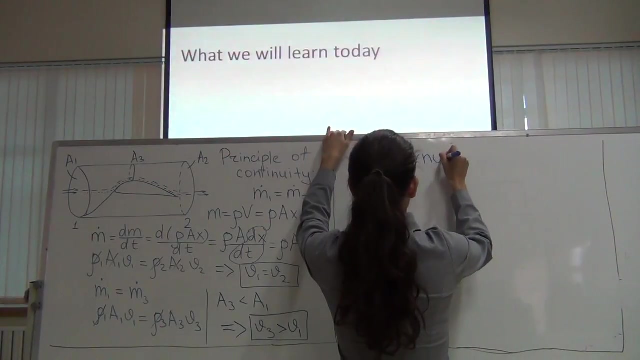 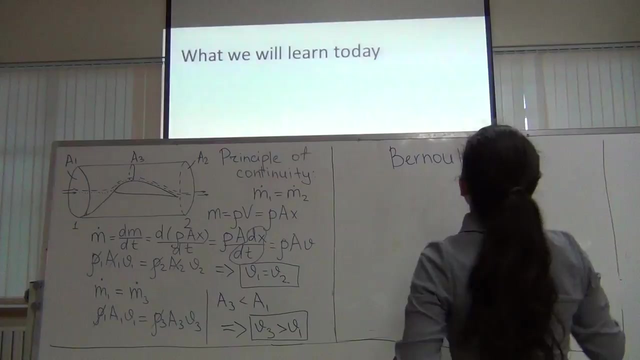 Velocity Of The Air In The Section With Larger Area. Okay, Let's Derive The Bernoulli's Equation. So, In Order To Derive Bernoulli's, 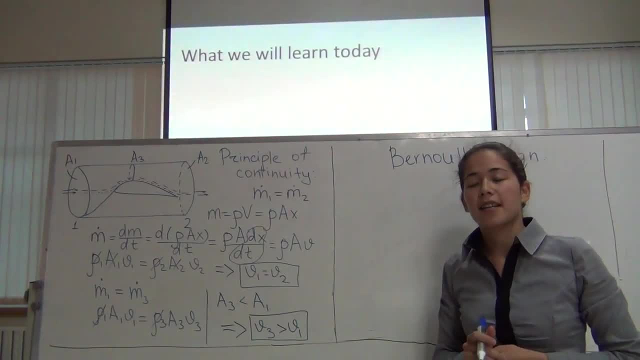 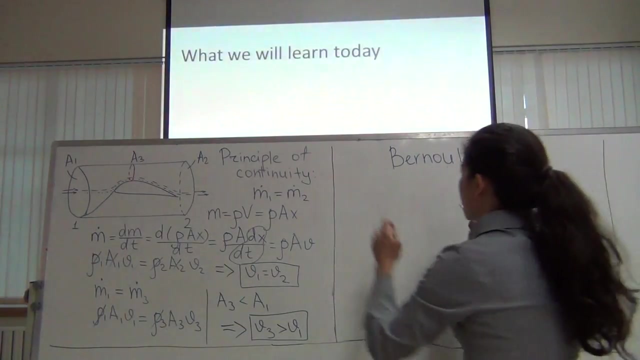 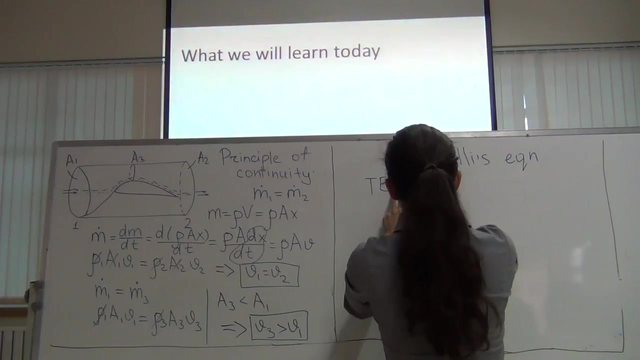 Equation We Apply Basic Physics Principle That Energy Can Be Neither Created Nor Destroyed. So That Means That Energy Is Total, Energy Is Equal To. 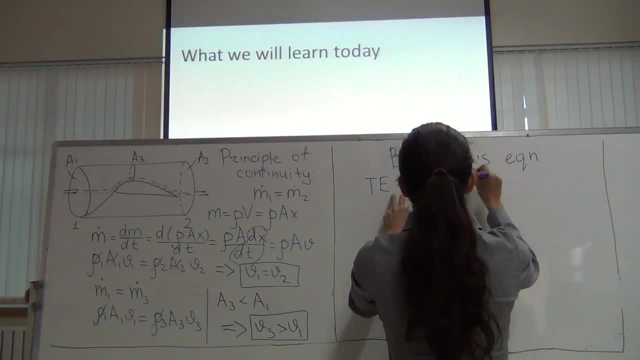 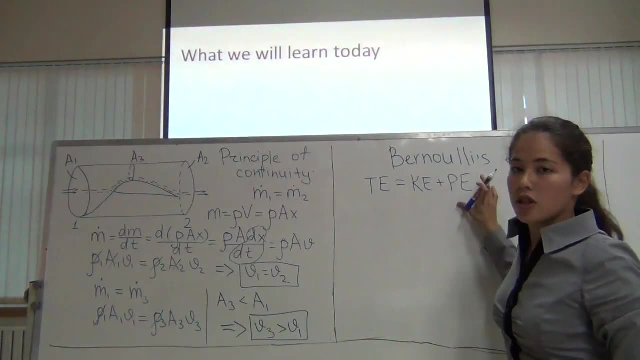 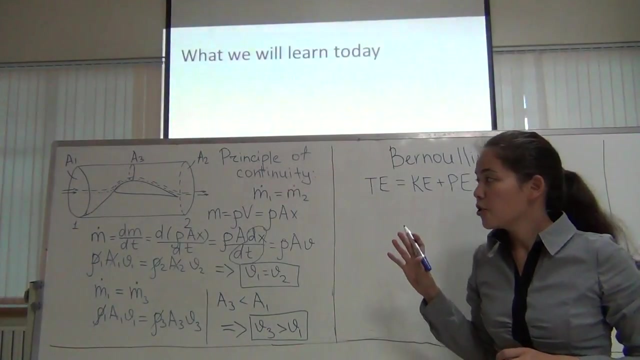 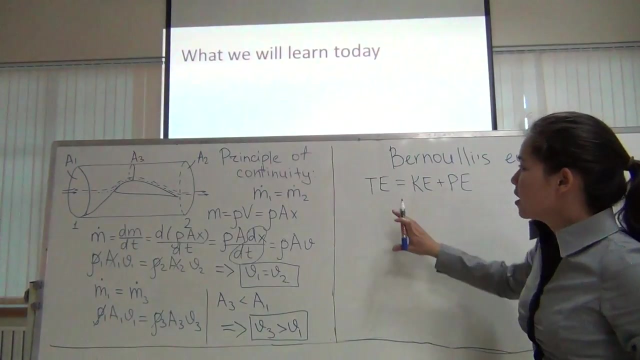 Kinetic Energy Plus Potential Energy, But This Is For Large Objects And It's Mainly Used In Physics. But In Our Case We're In Our 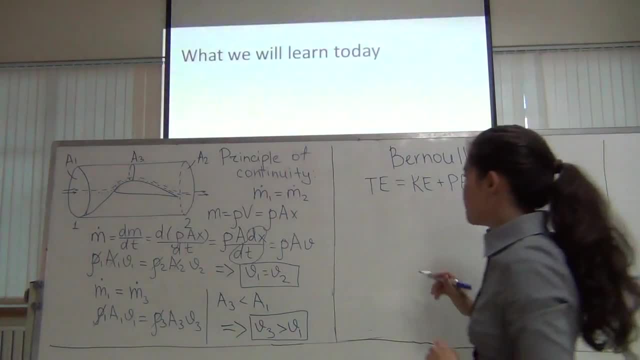 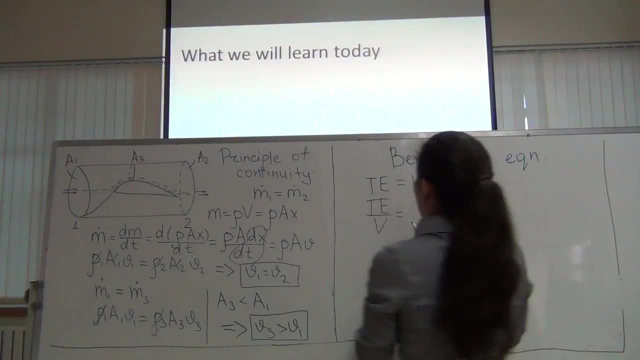 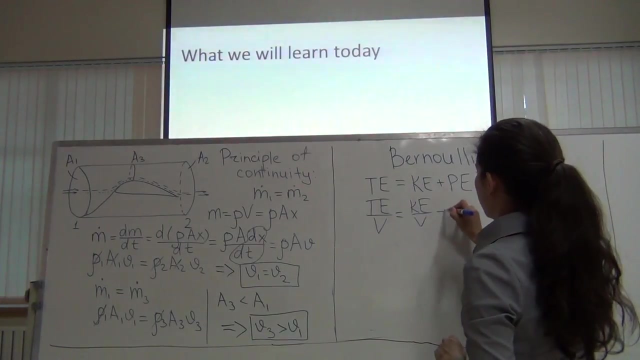 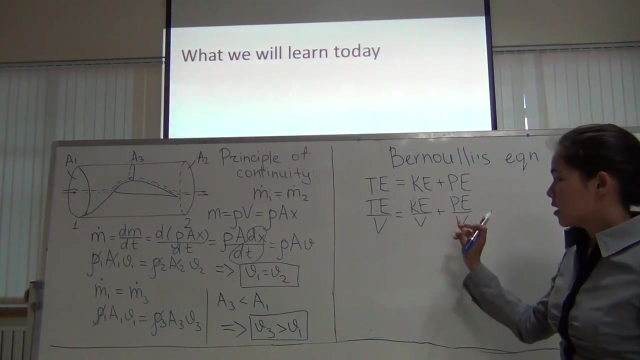 Study. So Let's Find Out What The Energy Is Per Unit Volume. So We Can Divide This Equation By Volume. So Total Energy Per Volume. 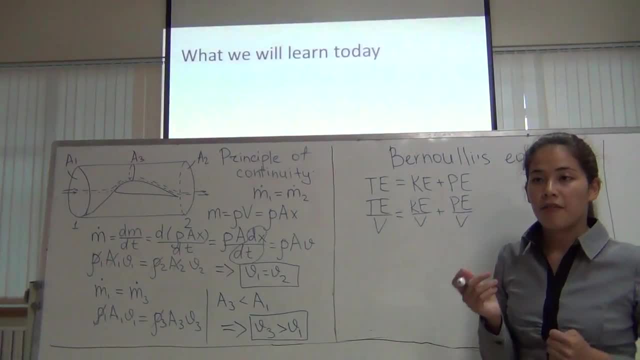 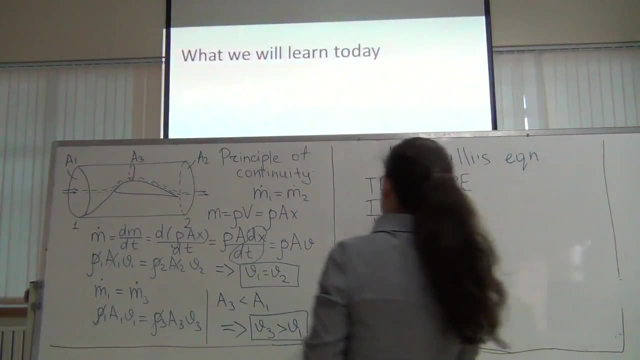 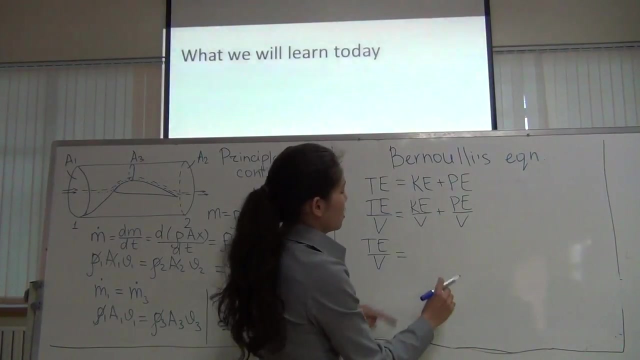 Is Equal To One Half Mass Multiplied By Velocity Square. Let's Substitute This Expression Into This Equation, So Total Energy Per Volume Is Equal To: 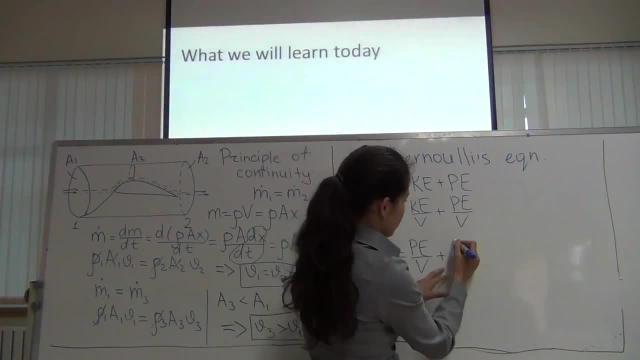 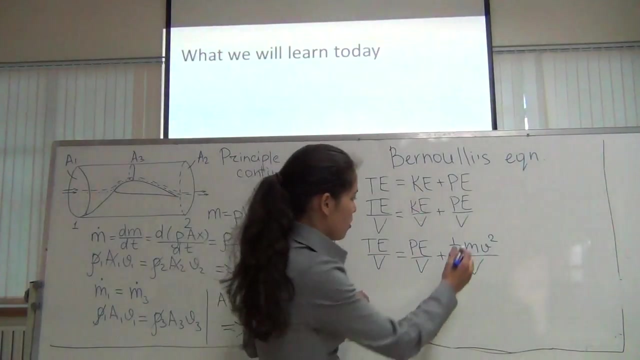 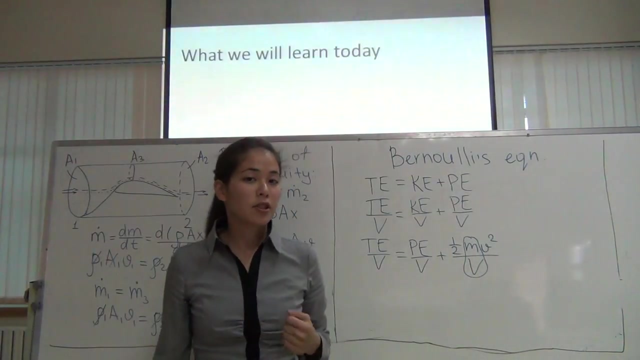 Let Me Put Potential Energy First Here. And We Can Divide By Velocity Square And Divide By Volume And We Can See Here, We Know This. 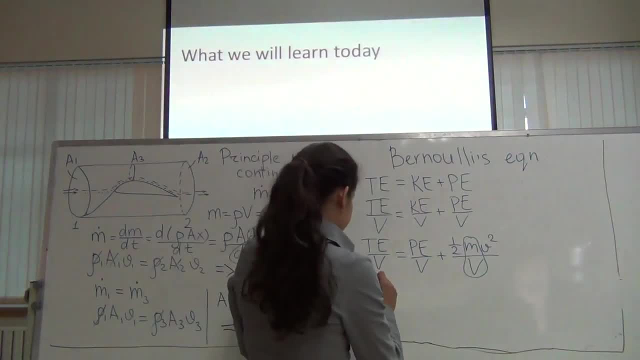 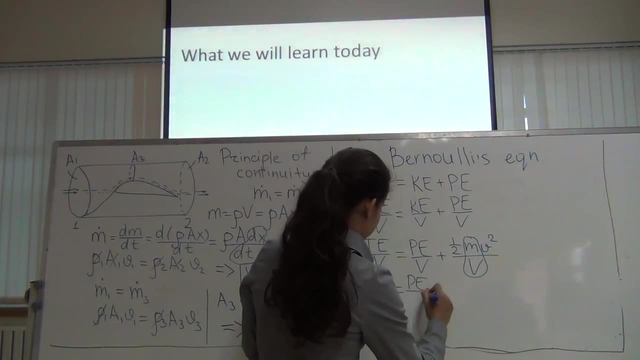 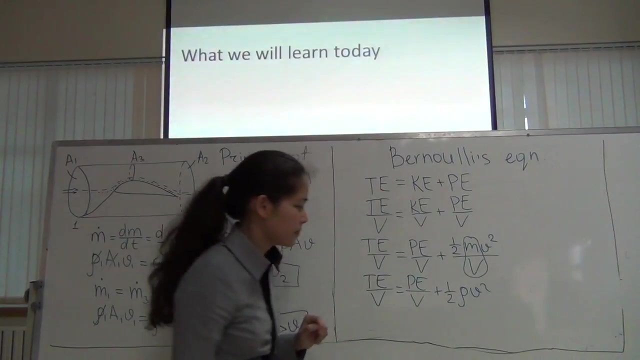 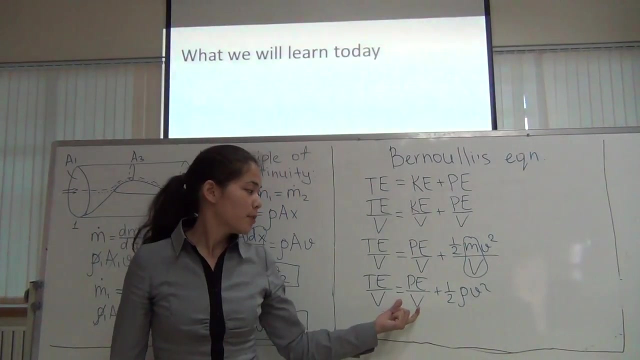 Quantity, Mass Of Substance Per Unit Volume It Is Equal To Potential Energy Per Volume. Let's Think About It For A Bit Of Potential Energy. 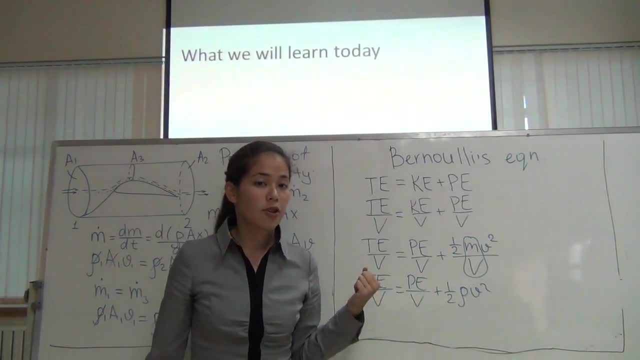 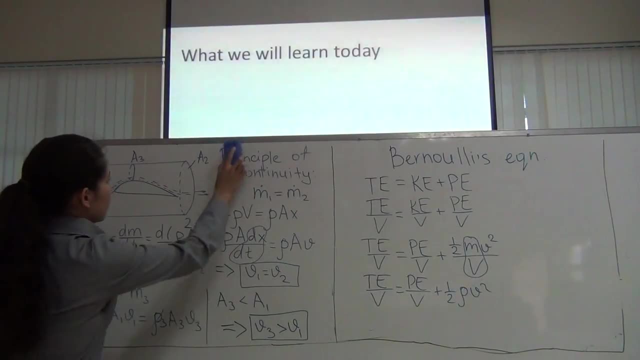 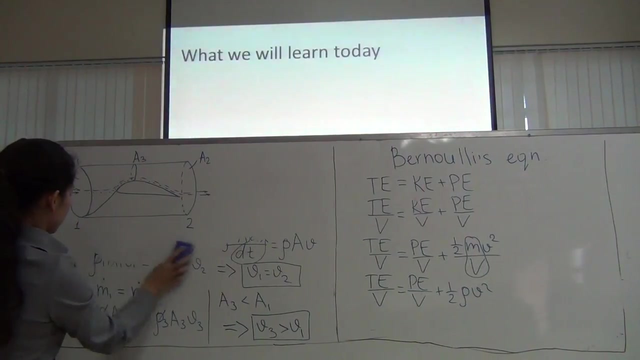 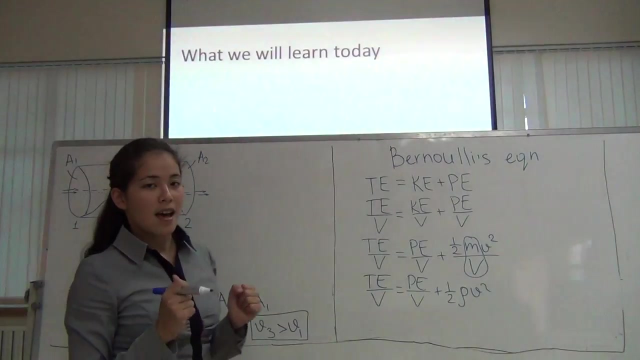 Per Volume- Let's Think About It For Bit- Can Erase Here. We Have A Volume Of Gas In The Cube And This Gas Has Some. 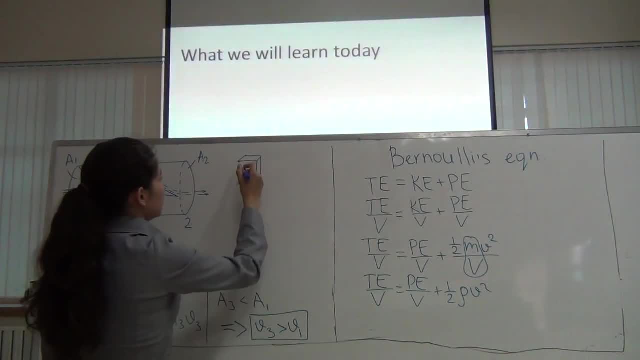 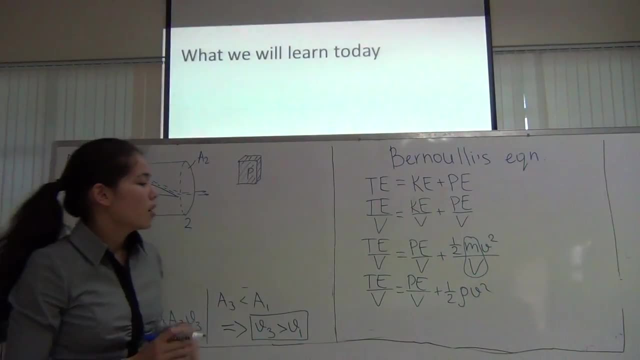 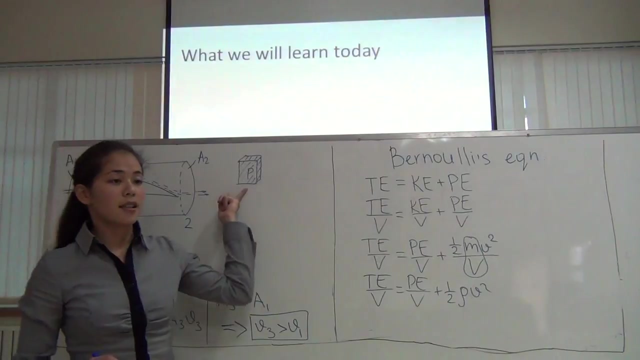 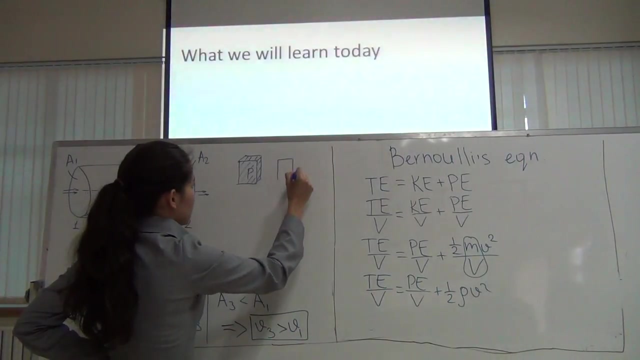 Pressure Inside. Now Potential Energy Is The Ability To Do Work. So What Kind Of Work Can Gas In The Box Do? Let's Think About. 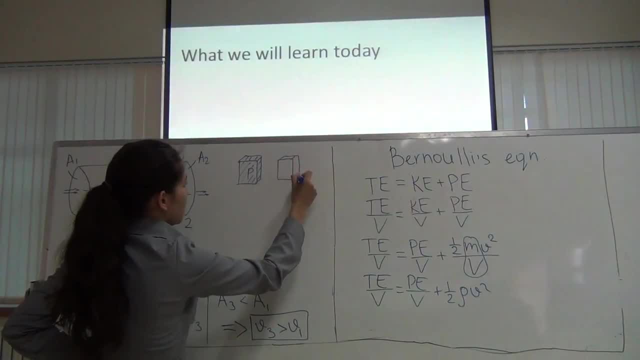 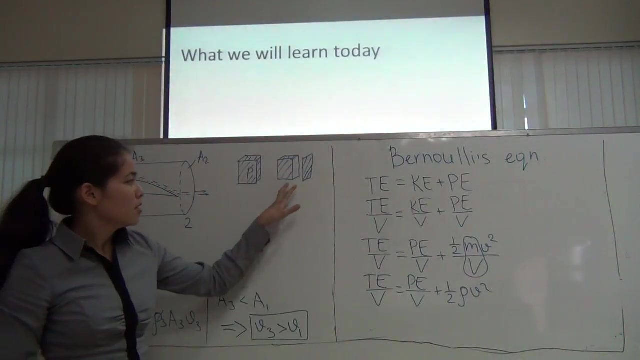 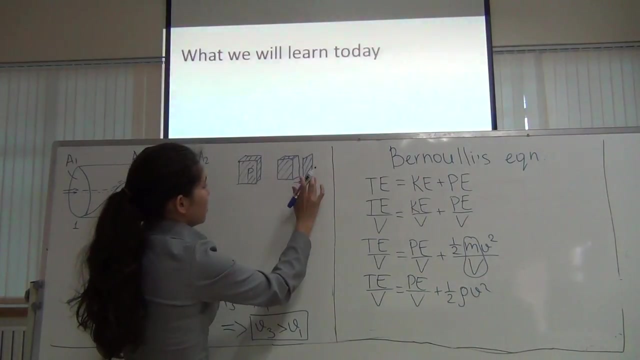 It. So If We Open Up The Box Open One Side Of The Box. So Here It's Still The Same, But The Gas Inside Will. 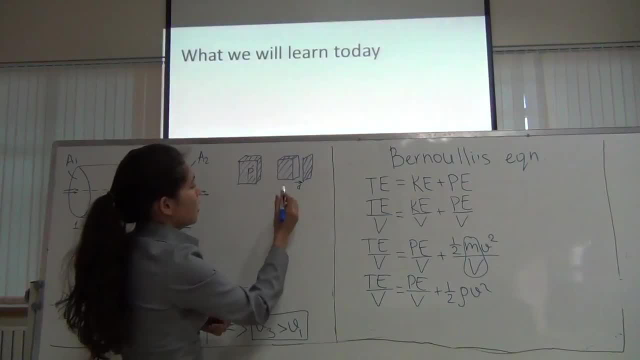 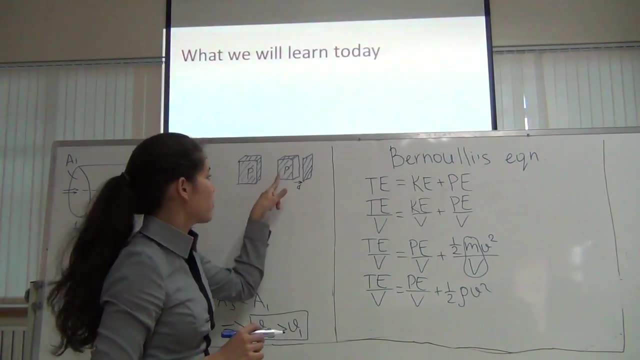 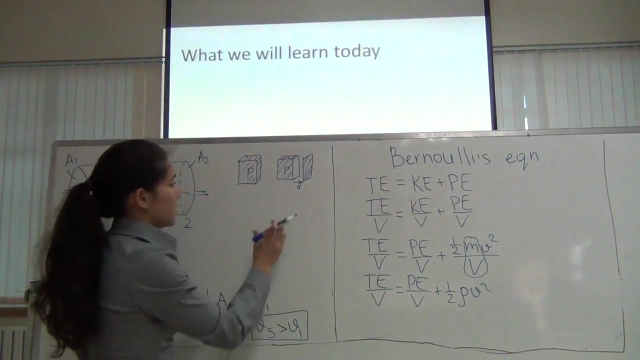 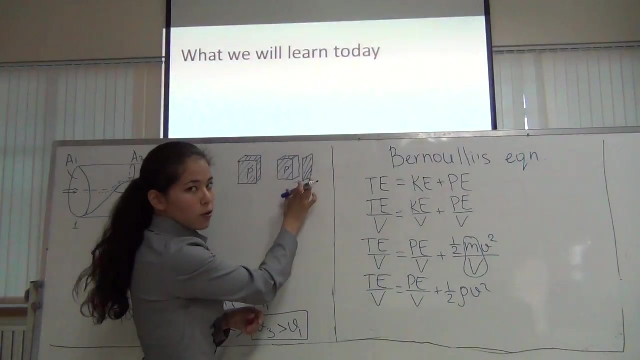 Move This Side Of The Box For Some Distance Because Of The Pressure That Was Inside, And It Will Move This Side Until The Pressure Is. 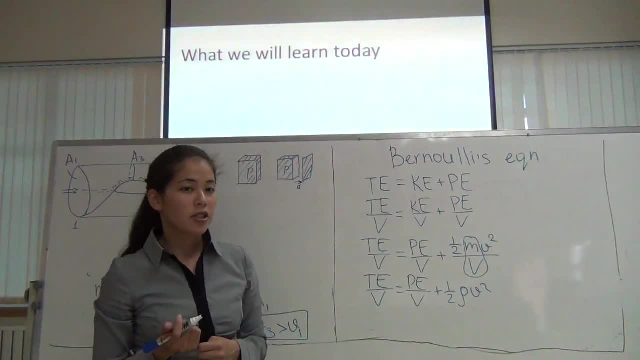 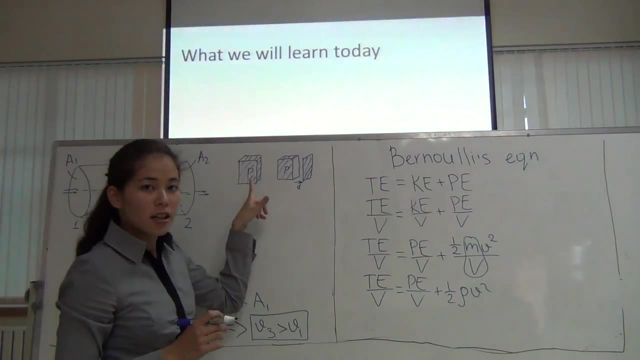 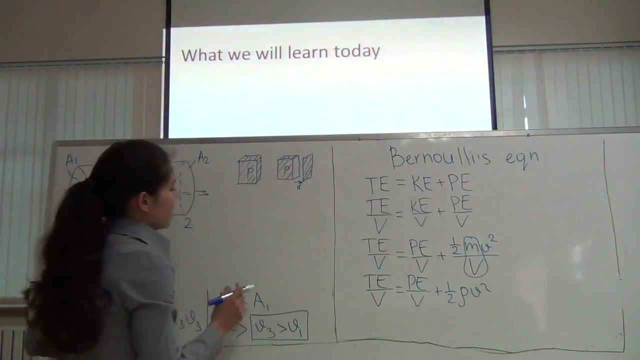 Distance. So That Means That Pressure Is A Potential Energy Per Volume Of A Gas. But Since The Gas Is Inside And It's Static, We 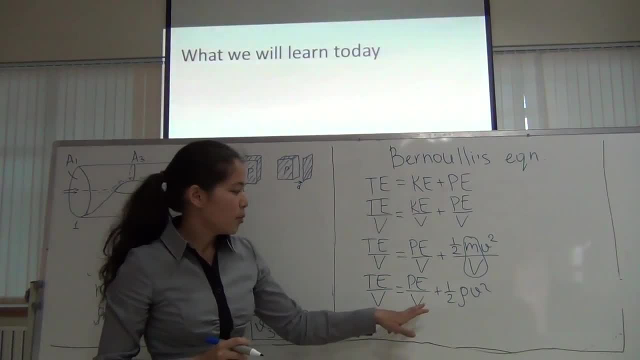 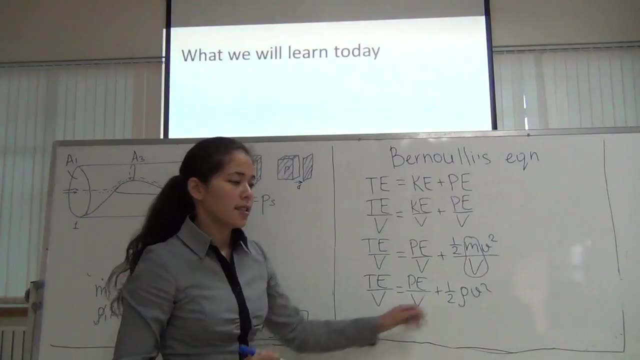 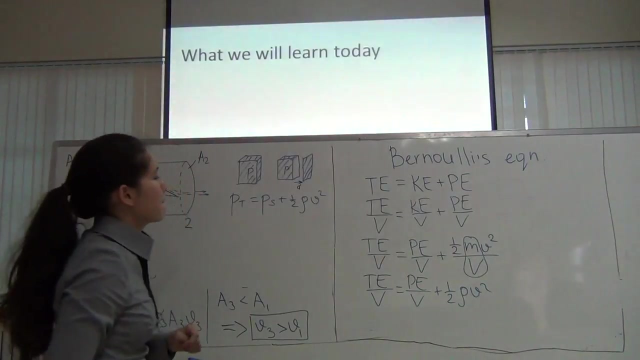 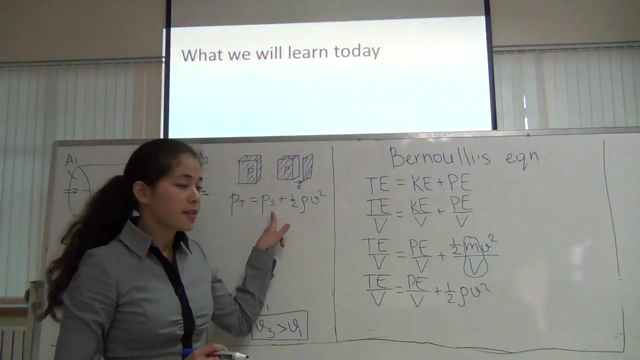 Call It Static Pressure. So It Will Be Static Pressure, And We Add The Quantity, That Is One Half Rho V Square. Okay, Now So. 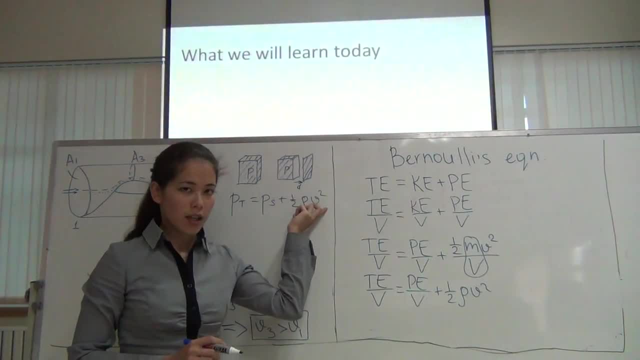 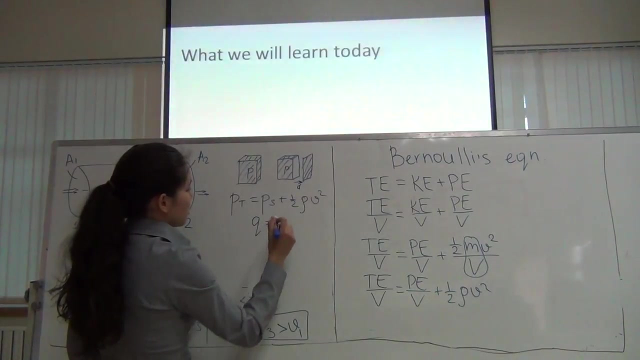 If This Is, This Is Total Pressure And This Is Static. We Will Call It Dynamic Pressure Because It's Moving And We Denote It As. 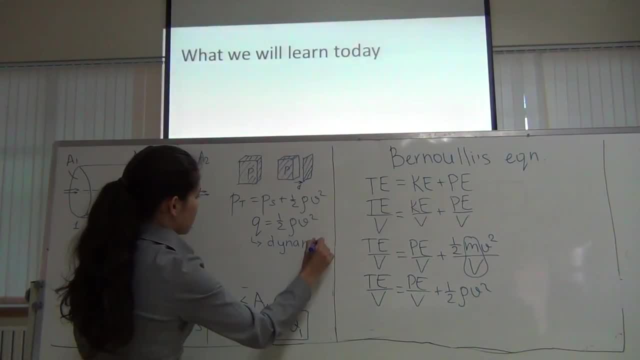 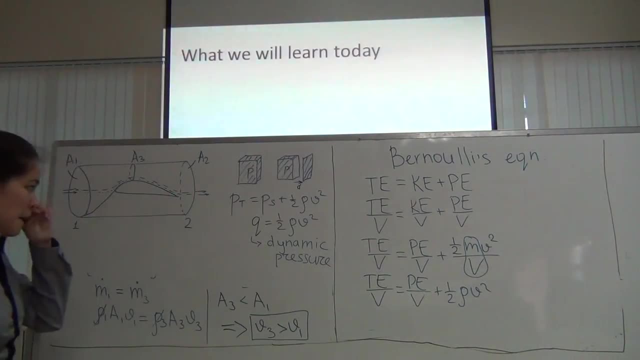 Q. Q Equals One Half Rho V Square, And This Is Dynamic Pressure, All Right Pressure. So Total Pressure Will Equal To Static Pressure Plus. 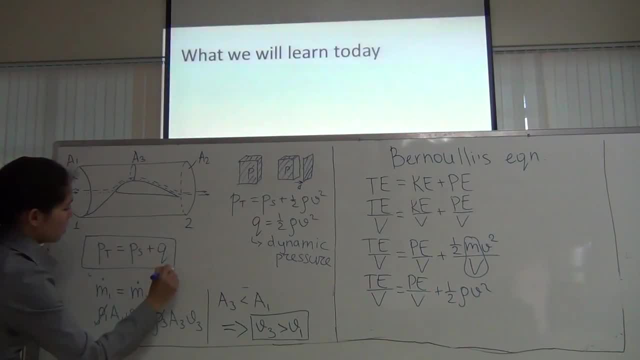 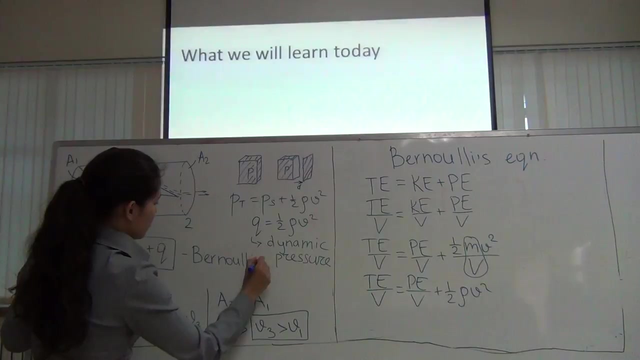 Dynamic Pressure, And This Equation Is Called Bernoulli's Equation, And Using This Equation, We Will Learn Why The Wing Is All Right. Now Let's. 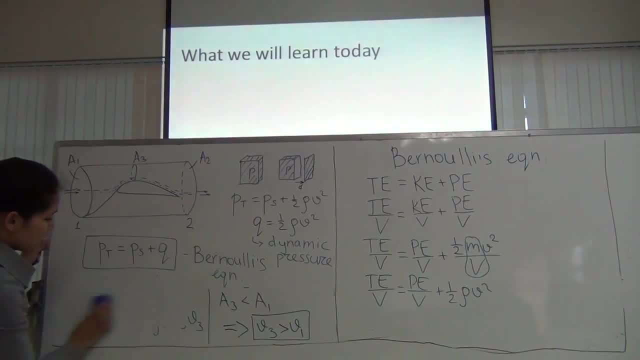 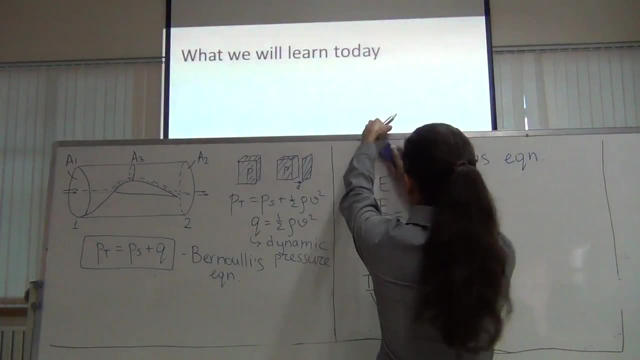 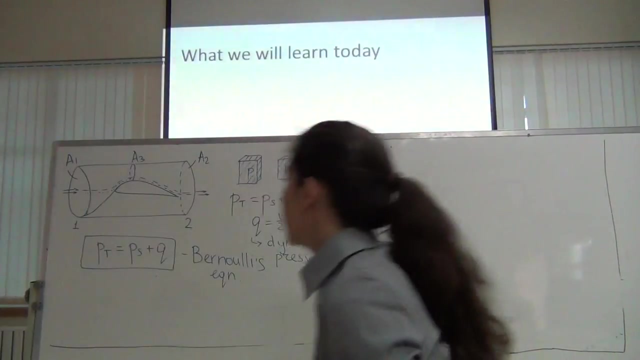 Apply This Equation To Our Wind Tunnel. Let Me Erase In Here, So For Inlet One. If We Apply Bernoulli's Equation, We Will. 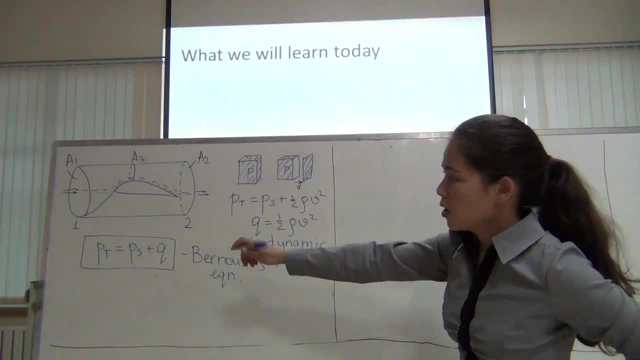 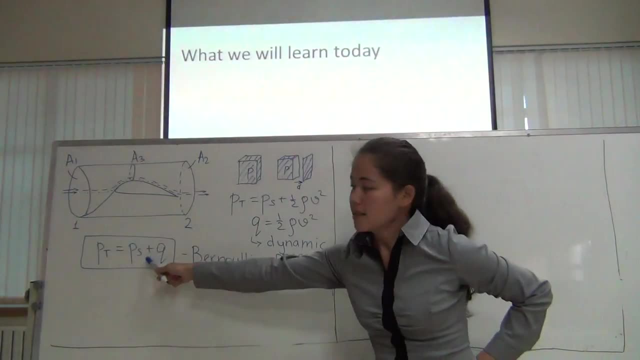 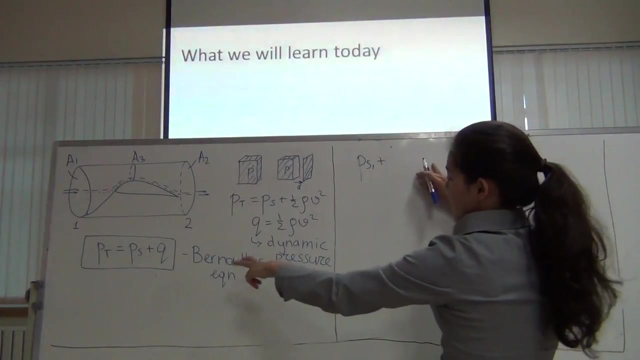 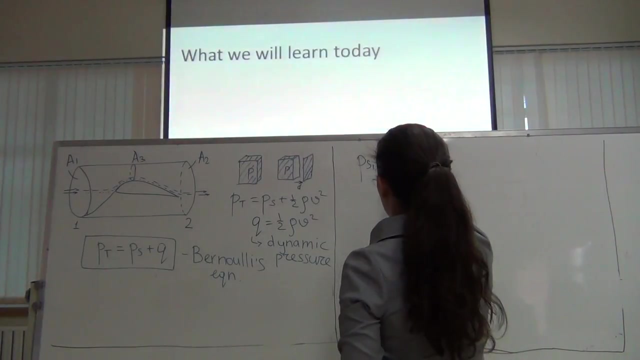 Get Total. Total Pressure Should Be Equal Everywhere Inside The Wind Tunnel. But For Inlet One We Will Get P Static One Static Pressure At. 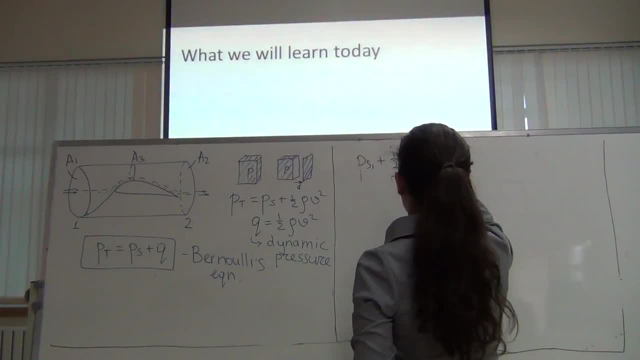 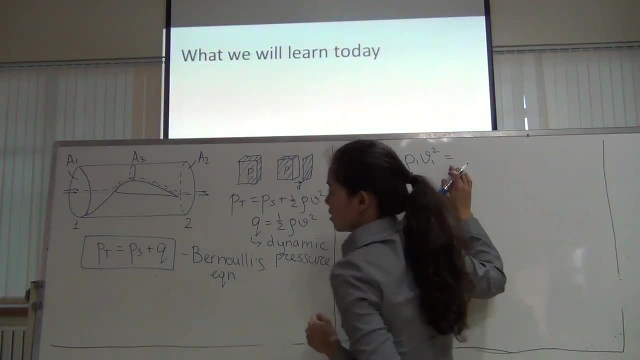 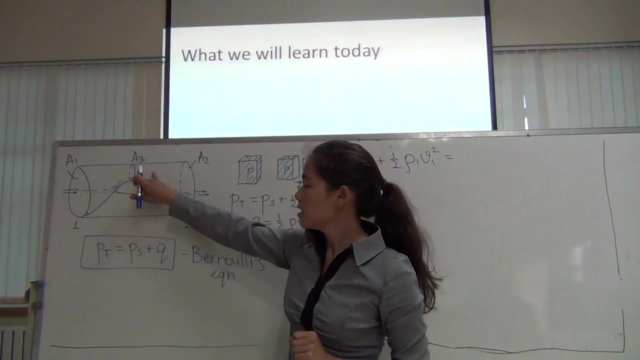 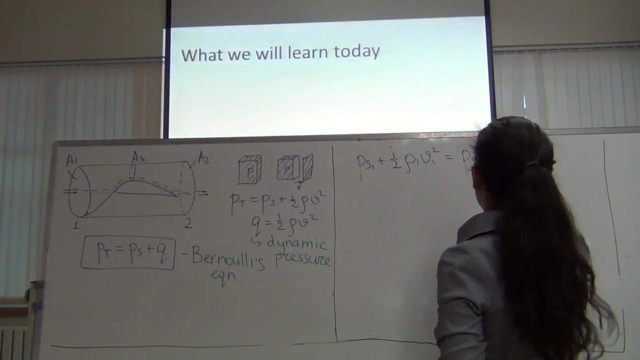 Inlet One Plus Dynamic Pressure At Wind Tunnel And This Will Be Equal To Total. Pressure Is Still Equal Inside The Wind Tunnel And This 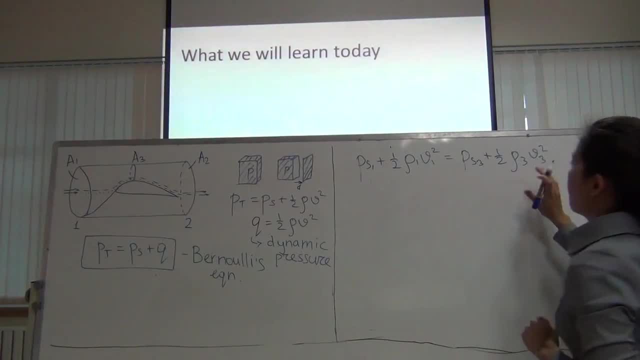 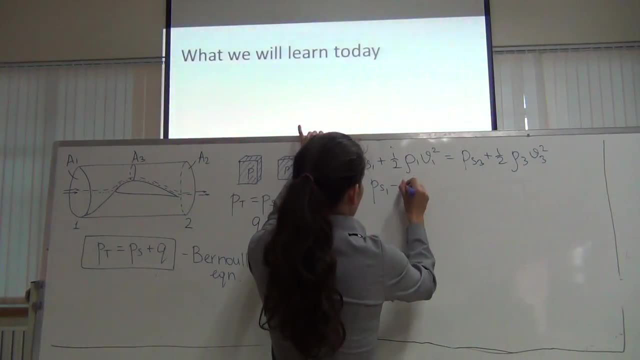 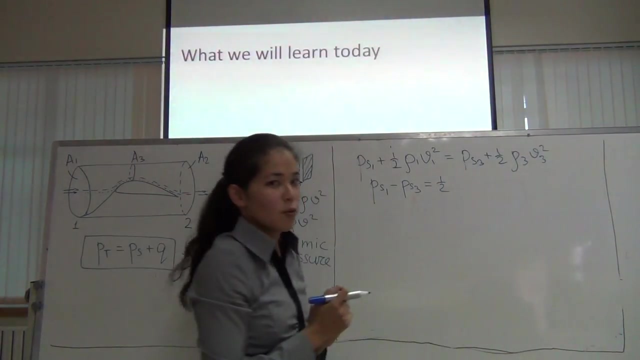 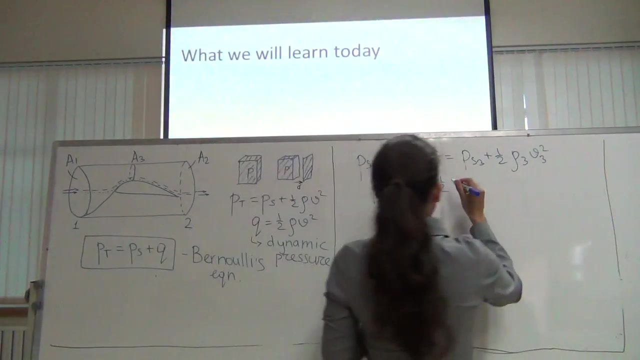 Will. If We Consider Area Three, We Will Have That P Static One Minus P Static Three, Equal To One Half, And We Assume That. 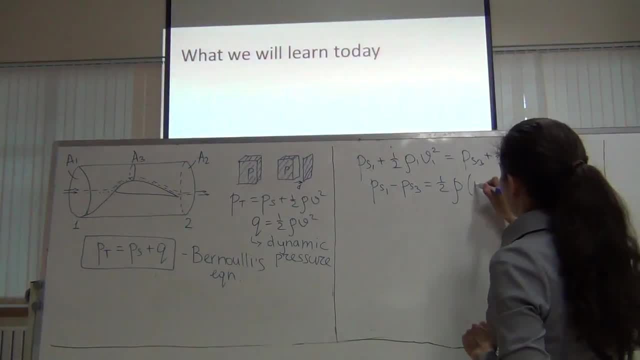 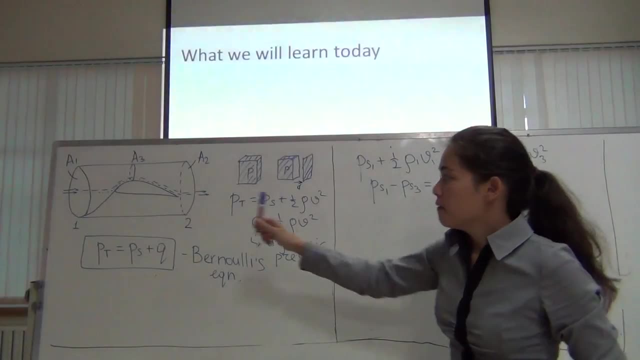 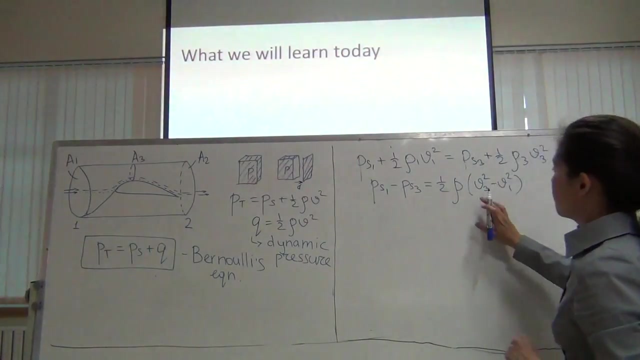 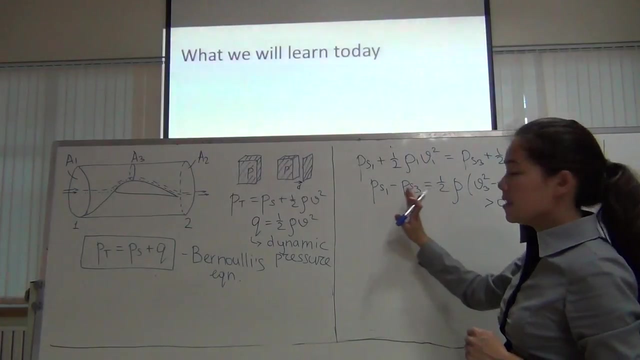 This Is Incompressible Flow, Which Means The Density Is Constant, So We Can Assume What We Found Out Before. So That Means, If We Subtract, 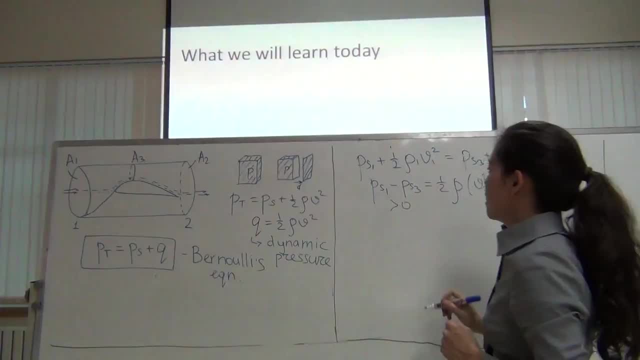 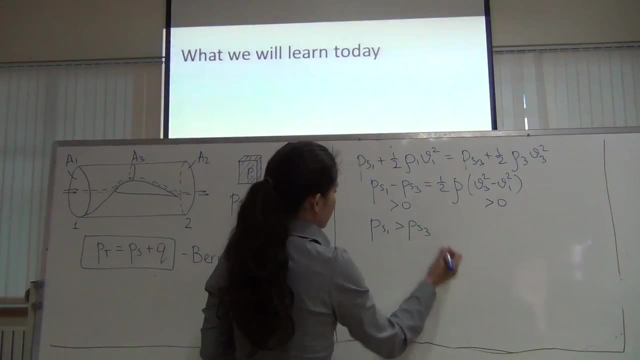 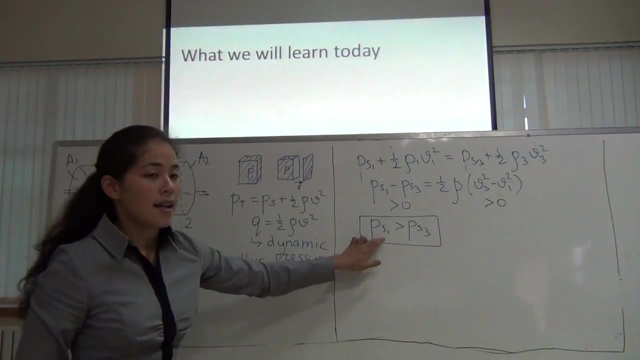 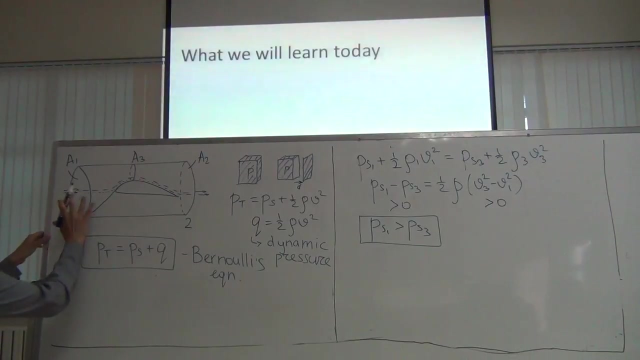 B1. From B3. It Should Be Greater Than Zero, But That Will Mean That This Side Of The One Is Pressure Here, But Also If 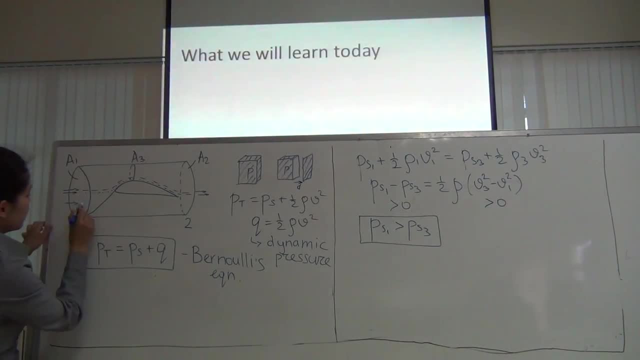 We Have, If We Had A Wind Tunnel Straight, Whatever Pressure The Air Enters Here Will Be The Same, While It's Moving Through Like Three. 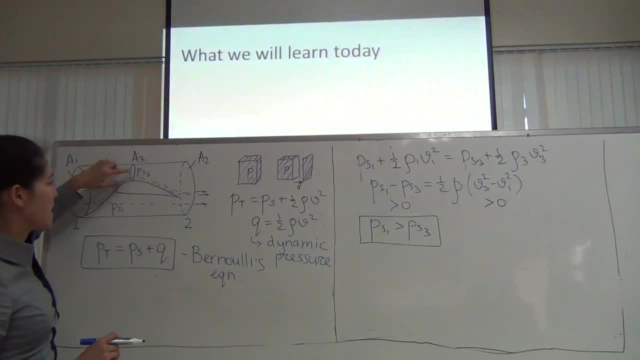 What Will Happen To Our Air Foil? It Will Tend To Move To The Area That Is Less Pressure, So It Will Tend To. 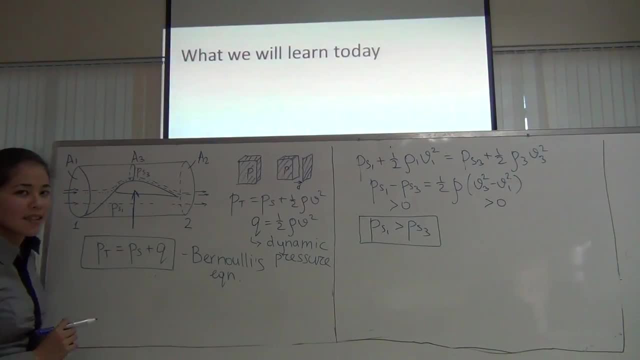 Move Where It Will Tend To The Air Force. So This Is Our Famous Lift Force. It Is Denoted As L, And This Is Why. 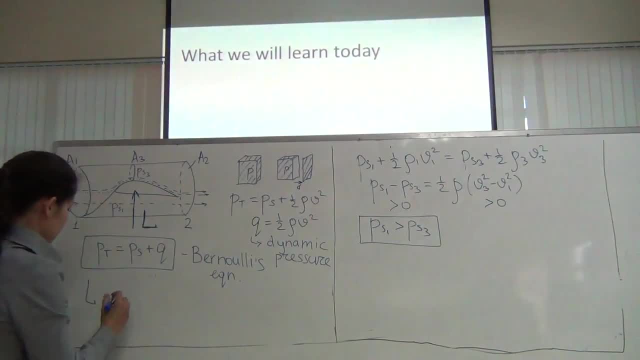 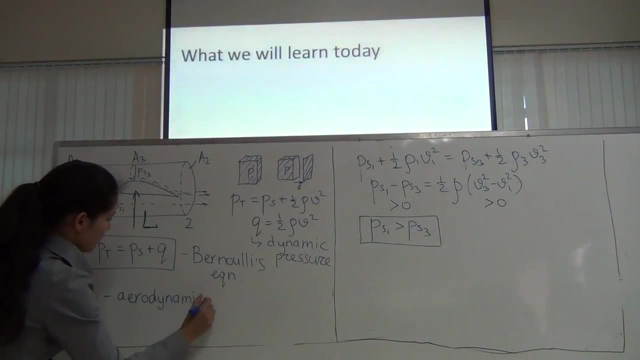 Airfoil And Wing And Aircraft Is Able To Move To The Area. It Will Tend To. The Area Is Less Pressure, It Will Tend. 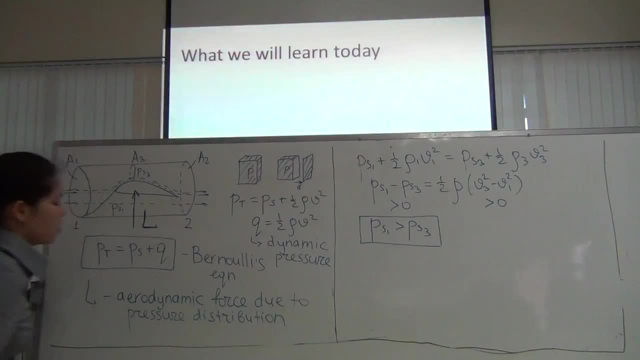 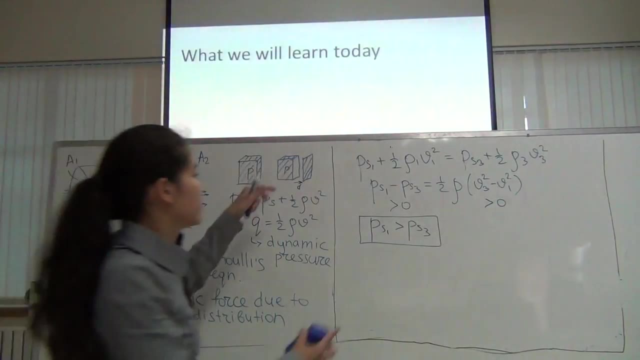 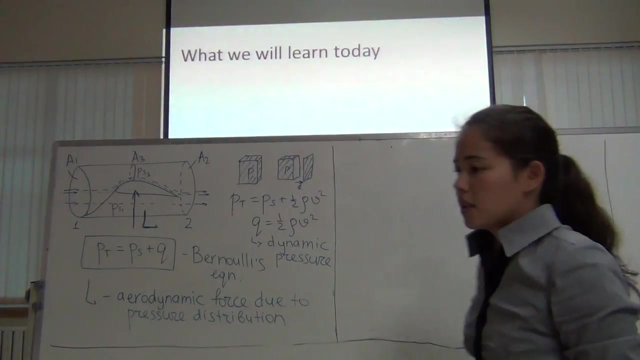 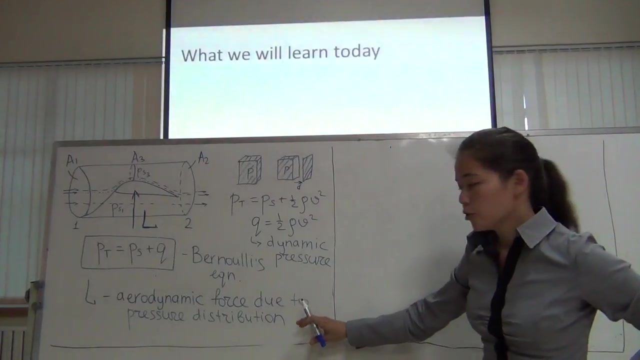 To Air Force Due To Pressure Distribution. All Right. Now It Is Time There Is Also Drag That Results From Pressure Distribution, But It's A Lot Smaller For The For Good Design, Well Designed Airfoil Drag Should Be A Lot Smaller Than Lift Upwards. We Found Out That It. 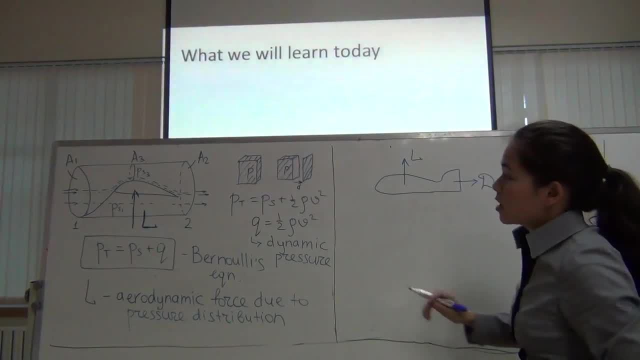 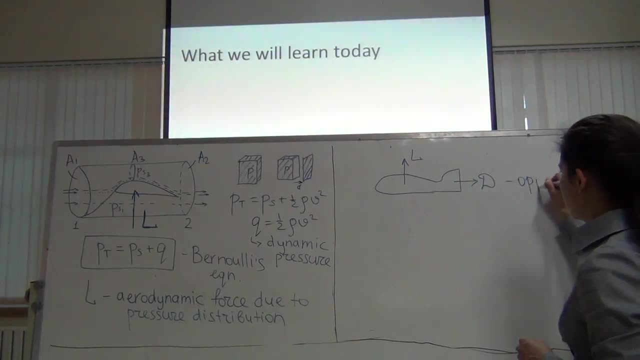 Has. Lift Upwards And Then Drag Is A Force That Occurs For The Same Reasons As Lift, But It Should Be Less, And It Is. 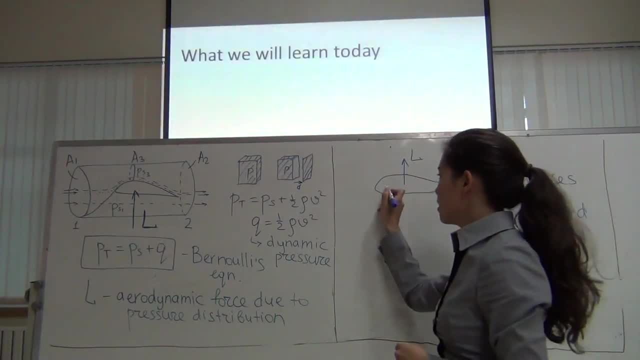 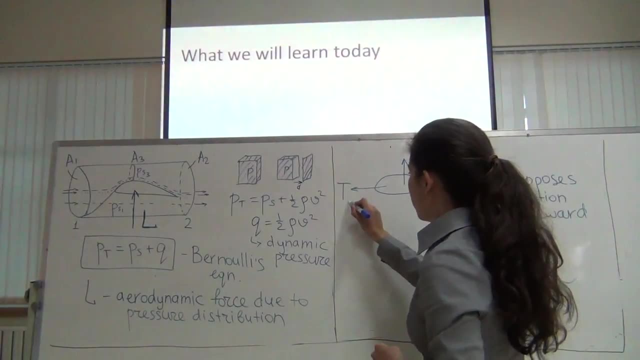 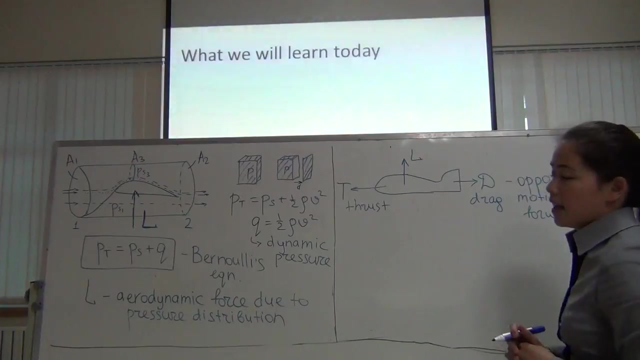 A Lot. But What Enables The Aircraft Fly Is Thrust That Occurs From The Engines. Thrust Is Denoted As T, So This Is Thrust. 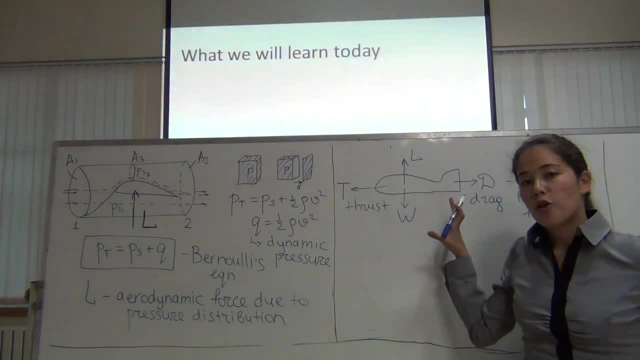 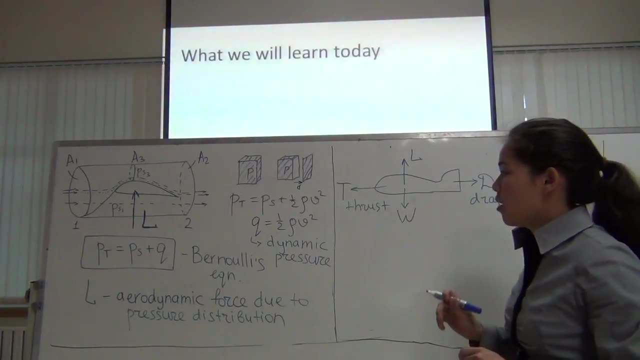 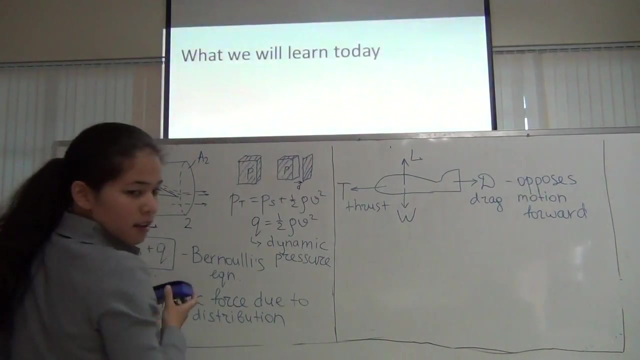 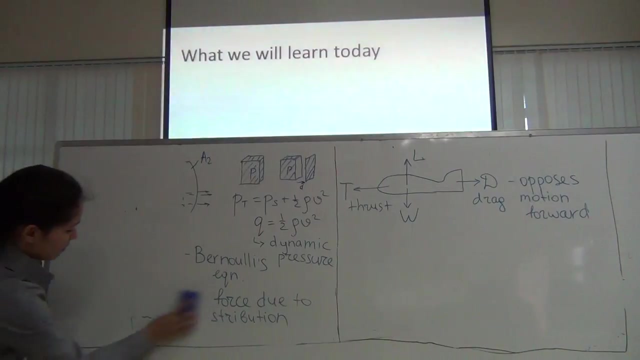 And This Is Drag Forces, Main Forces That Act On The Aircraft During Flight. All Right, Now Let's Proceed On To How Lift Is Calculated. 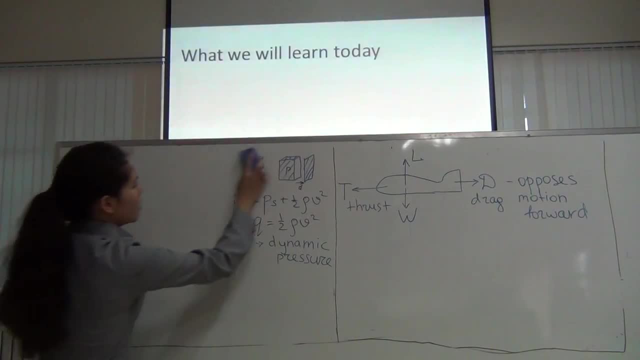 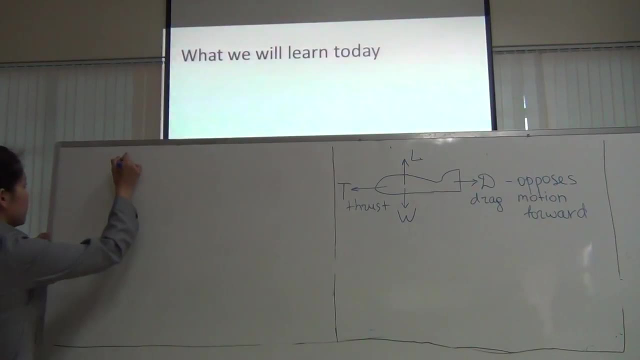 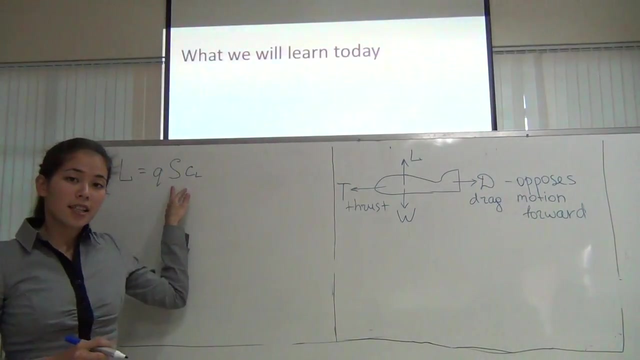 Okay, We Can Get Rid Of This Metal Hope. So Lift Is Equal To Dynamic Pressure Multiplied By The Plan Form Area Multiplied By C. 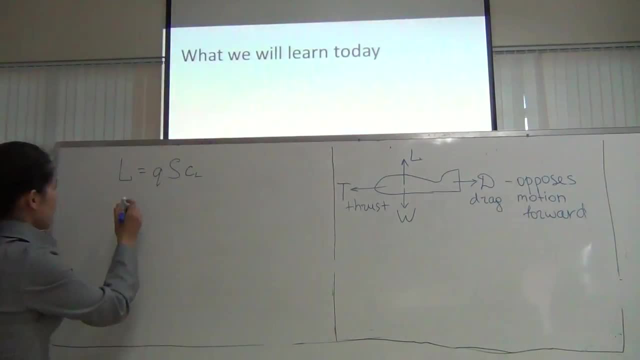 L. This Formula Was Determined Theoretically But Also Proven Experimental Many Times And To Dynamic Pressure Multiplied By Plan Form Area, It's Almost. 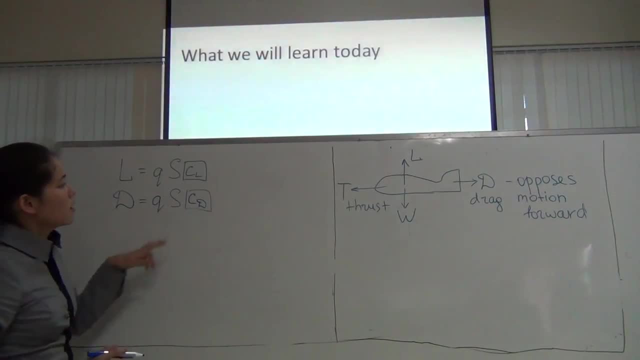 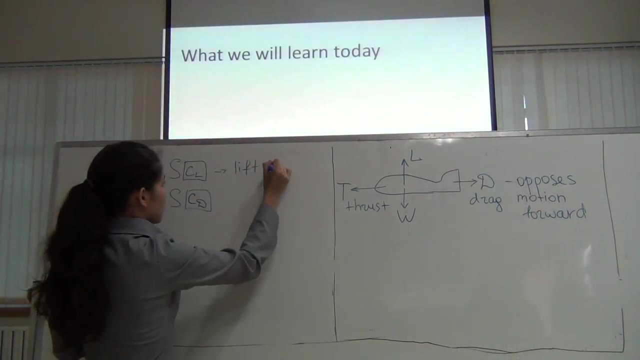 The Same, But The Coefficient Is C D. So What Are These Coefficient? C? L Is Called Lift Coefficient And C? D Is The. 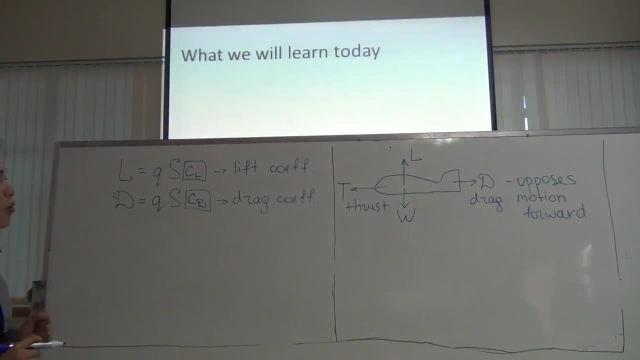 Coefficient Now. So Imagine If We Had Two Airplanes: One Very Small That Fits Into Wind Tunnel, And The Other One Is Air Bus A380.. 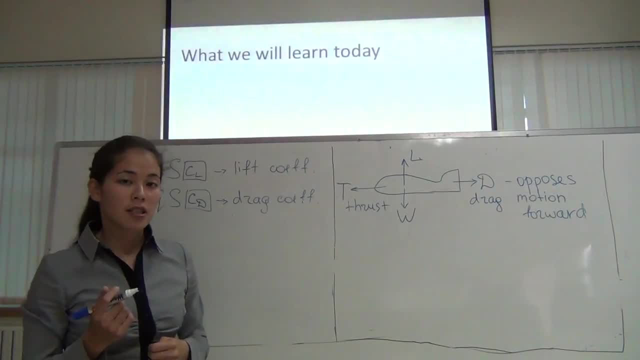 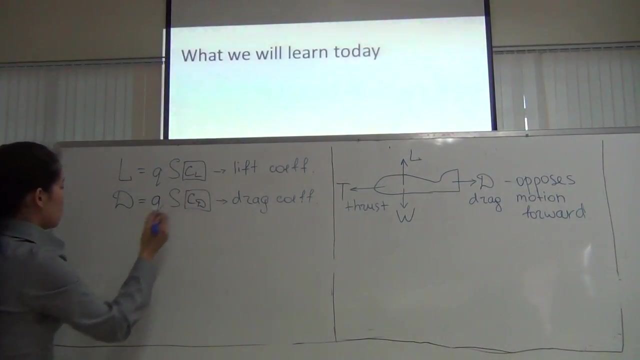 If We, It Is Dimensionless, And These Two Coefficient Enable Us To Understand How How Good The Air Flow Performs. So These Are Called Performance. 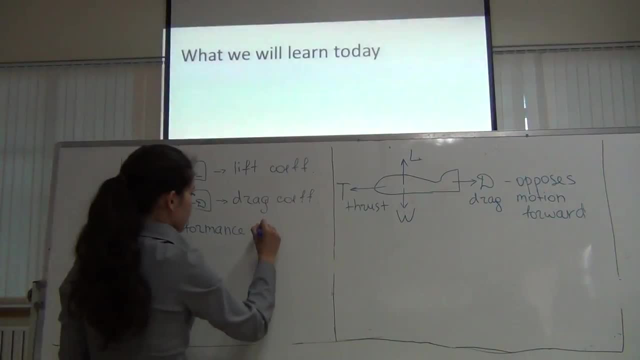 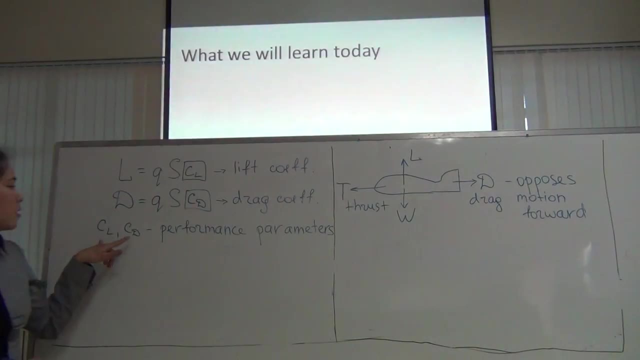 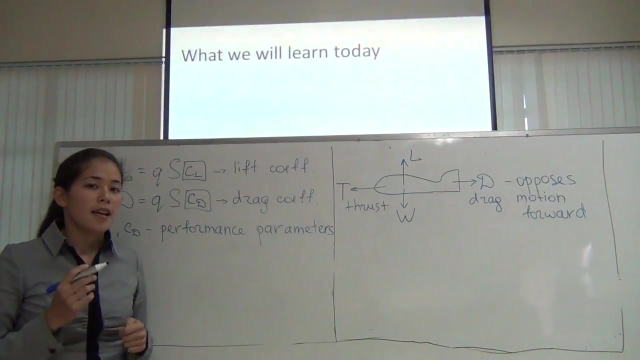 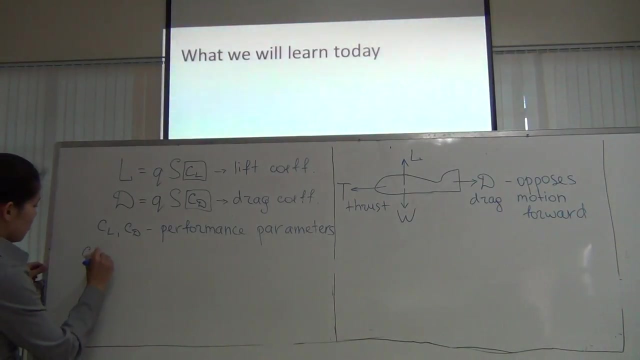 Parameters And It Was Determined That C, L And C Lift Coefficient And Drag Coefficient Depend On Angle Of Attack And Also On Two. 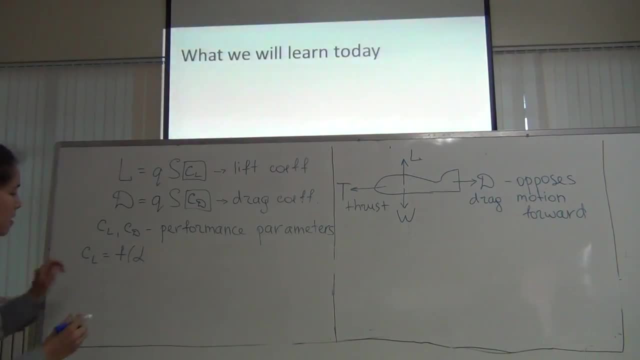 Other Dimensionless Numbers, Which Are Mach Number And Reynolds Number, And C? D Is The Same. It Depends On The Same Coefficient. But Let's 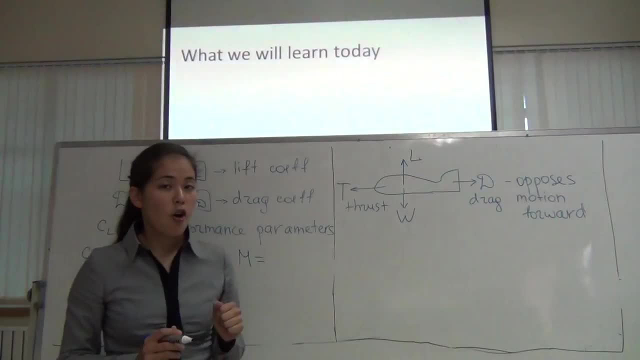 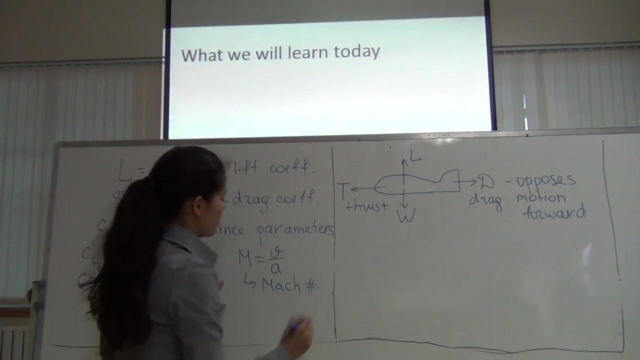 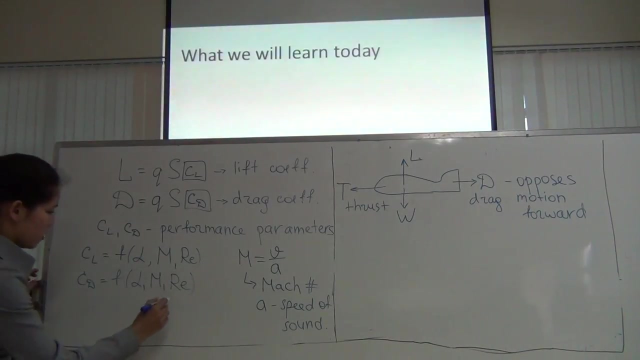 See What Mach Number Is The Ratio Of The Speed Of Sound. So This Is Mach Number And A Is Speed Of Sound. And What Is? 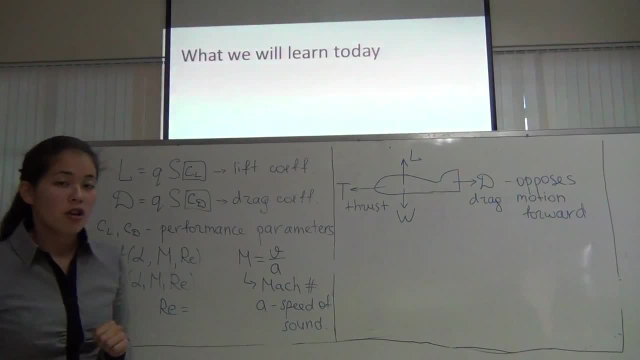 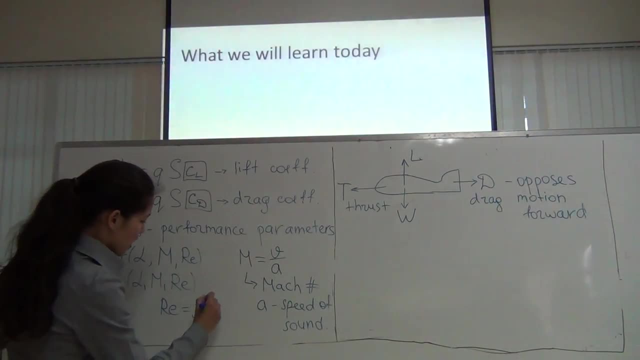 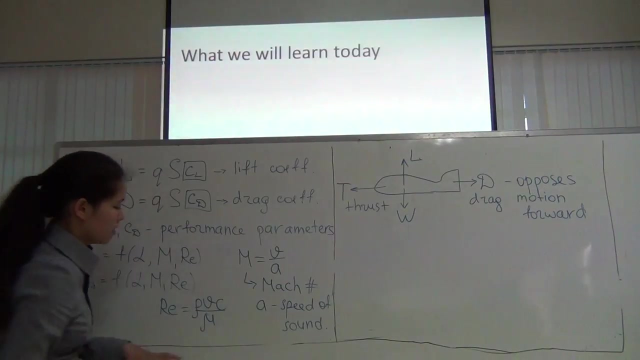 Reynolds Number. Reynolds Number Is A Measure, So Reynolds Number Is Defined As Density Multiplied By Velocity, Multiplied By Cord Over The Airfoil And. 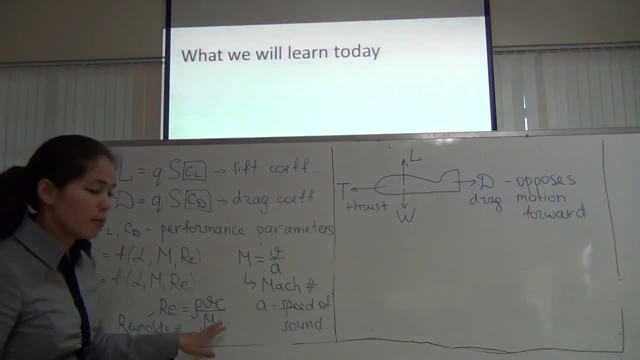 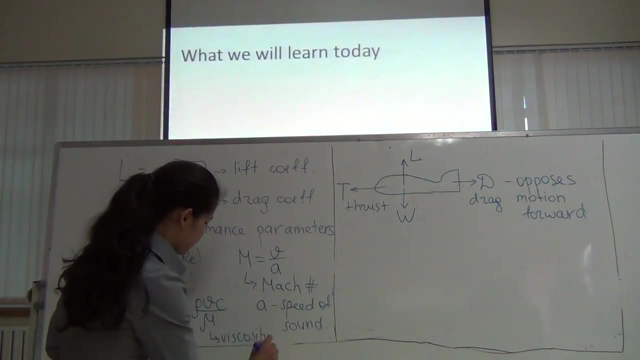 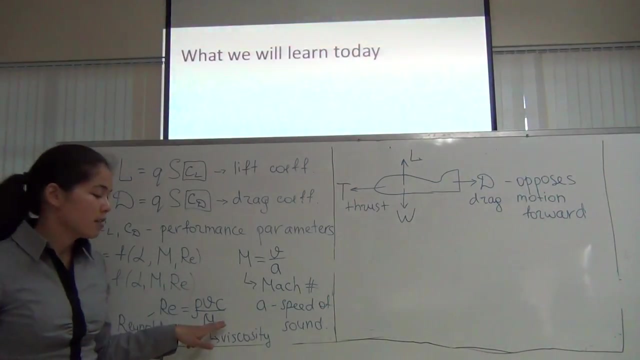 Divided By Viscosity. So This Is Called Reynolds Number And Mu Is High, So High, High Reynolds Number Mean That Viscosity Is Low. 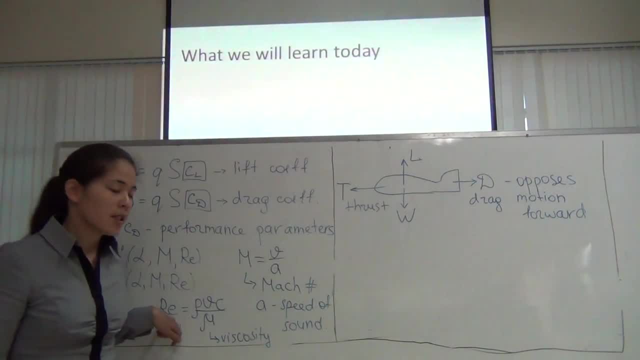 So We Can Assume That The Flow Is Invisible? This Is True For Low Velocity Flows And Low Speed And, Depending On Mach, Number Flows. 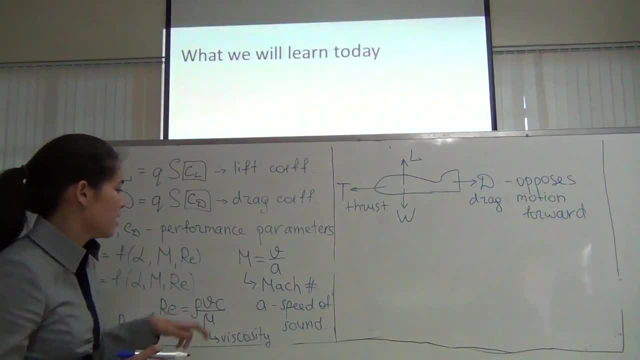 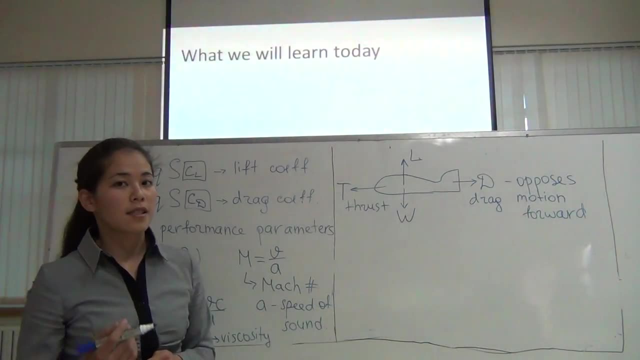 Can Be Supersonic, Subsonic Or Transonic. So If Mach Is Less Than One, This Will Be A Subsonic Flow, Which Means Flows. 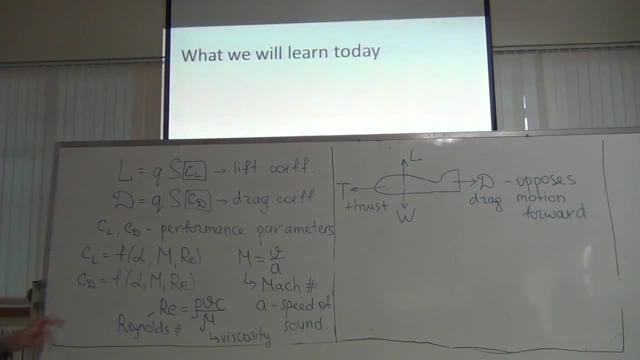 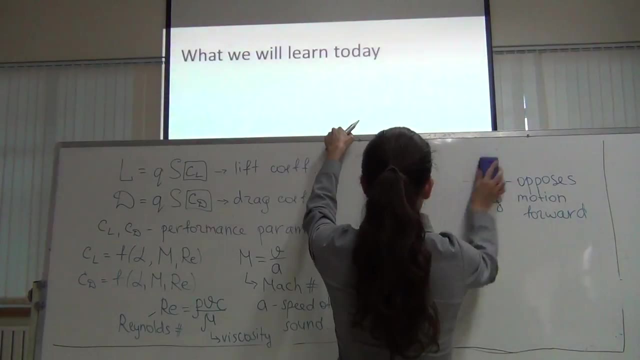 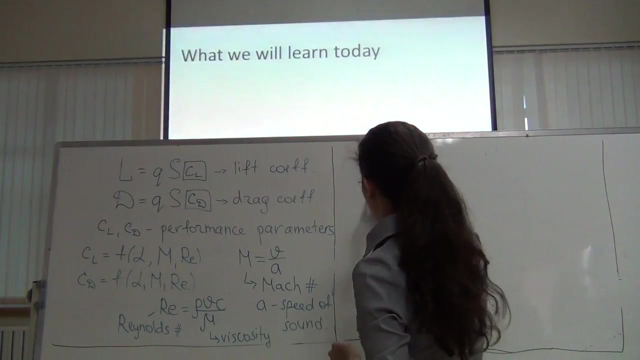 With These Numbers And Let's See How Lift Coefficient Depends On Angle Of Attack, It Was Determined That Lift Coefficient Varies With The: 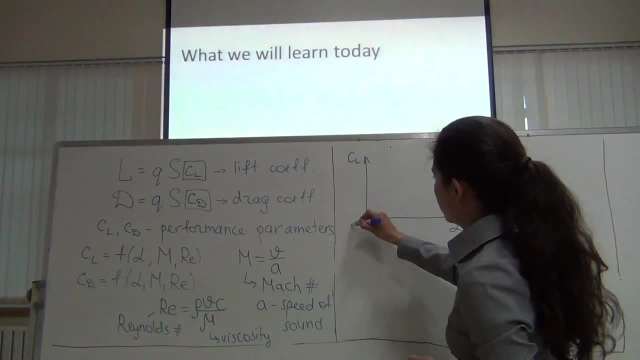 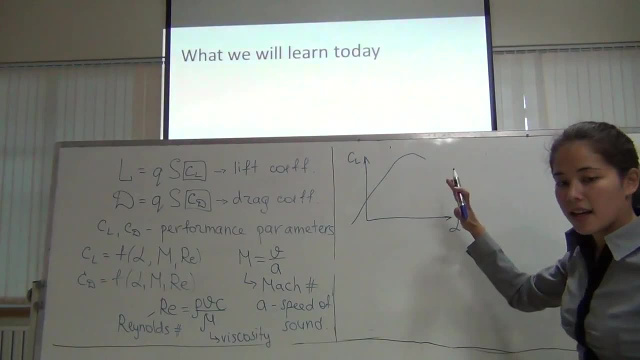 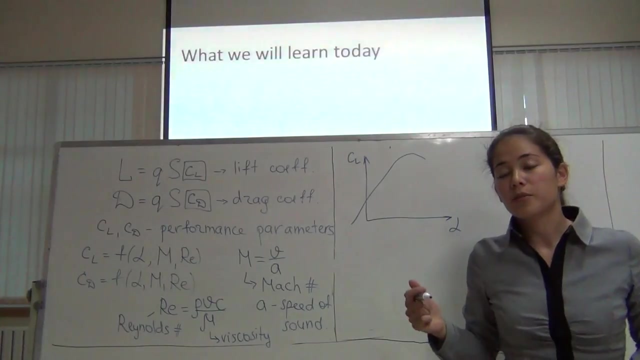 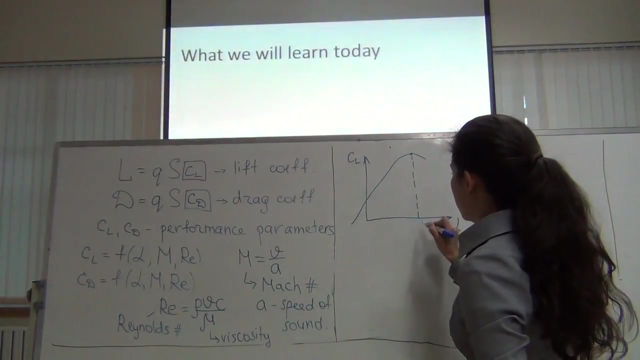 Angle Of Attack According To This Like This: So We See That As We Increase The Angle Of Attack, The Lift Coefficient Increases, So That 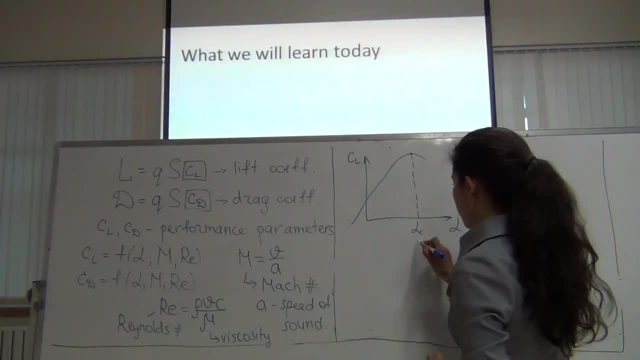 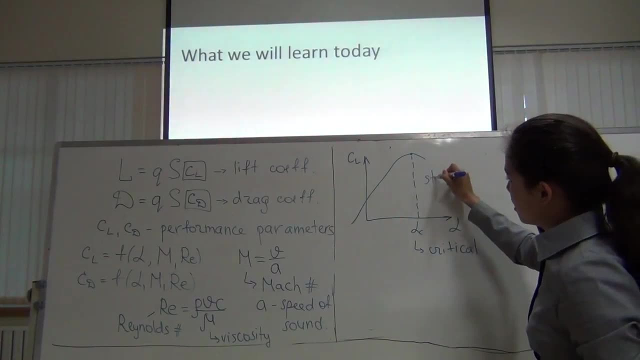 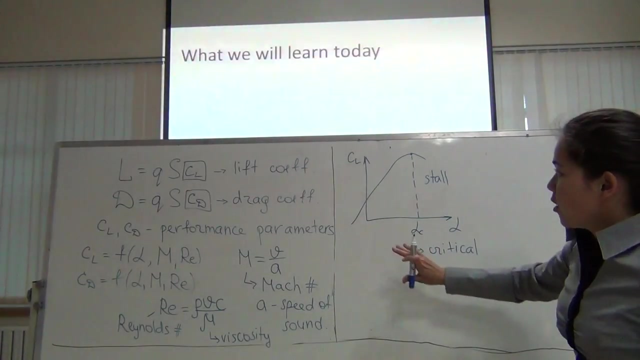 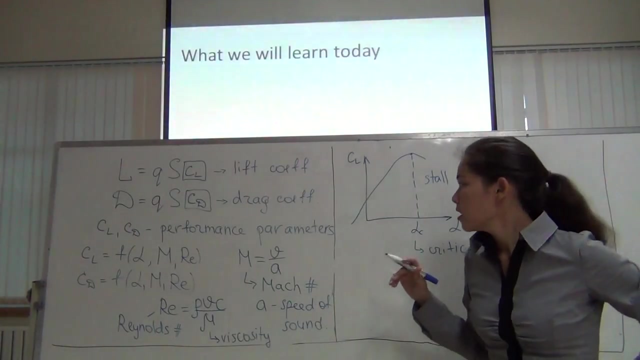 Means The Air Flow Will Produce More Lift, But There's At Some Less And Less Lift As You Increase The Angle Of Attack. So I 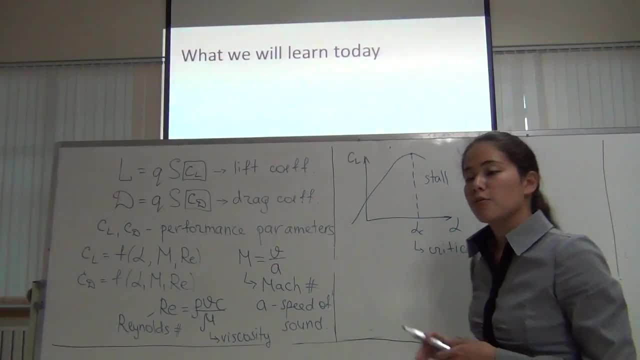 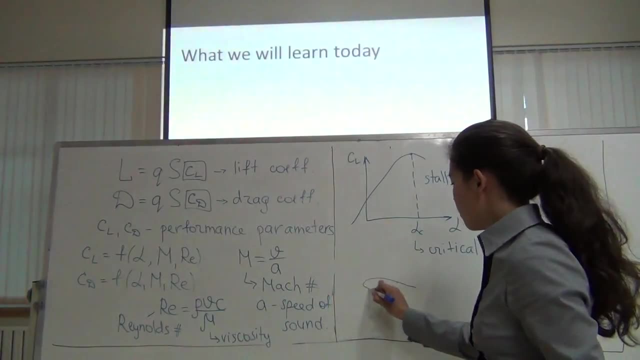 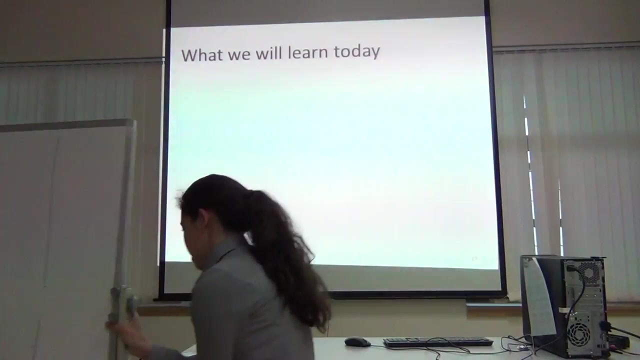 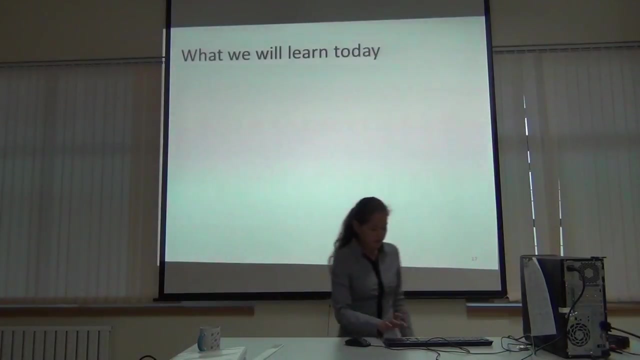 Think This Is Good For Today, But This We When We Talk About Air Falls, We Have Three Dimensions, So That Means The Physics Are A. 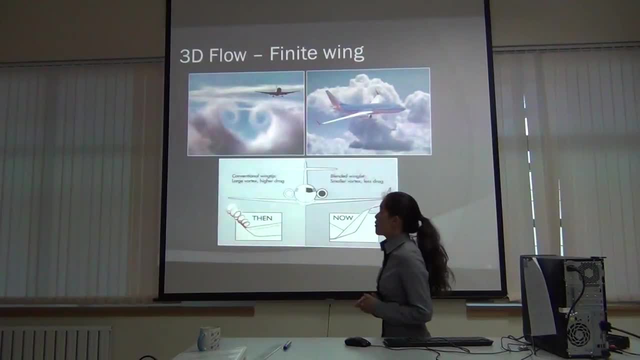 Little Bit Different And If We Consider A Finite Wing And 3D Flow, We Will See That An Effect Like A Flow On The Air